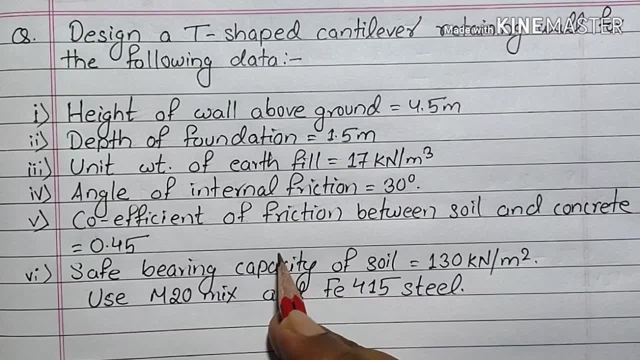 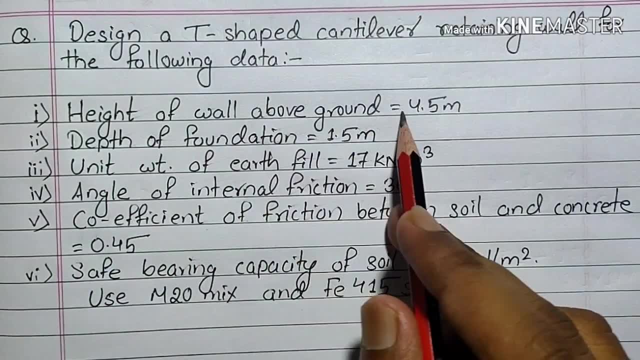 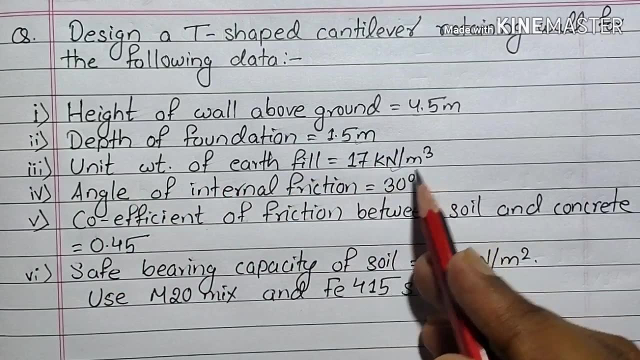 currently studying cantilever retaining wall. so, without wasting time, let's begin the video, and the given data is: the height of wall above the ground is 4.5 meter. depth of foundation is 1.5 meter. unit weight of earth fill is 17 kilo newton per cubic meter. angle of internal friction: 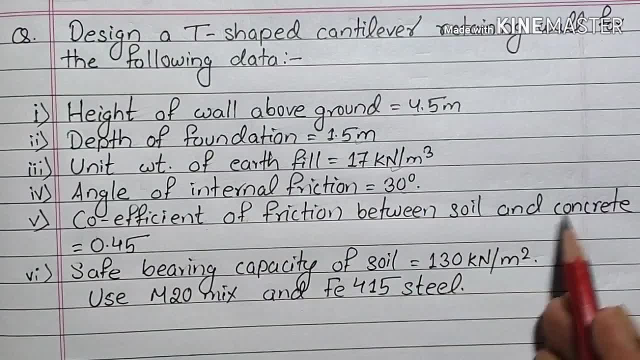 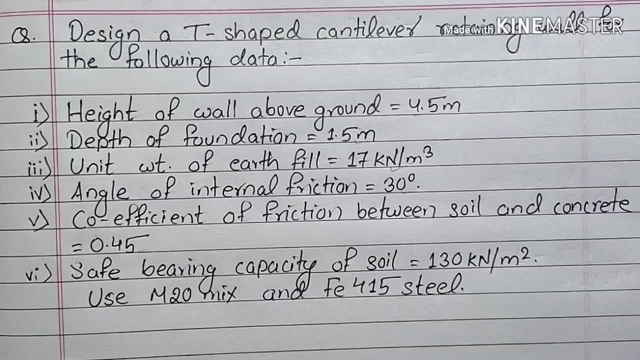 is 30 degree. coefficient of friction between soil and the concrete is 0.45. safe bearing capacity of soil is 130 kilo newton per meter square and the we are asked to use m20 mixed concrete and fe 400 rate 15 steel. so we will begin with a diagram or rough diagram of the retaining wall, from which 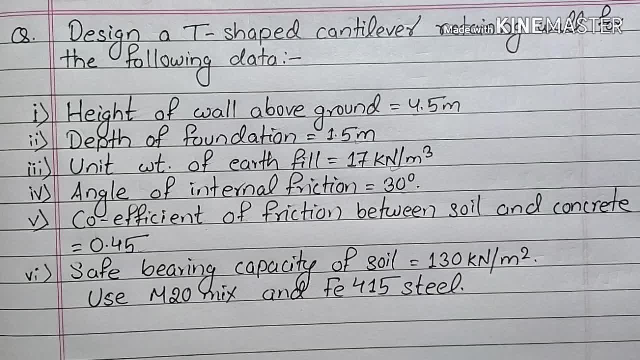 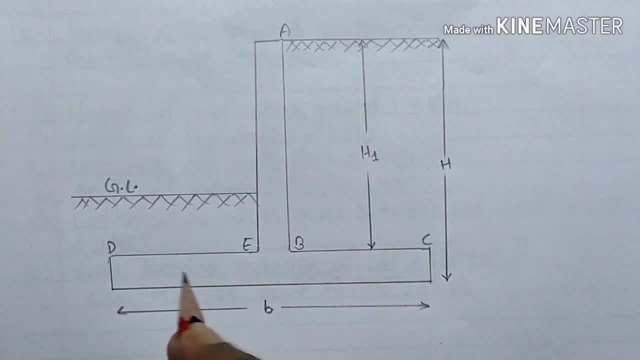 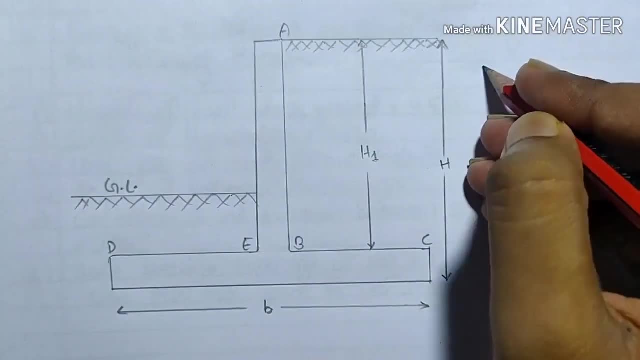 from which i will explain you about different parts of the retaining wall. so let's have a look at the diagram. and yes, here is the diagram of a t-shaped cantilever retaining wall. here the portion a, b is called the steam of cantilever retaining wall. let me write it down here: a, b is steam. 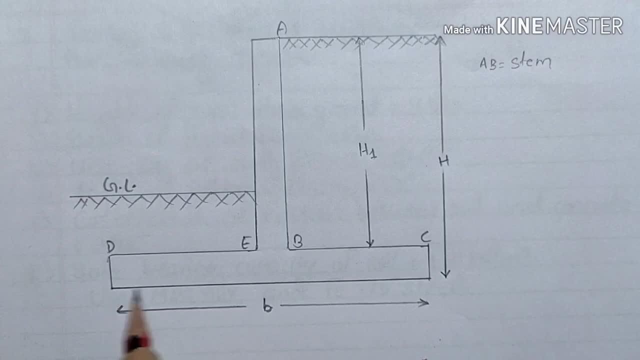 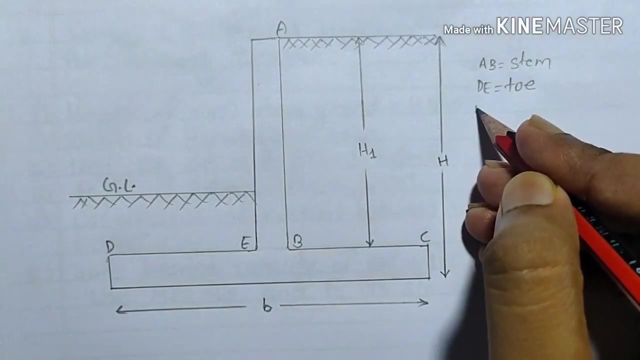 of cantilever retaining wall and b is steam of cantilever retaining wall and, of course, if you retaining wall and our base, this lowest portion is the base, which is denoted by B, and the span DE is our toy and the span BC is our heel. slab BC is our heel. 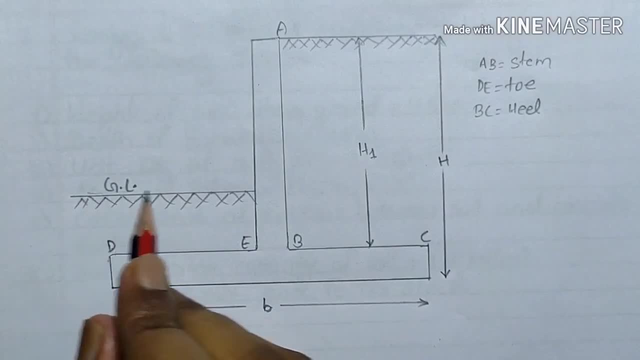 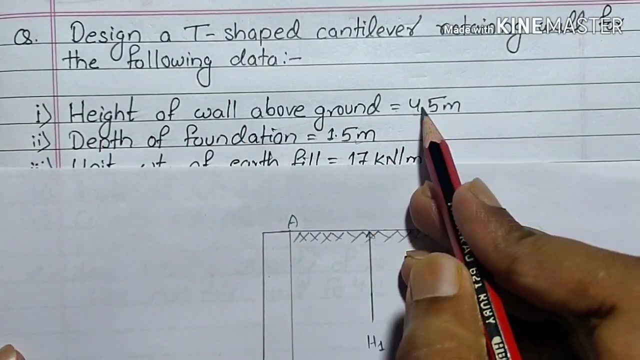 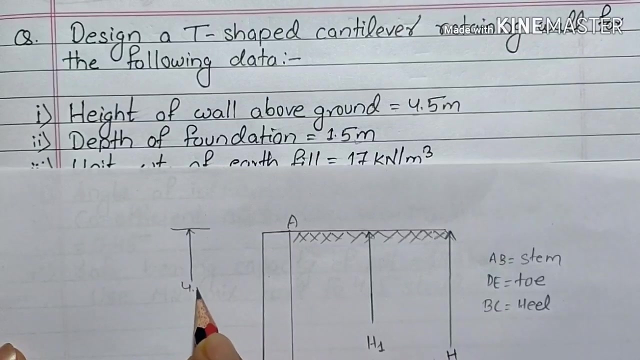 slab. similarly, the depth: this is our ground level, then the depth below the ground level is our footing. this is our footing and in the given question we are provided with. the height of wall above the ground is 4.5 meter means we are provided with the value of this span, which is 4.5 meter, and the depth of. 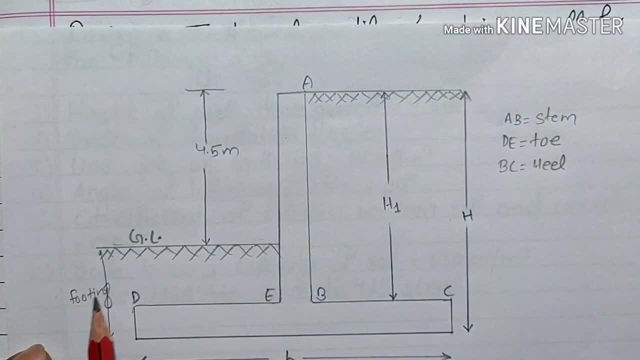 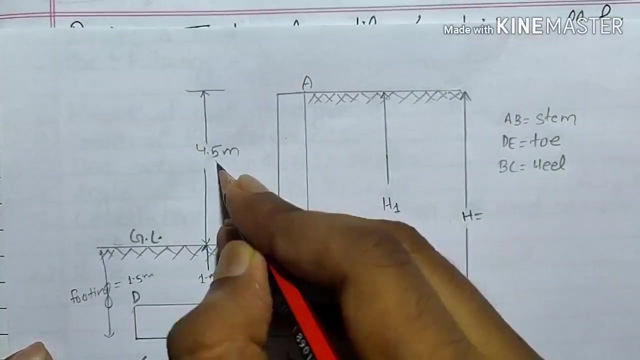 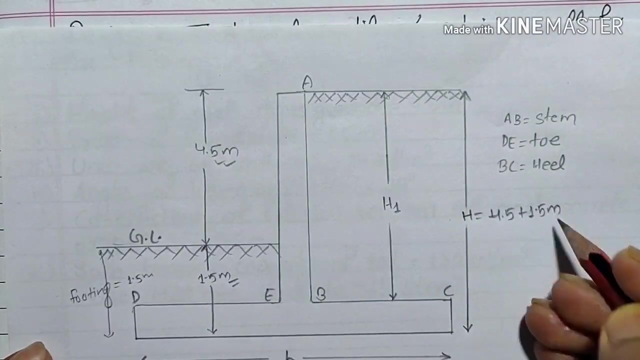 foundation is 1.5 meter means the footing depth is 1.5 meter, so this span is our. 1.5 meter means we have got the value of capital H, which is equals to 4.5 meter plus 1.5 meter. write it down here: 4.5 plus 1.5 meter, which. 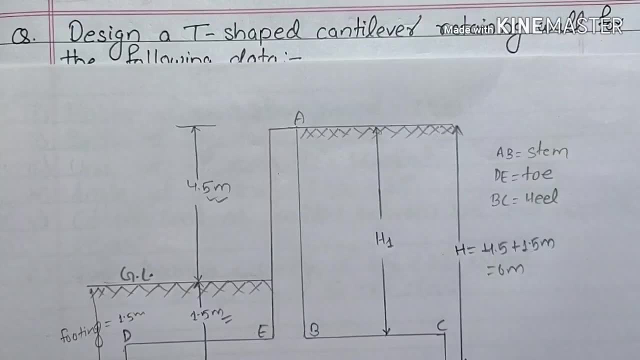 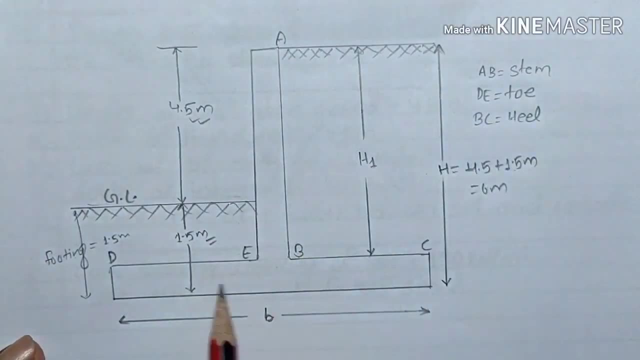 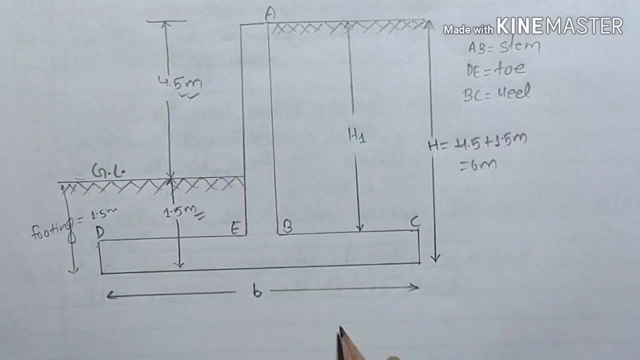 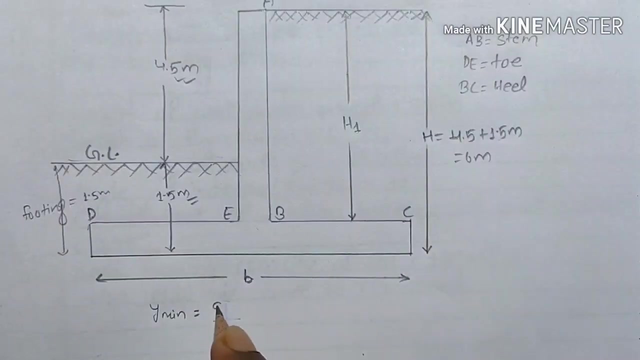 will be equals to 6 meter and in the given question we are provided with the depth of the foundation. in some question one may not. we may not be provided with the span of the footing. then in that case we need to use a formula which is given as Y. minimum means minimum depth of foundation equals to Q. note by: 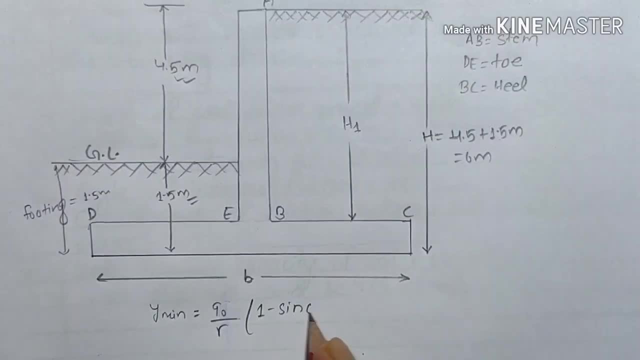 gamma times 1 minus sine Phi upon 1 plus sine Phi to the power whole square in. whenever we are not provided with the depth of footing, at that time we will be applying this formula for calculating the depth of foundation. now we have got the overall depth of the steam, the sorry. 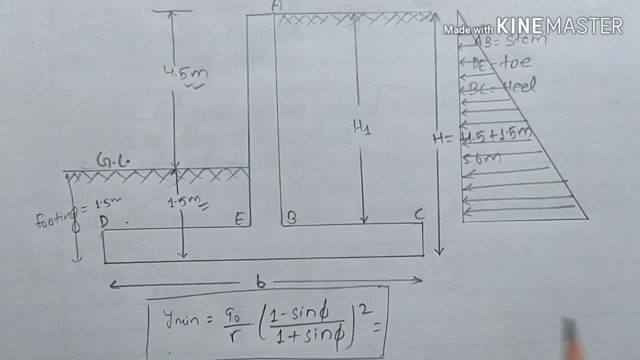 retaining wall. now let's move toward the next step, and here the next step is: the intensity of active earth is related to design means and pressure which is exerted by the soil on the steam of the retaining wall, and the base of the intensity of active earth pressure is given as kA gamma into this height and T. 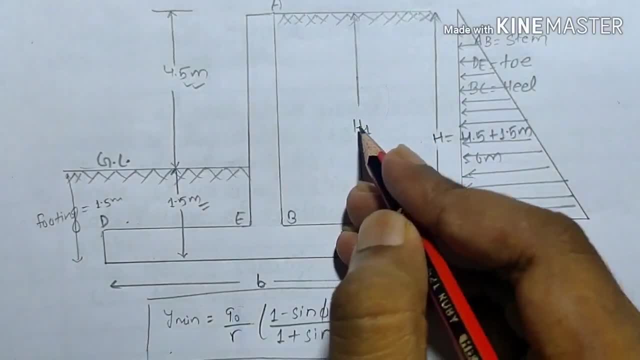 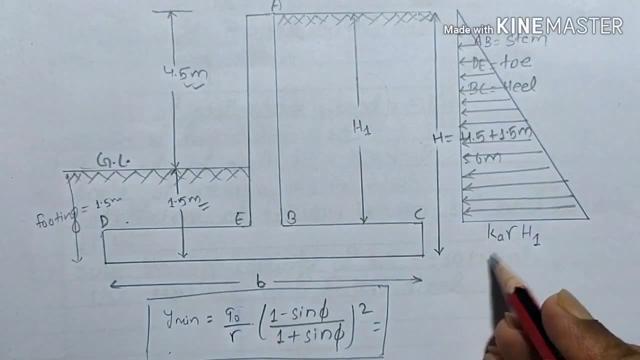 height h1. up to which, up to the, the height at which the soil is exerting pressure, height of soil is h1. so here we need to multiply this ka gamma into h1. now let's move toward the solution of the numerical, and our first step is going to be the right to write down given so unit. 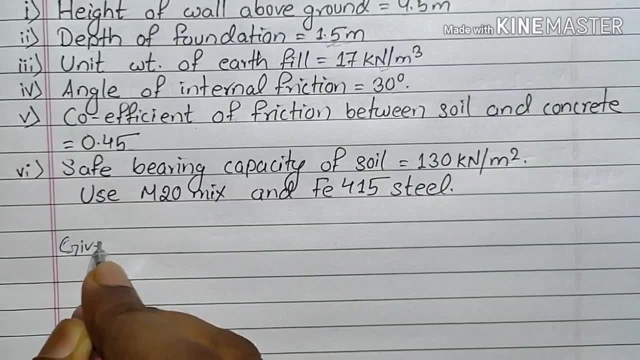 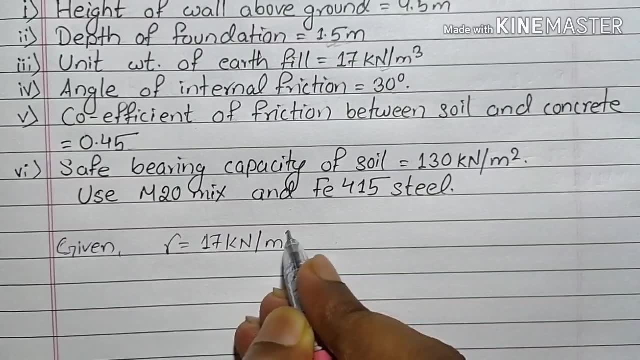 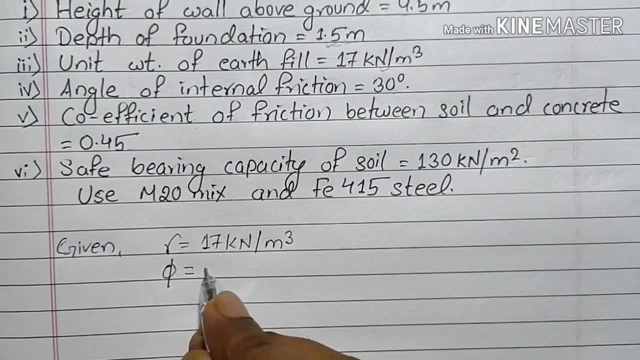 weight of the earth field means here the first given is gamma equals to 17 kilo newton per cubic meter, and the second angle of internal friction is 30 degree, means we are provided the value of phi which is equals to 30 degree, similarly coefficient of friction between the soil and concrete. 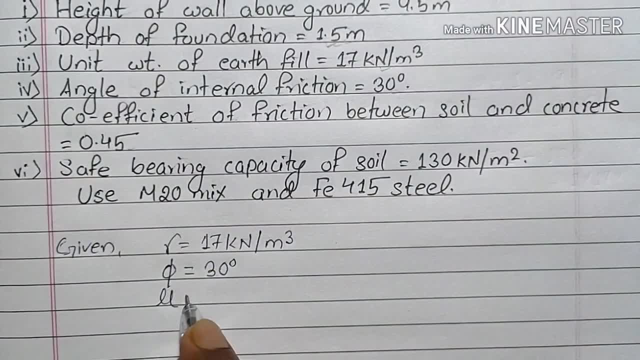 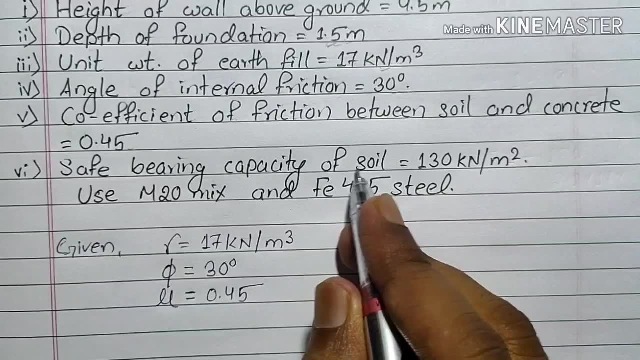 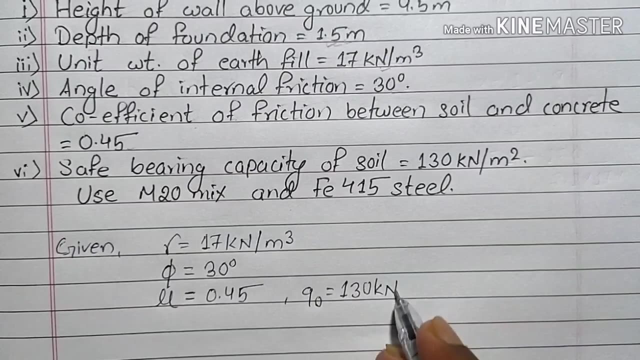 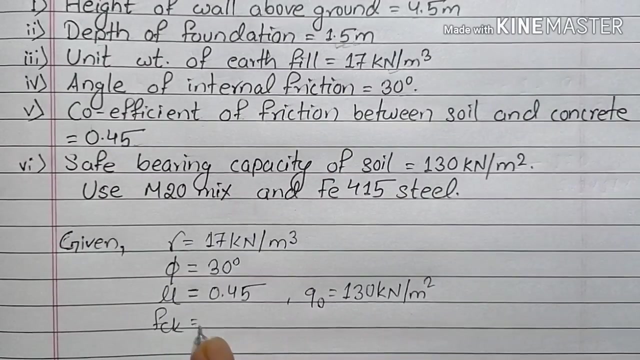 is 0.45 means we are provided with the value of mu, which denotes the coefficient of friction as 0.45, and the safe bearing capacity of soil is 130 kilo, which is denoted by q. notifications equals to 130 kilo newton per square and f? ck equals to 20 newton per millimeter square. 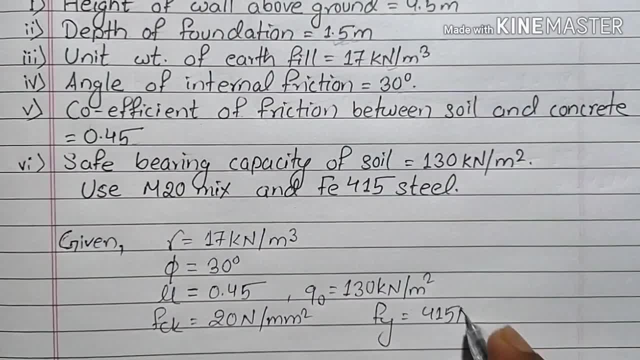 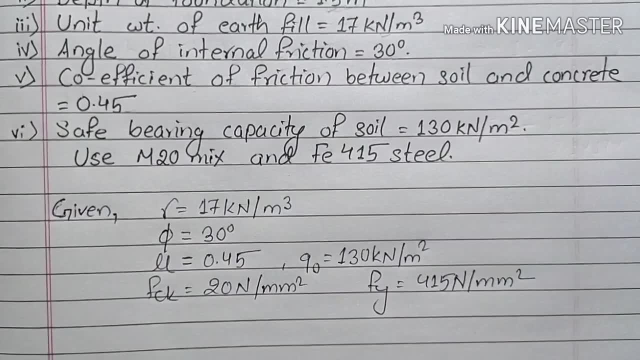 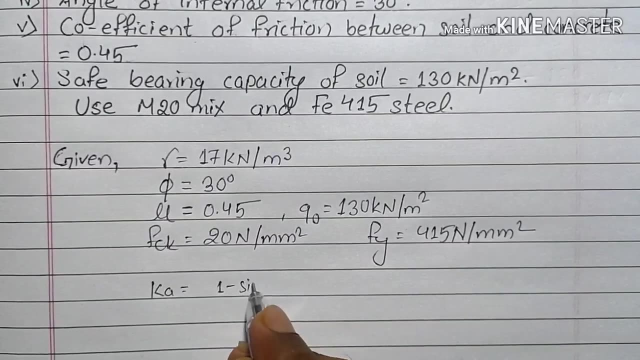 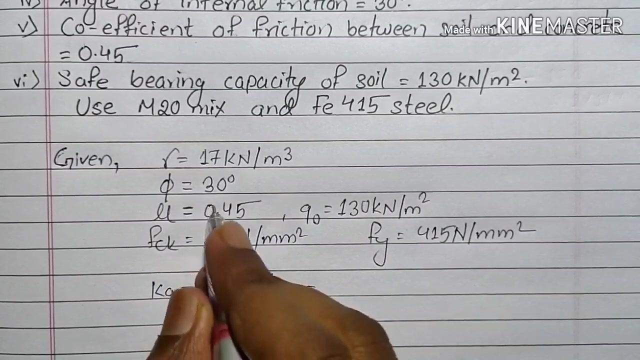 similarly, fy equals to 415 newton per millimeter square. now, as a, we are given the value of Phi. so let's find out the coefficient of active pressure. that is, Ka equals to 1 minus sine Phi upon 1 plus sine Phi. on putting the value of Phi equals to 30 degree, we will get coefficient of active earth. 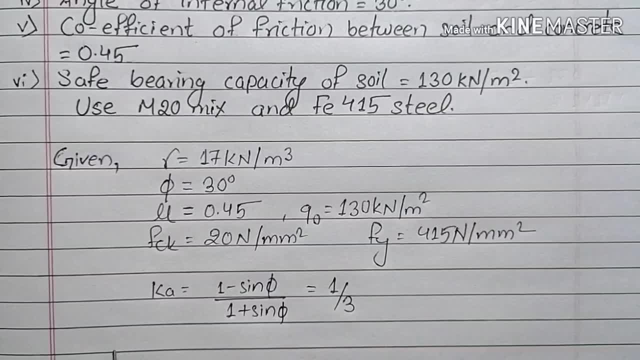 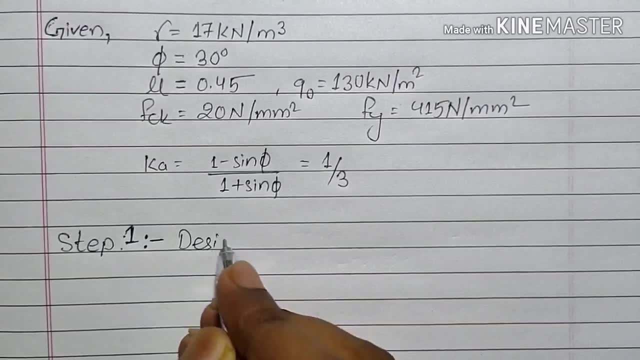 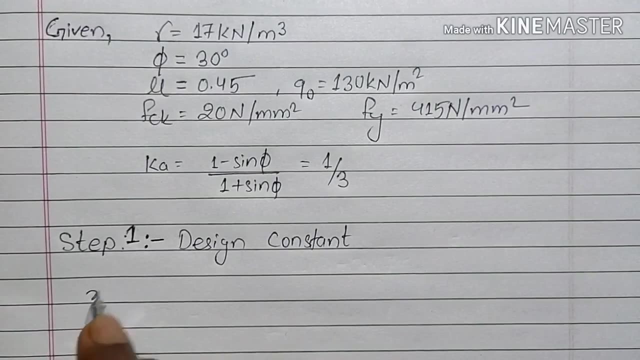 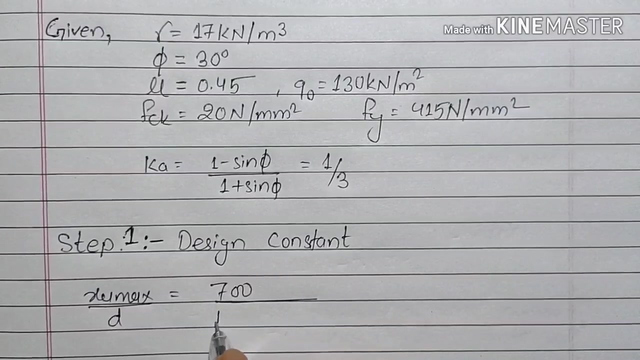 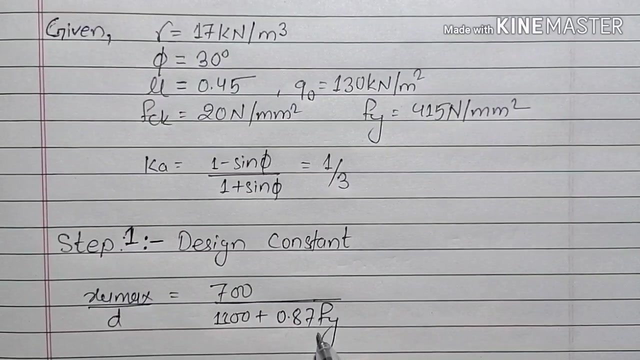 pressure. Ka equals to 1 by 3. now let's move toward step 1 here. in step 1 we will be finding the design constant and we have formula for finding design constant like: X, u max upon D equals to 700 by 1100 plus 0.87 f Y. now put the 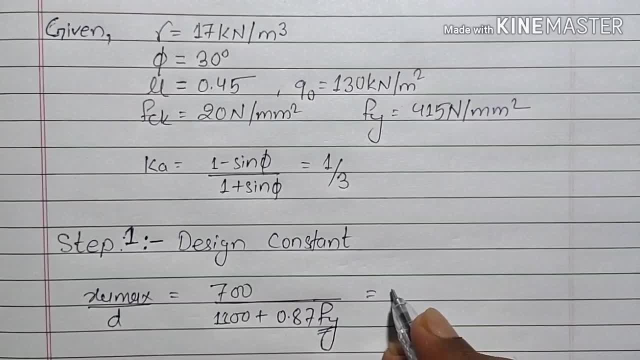 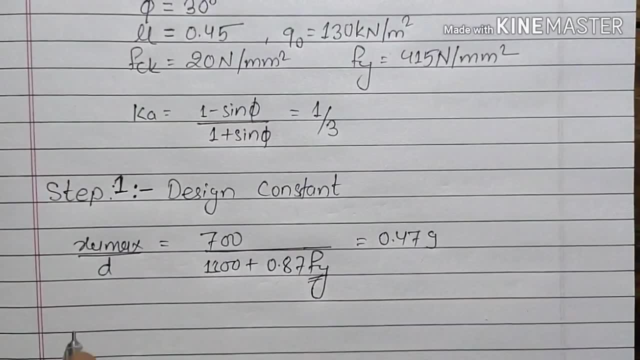 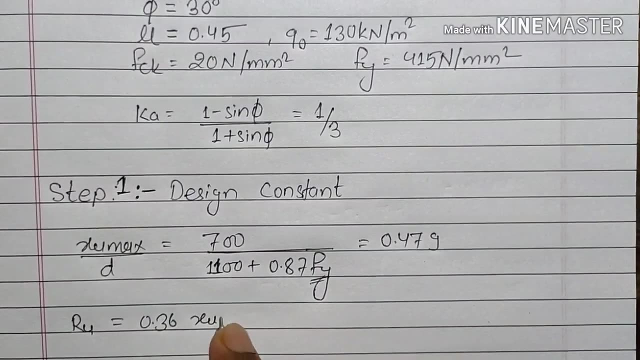 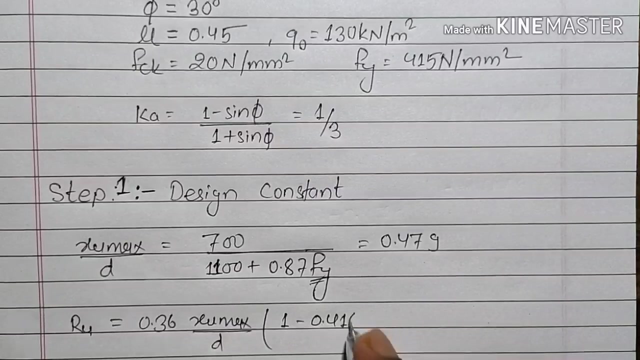 value of f? y is equal to 450 and you will get X? u max by D equals to zero point four seven 9. similarly, our second design constant is ru and we have the formula for ru equals to 0.36 x? u max upon d times 1 minus 0.416 x? u max upon d. now put the value of x? u max. 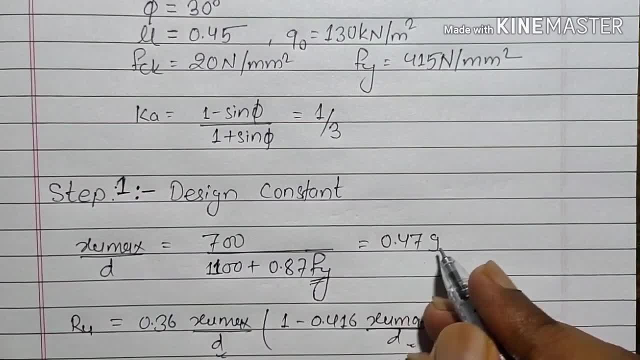 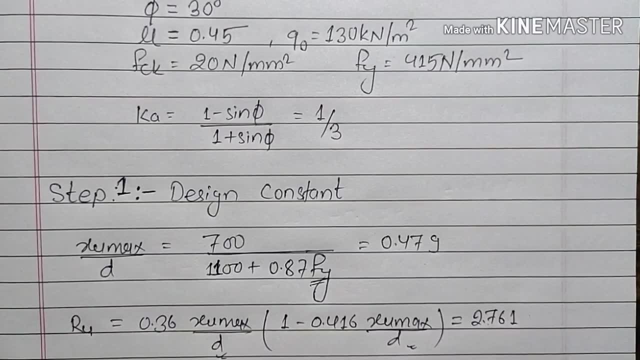 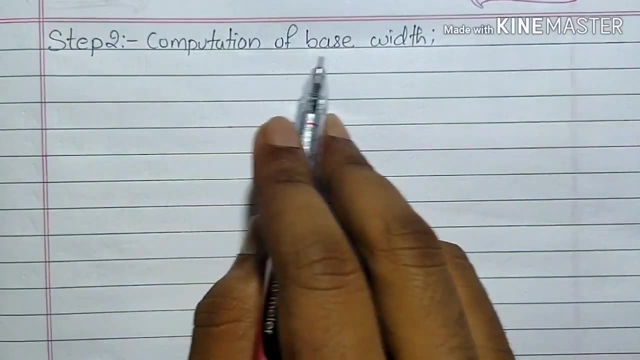 here x max by d, upon here d, that is 0.479, then you will get the value of ru equals to 2.761. now let's move to our step 2. in step 2 we need we will be finding the base width. that is the value. 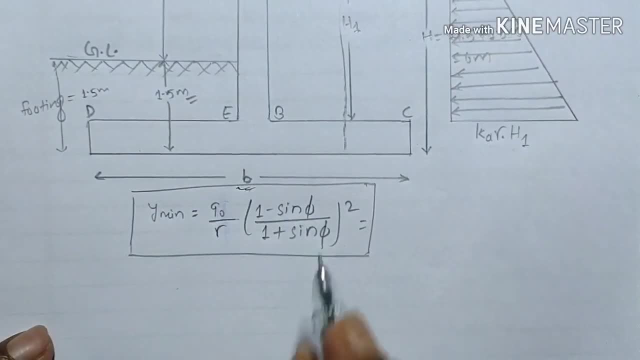 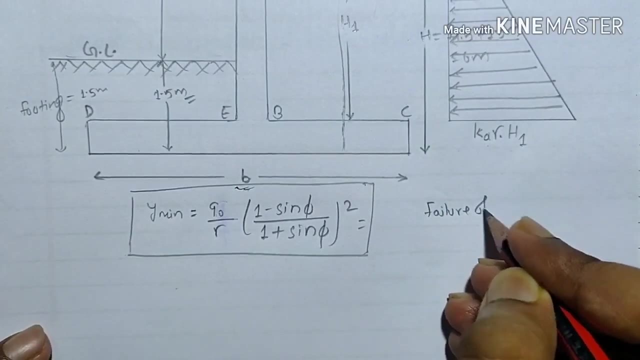 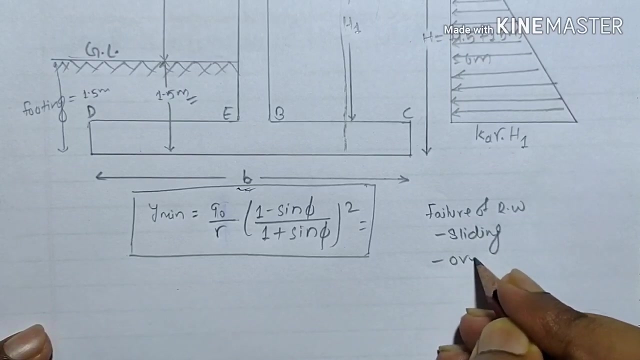 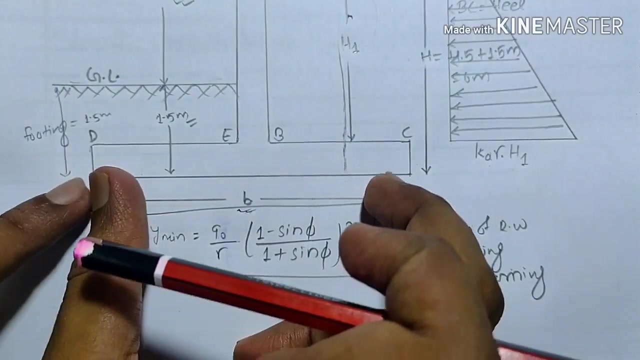 of b, we will be finding this value. and here, students, i would like to tell you one thing: that the failure of retaining wall is mainly due to sliding, sliding and overturning. overturning occurs when the retaining walls turn from the about the point d and the sliding means 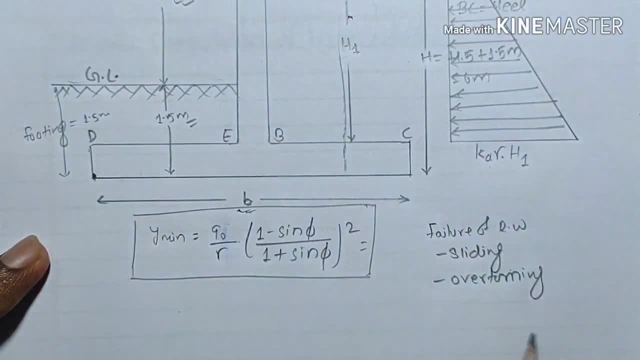 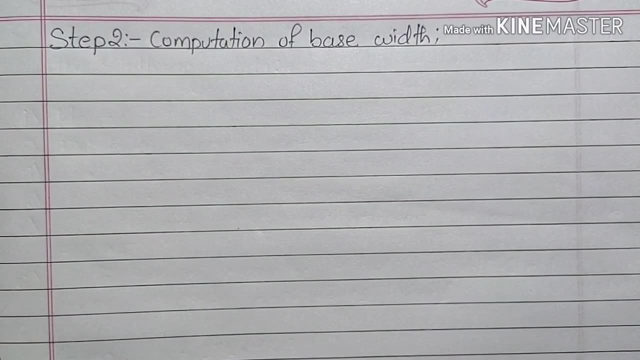 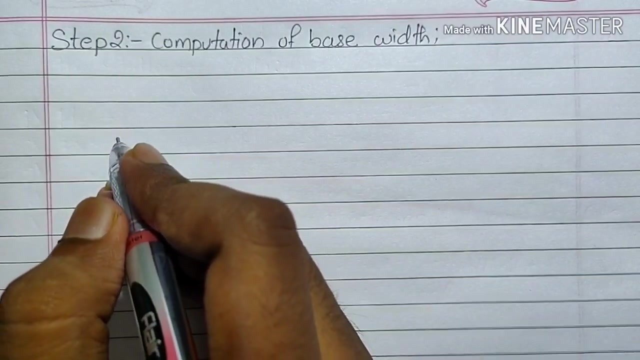 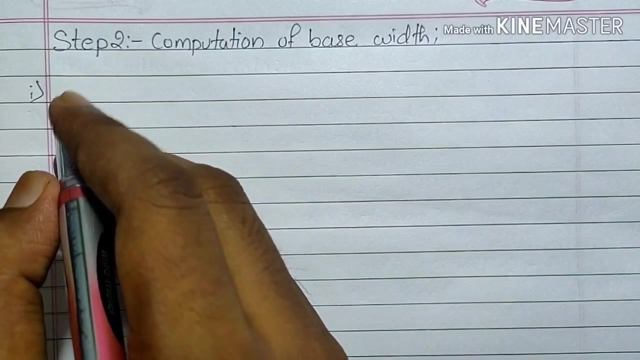 the base of the retaining wall is displaced from its original, from its original position. so we need to find the width base of the retaining wall on both, on the both consideration about one about the overturning and other against the sliding. so first let's uh find out the base against overturning. 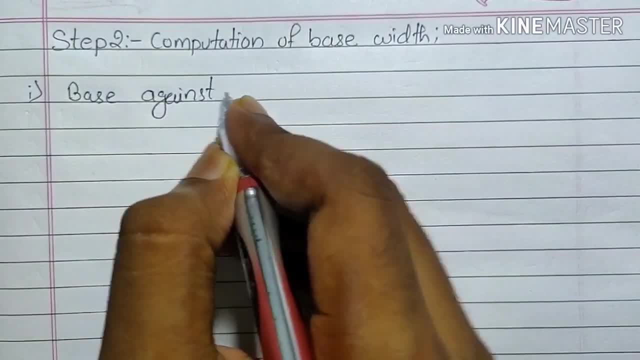 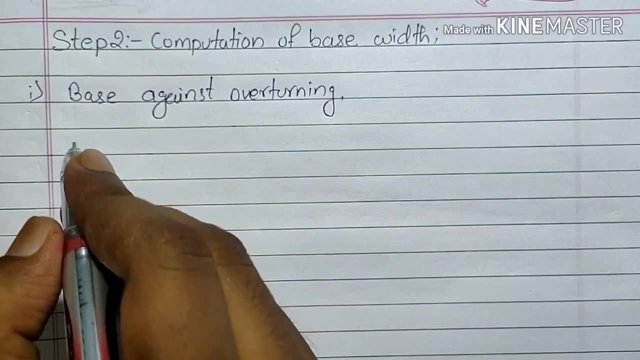 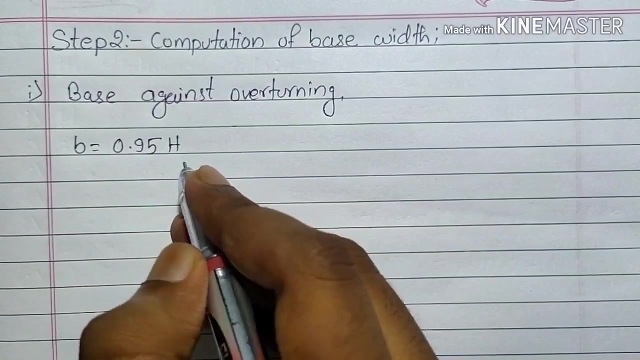 base, agnest, and we have the formula for basic finding the base of the Beat the ice, and we are considering the only sides that we have right now. So let me verify that. the Turner sagen we don't have a classic root from here, but actually, if we like to know what is this zeta model itsule a z to the channel. 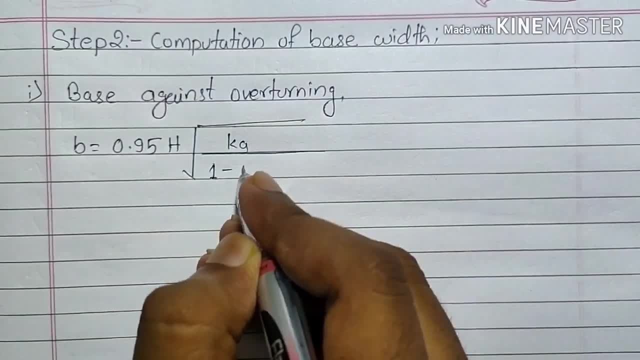 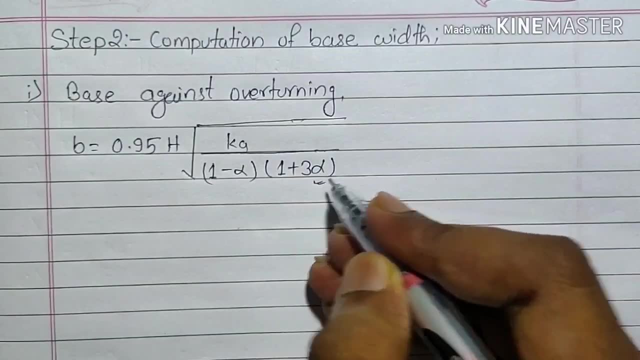 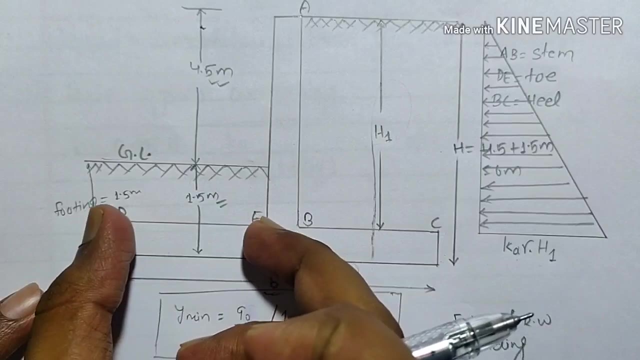 let's first of all, we need to calculate theério to the당 ü, and these are the roots of this. a is indeed that we are talking about. the root to the county n is in the position we have to take u n to equal to infinity. huh, that means it is also intended to be equal to infinity, or minus 1 square m. 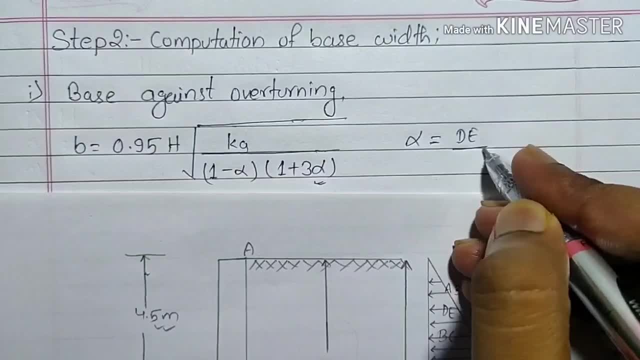 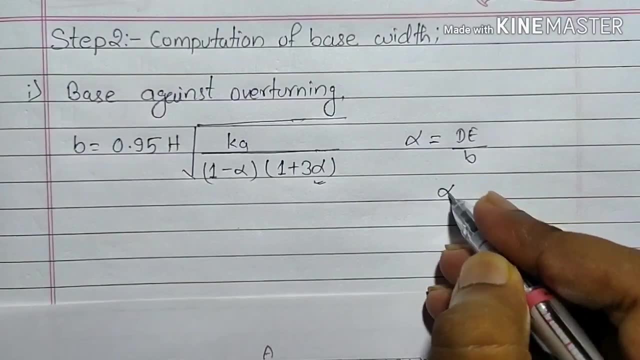 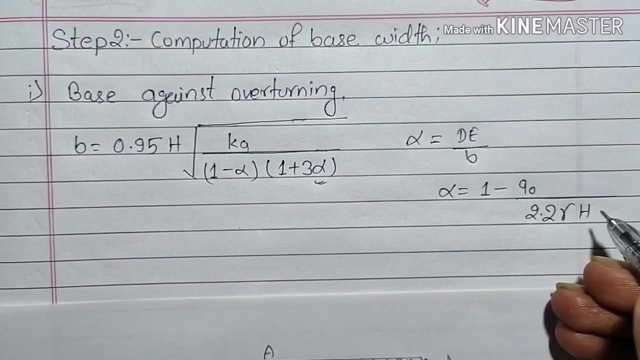 The starting substitution has been obtained by taking n equals to n, alpha equals to DE upon b and we have a formula to find the value of alpha, which is given as alpha equals to 1 minus QNOT by 2.2 gamma H. Now let's write, put down the value of: 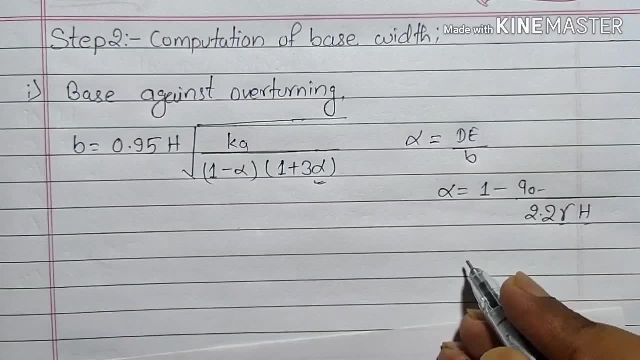 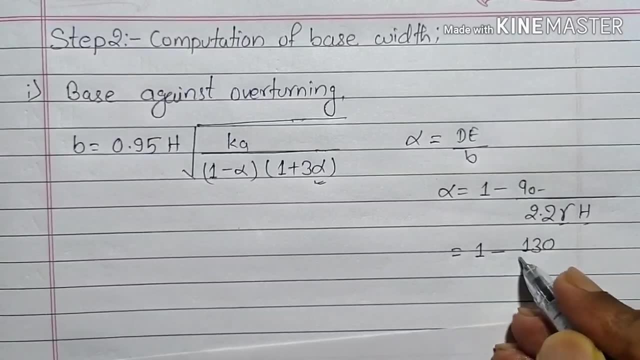 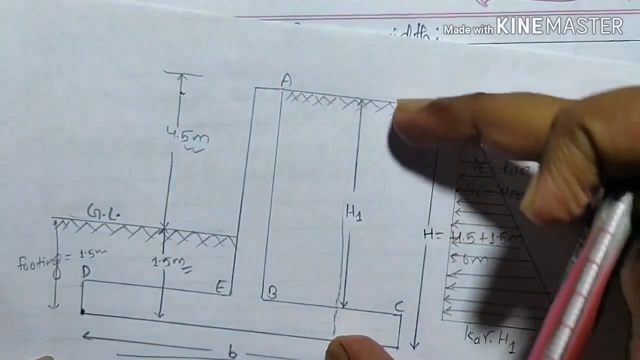 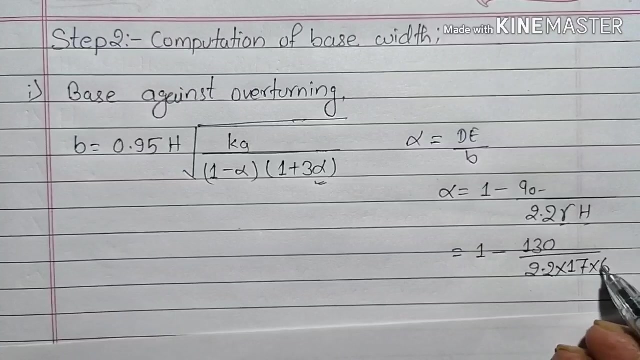 QNOT, gamma and overall H, and then find the value of alpha, and here it will be 1 minus QNOT is 130 by 2.2 and the value of gamma is 17 and the height means overall height. this height means 4.5 plus 1.5, which is equals to 6 meter. so put it here and you will get. 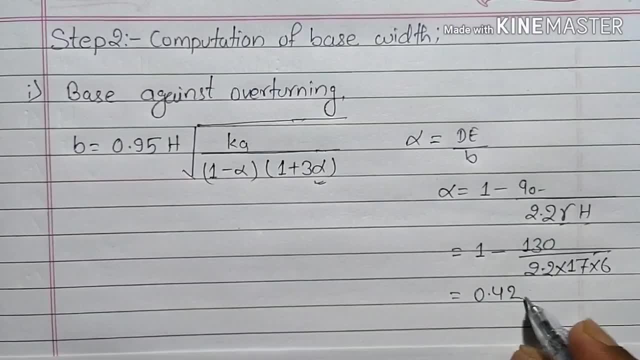 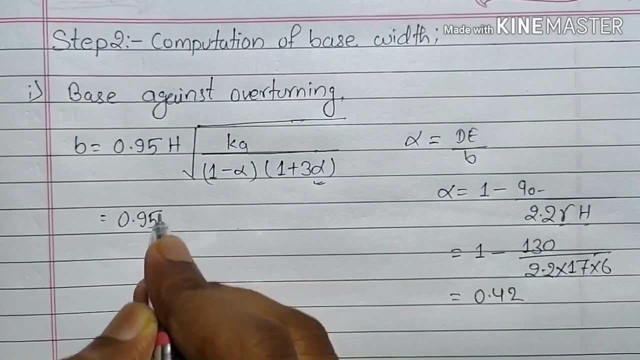 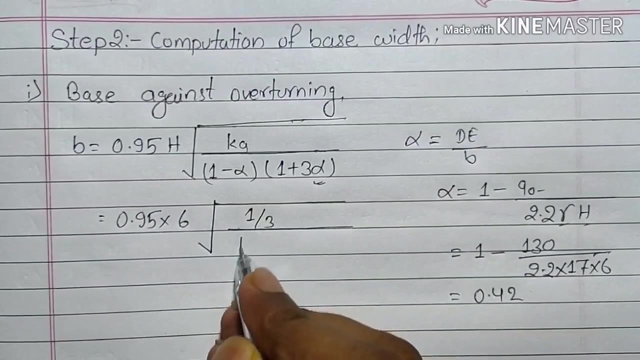 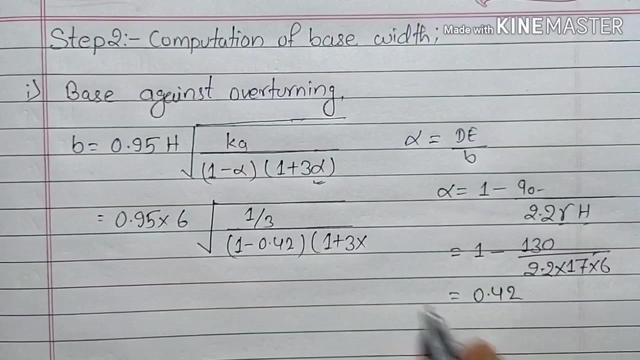 the value of alpha equals to 0.42.. Now put down the value of alpha in this question, then we will have 0.95 into 0.42.. H is 6 times root under KA is 1 by 3 upon 1 minus. alpha is 0.42 times 1 plus 3 into alpha. 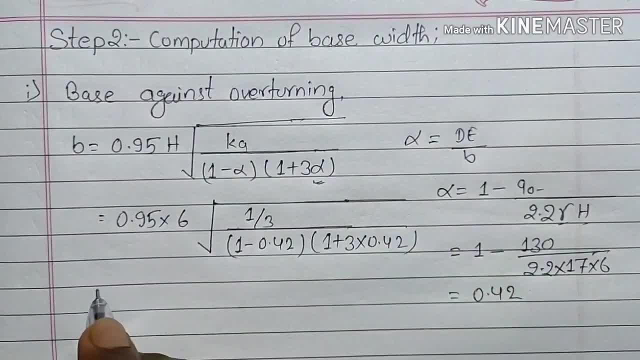 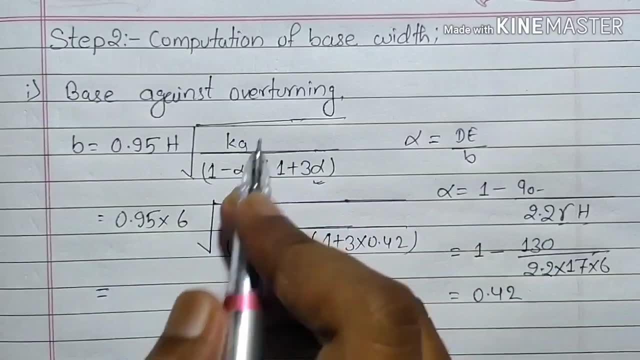 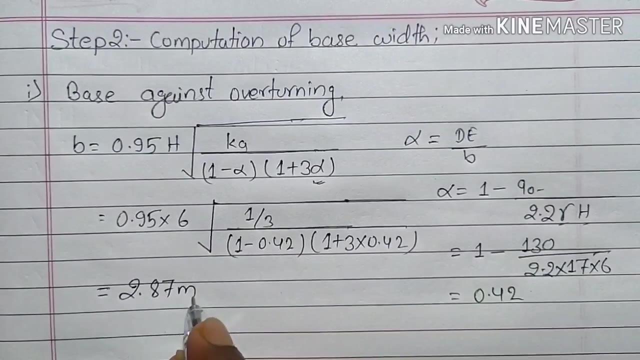 is 0.42.. On solving this, we will get the value of b, which we need to consider for providing making the retaining wall safe against overturning, and we will get its answer as G2.8.. Now we will again find the base, but this time we will be finding the base against sliding. 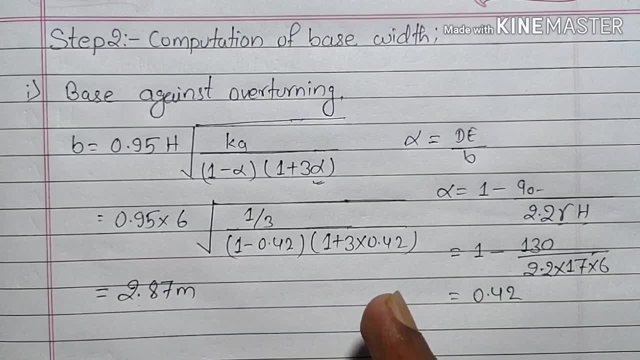 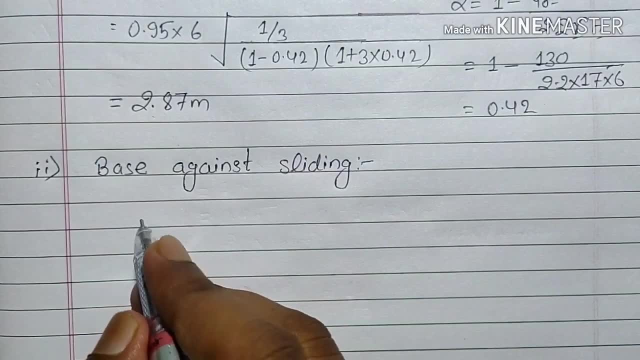 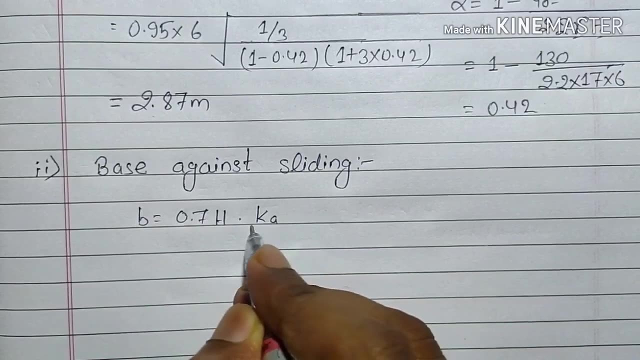 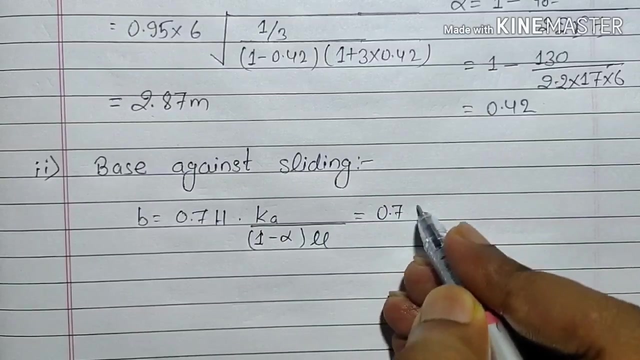 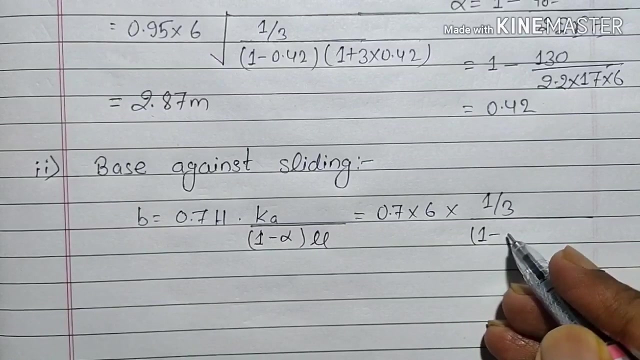 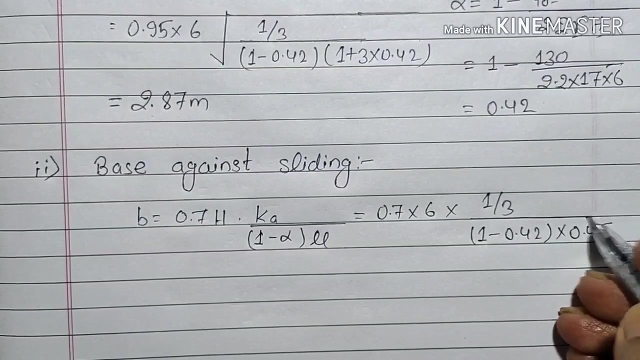 means base, in order to protect the retaining wall from the sliding. and the base against sliding is given by using the formula d. equals to 0.7 H times KA by 1 minus alpha times mu. Now put the value of alpha Here: alpha is 0.7 into 6 times 1 by 3 by 1 minus alpha, value is 0.42 into mu, mu is 0.45. 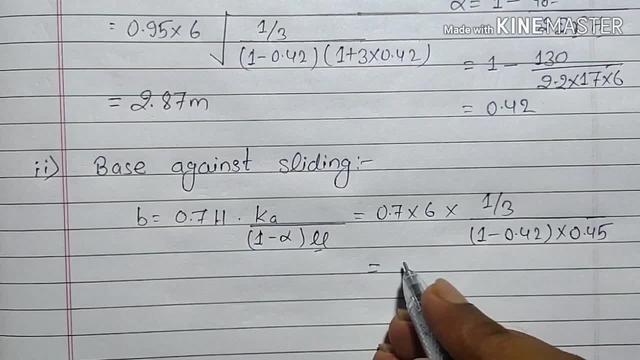 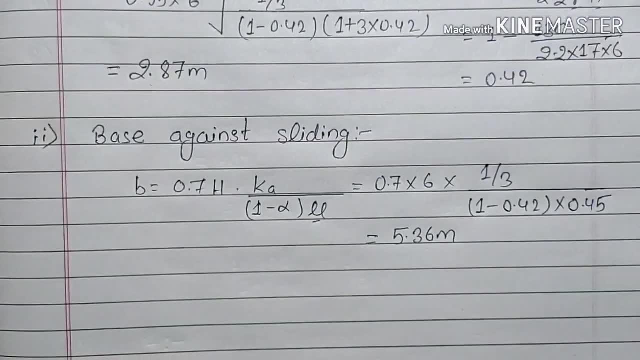 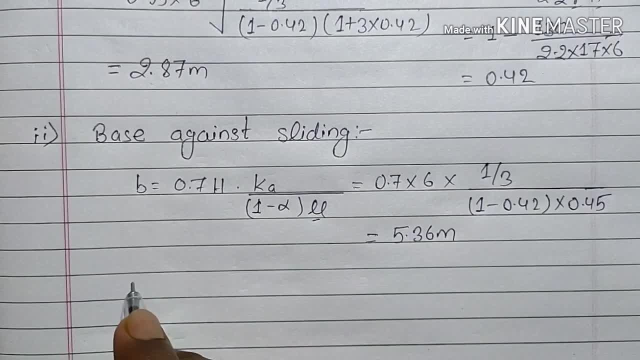 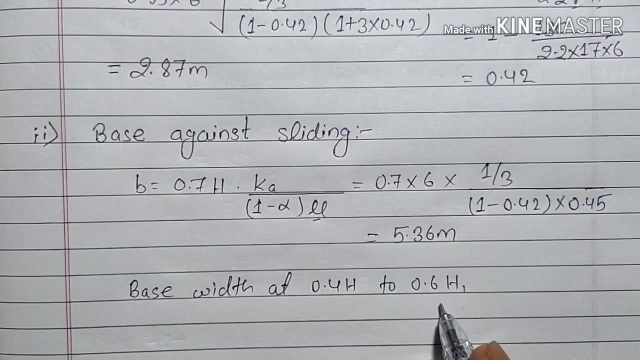 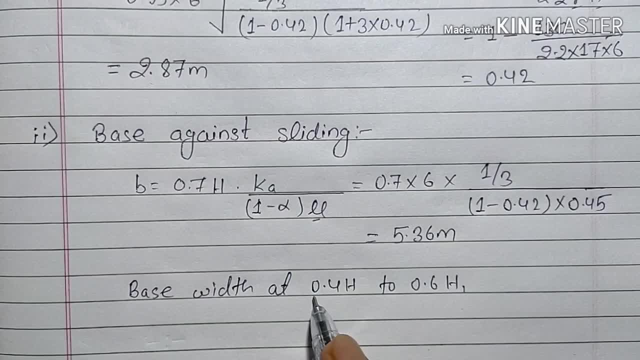 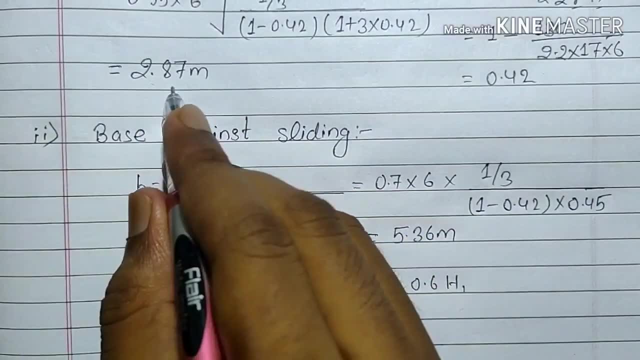 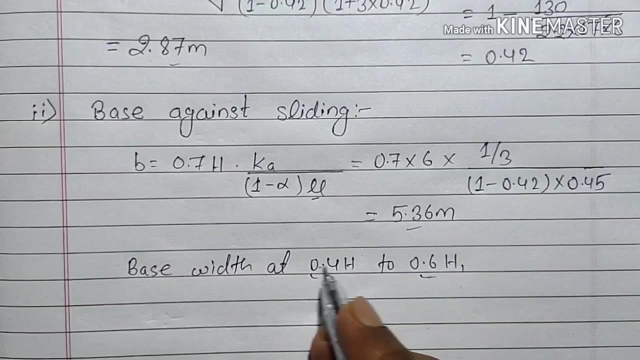 considered that the base width from the range 0.4 H to 0.6 H is considered as the safest one. so we do not. we will not take these two base, but we will take new base. as per this assumption, which is 0, you can take either 0.4 H, 0.5 H or 0.6 H. 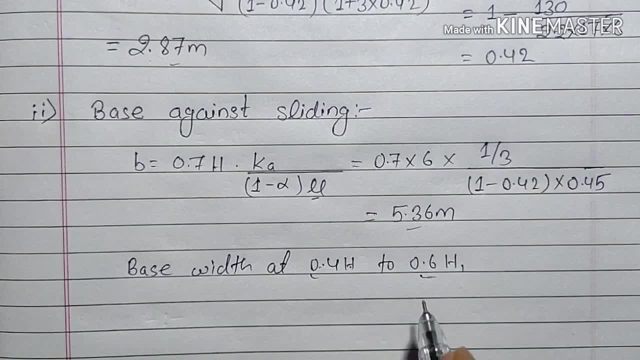 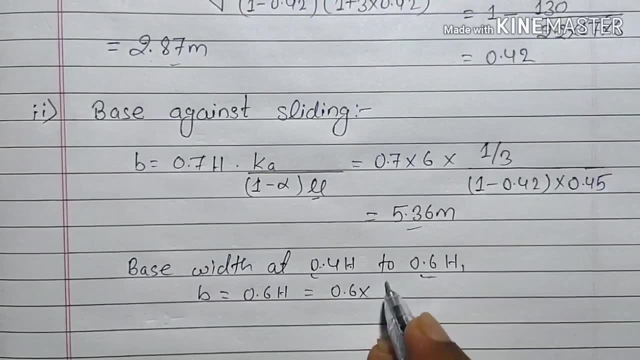 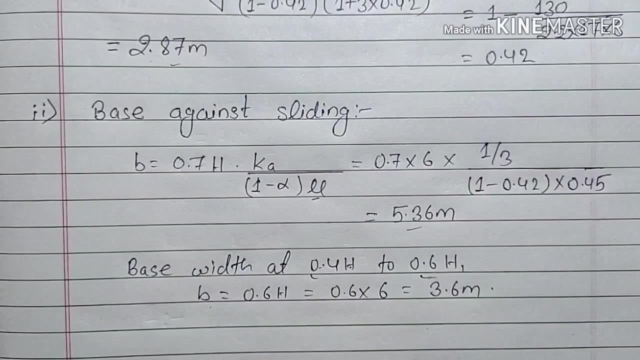 so let's take it, let's proceed. taking the maximum value of B, that is, B equals to 0.6 H. so 0.6 into 6 equals to 3.6 meter, and this is going to be the value of small b. now time for the width of. 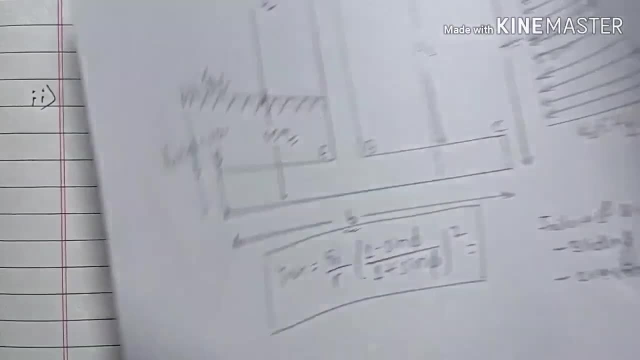 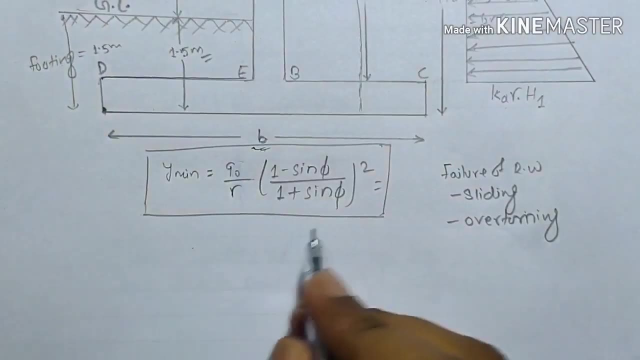 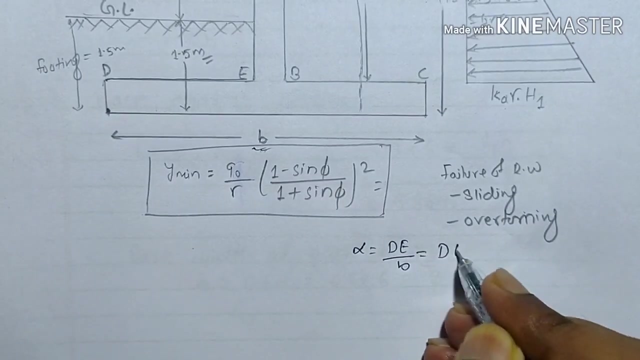 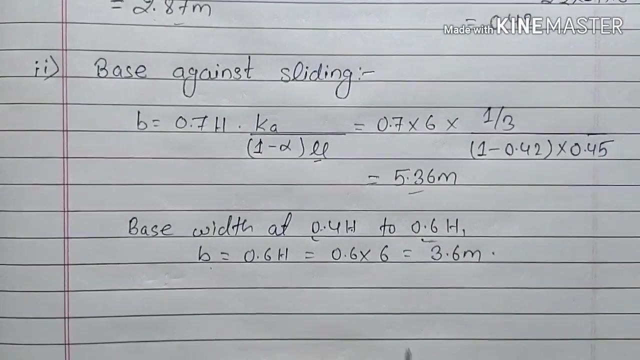 twice slab. and here we need to find the value of D E, and I already told you that alpha was the ratio of D E by B. so our D E is going to be alpha times B, and we have got the value of alpha and B as well. so our base width- sorry, our toy slab. 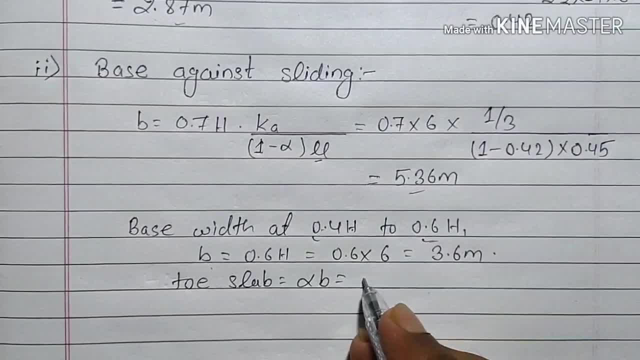 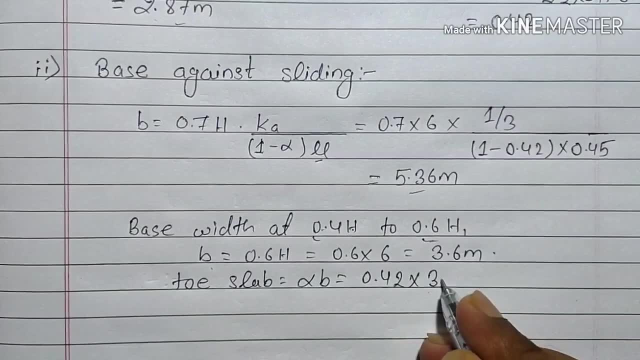 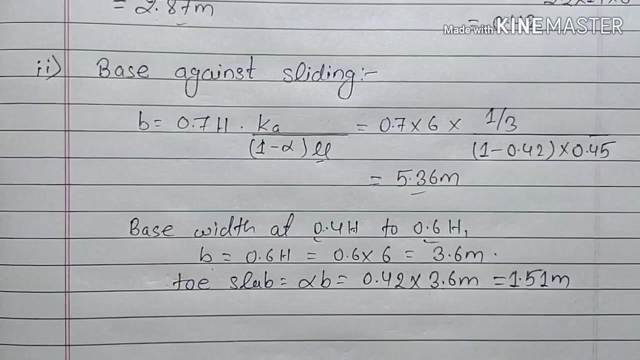 length is going to be alpha b equals to value of alpha is 0.42 into b is 3.6 meter and this total will be equals to 1.51 meter. similarly, we need to find the thickness of base means. we need to find 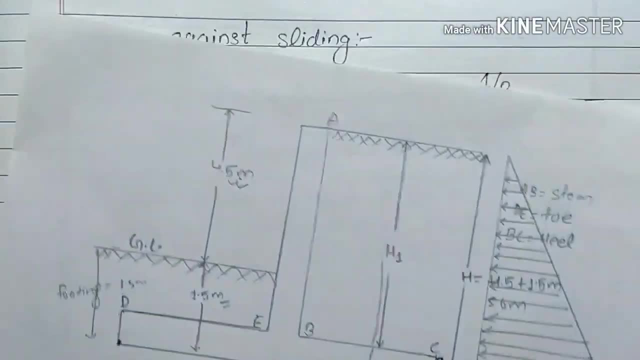 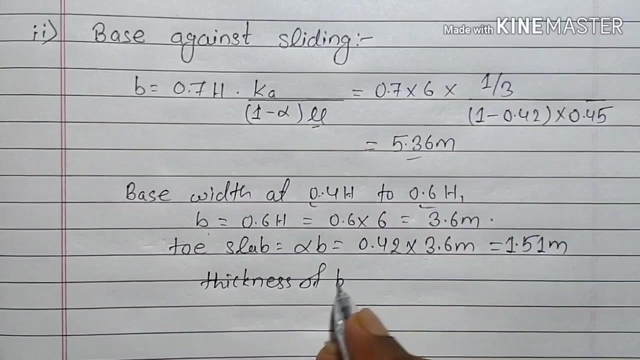 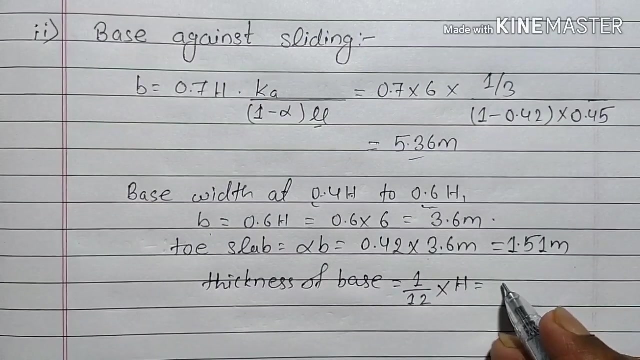 this length, or the thickness which is usually taken as thickness of base, equals to 1 by 12 times h, and our h is 6 meter. so we will get 1 by 12 into 6 equals to 0.5 meter. now we have got the. 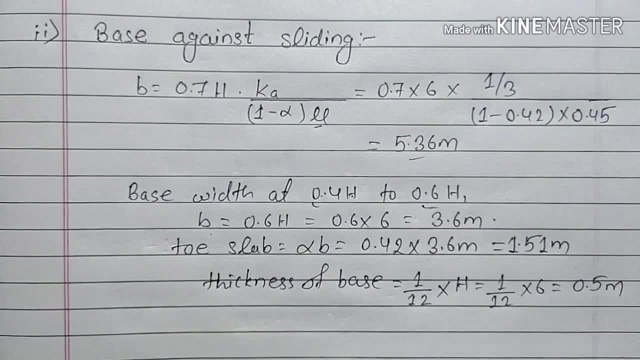 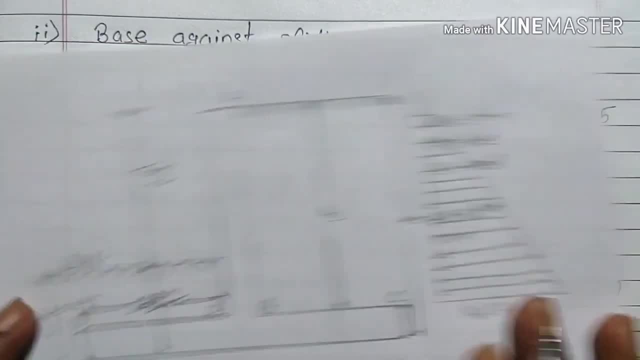 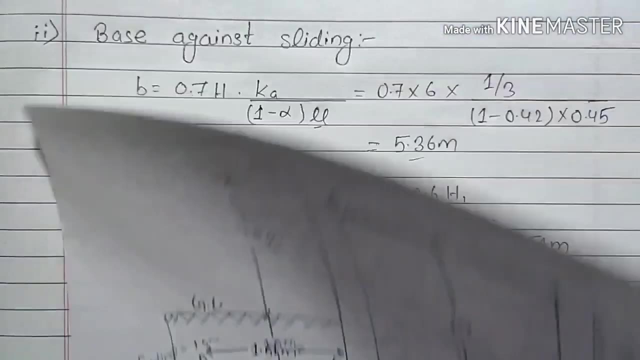 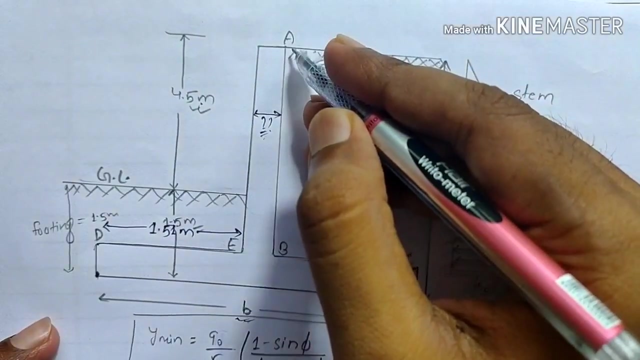 value of d e, which is equals to 1.51 meter. 1.51 meter and the thickness is 0.5 meter. now let's move towards the step 3.. in step 3, we will be calculating the thickness of steam, as we all know that our steam is a- b and we need to find the thickness means we need to find. 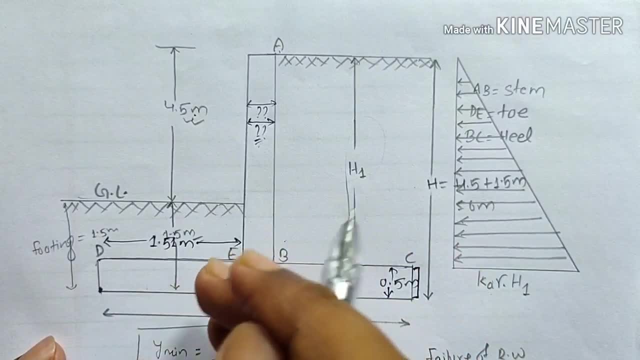 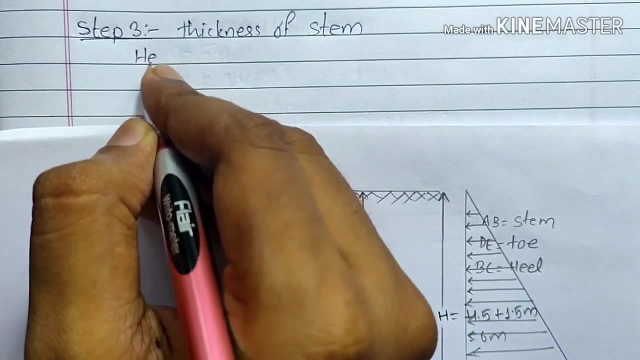 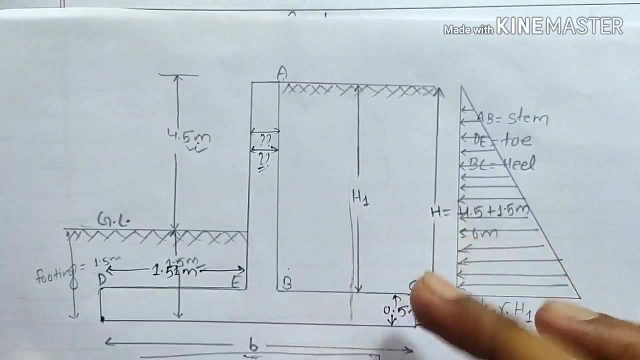 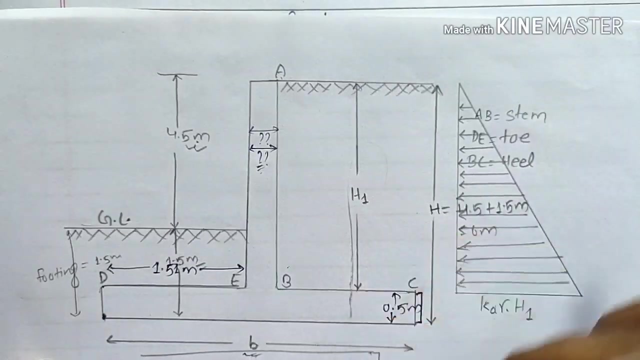 this value and let's learn how to calculate the thickness in this step. for that, we will begin with the height of steam and we have. the overall height of the retaining wall is 6 meter and we have calculated that the thickness of base slab is 0.5 meter. so our height of retaining wall, that is, h1, will be 6 minus 0.5. 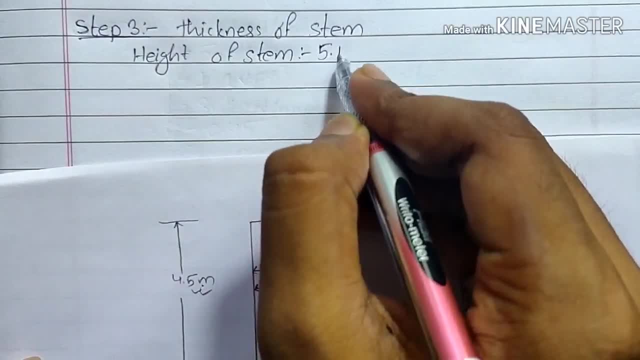 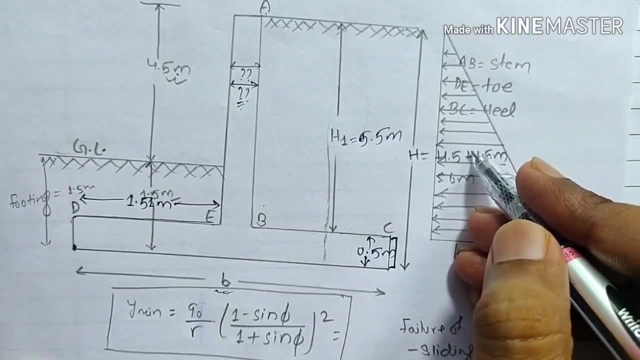 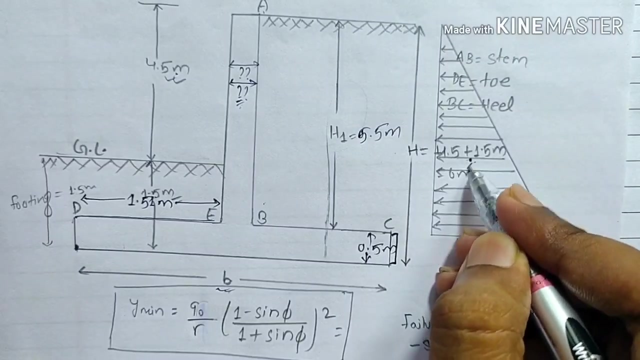 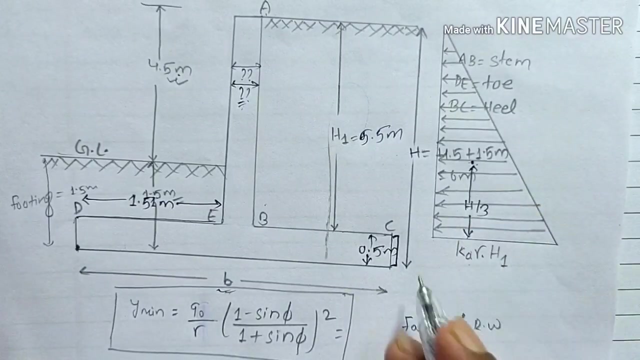 meters. so let's write it down: height of steam is 5.5 meter. now come towards the this diagram, triangular portion, which is the intensity of active earth pressure, and always remember that the intensity of active earth pressure, ka, always acts at height h by 3 from the base. so we will have 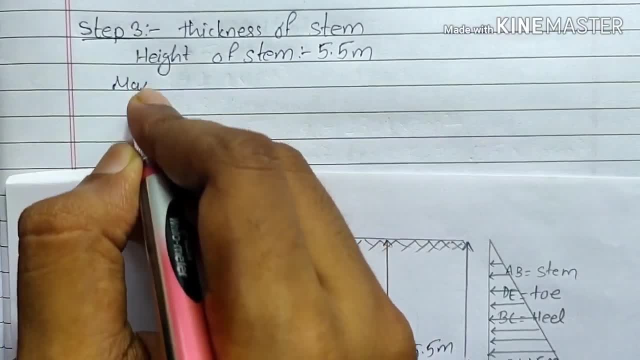 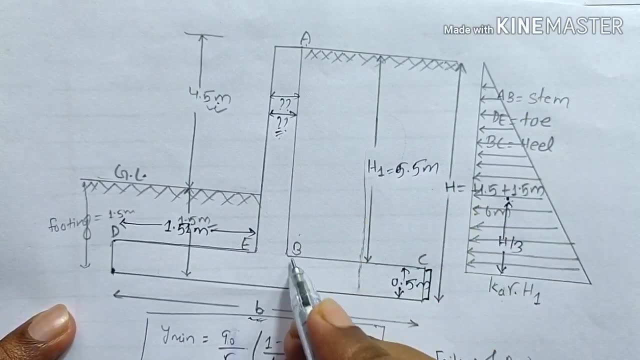 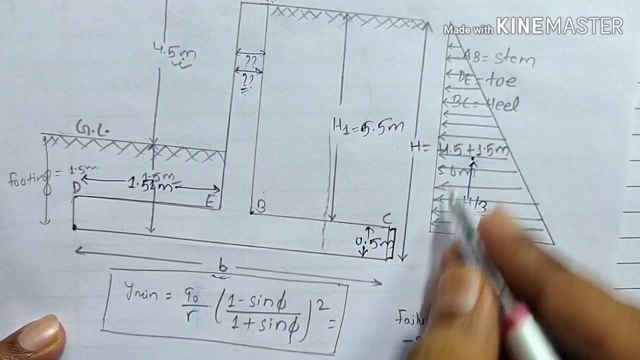 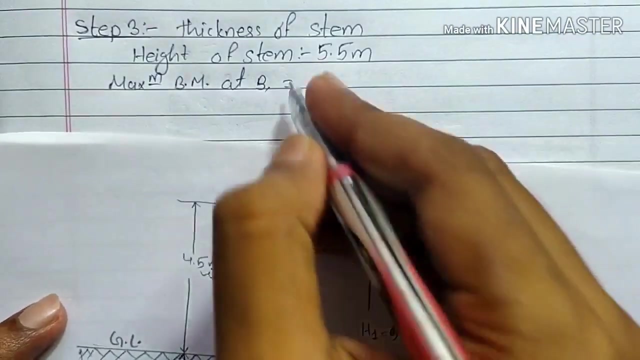 here. bending moment at b means how much moment will occur due to this soil portion, soil loading, and for that we have, we need to find the pressure diagram. we need to find the area of this diagram which is given, as this is triangular. so half into our base value is ka, gamma h1, so write it down. 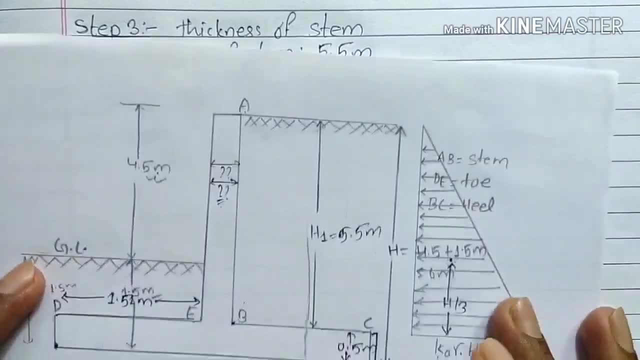 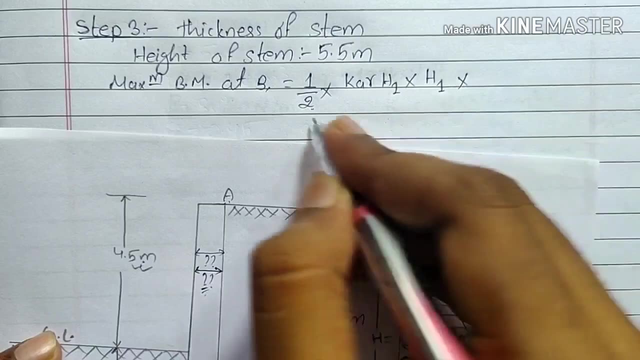 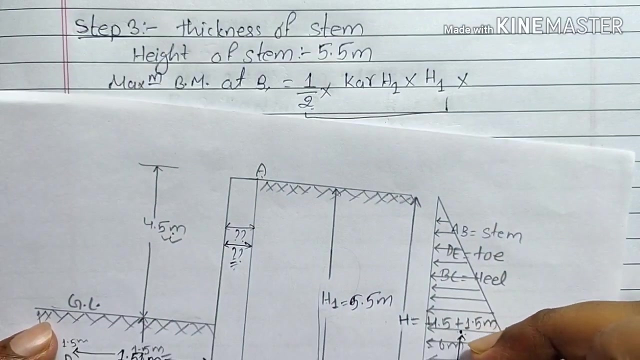 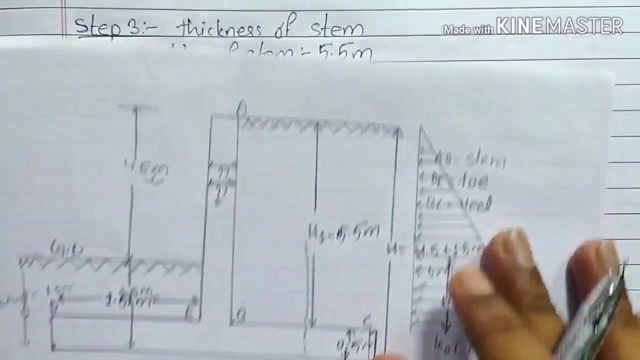 here ka gamma h1 into this is our half into base times height and our height is h1, so h1. now this is our force. this area of this triangle gives force. now we need to multiply this by the span to the up to the cg, and i told you that ka acts as distance h by 3 from the base. so multiply this by. 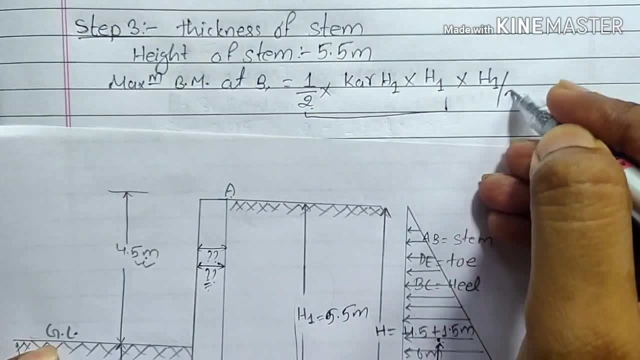 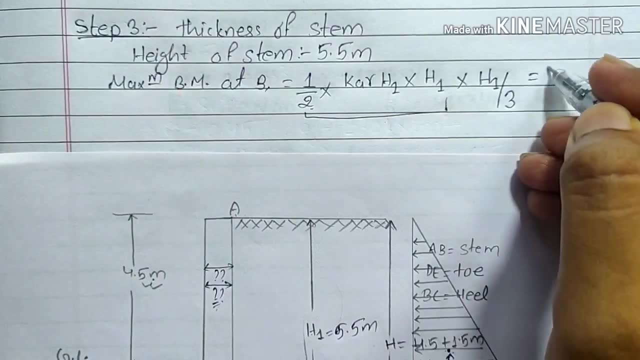 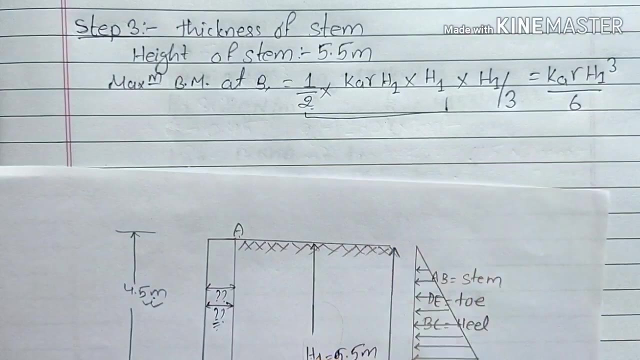 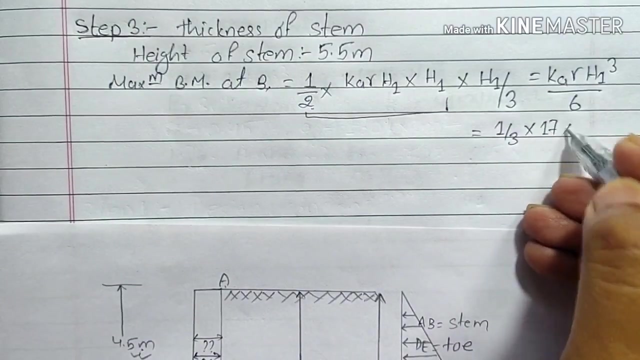 h1 by 3, because this is our h1 by 3. so finally we will have ka gamma h1 to the power, 3 by 6, which will give us a bending moment. now put the value ka value is 1 by 3 into 17, into the value of h1 is. 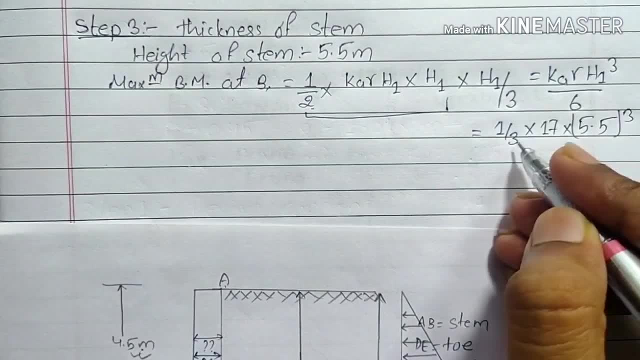 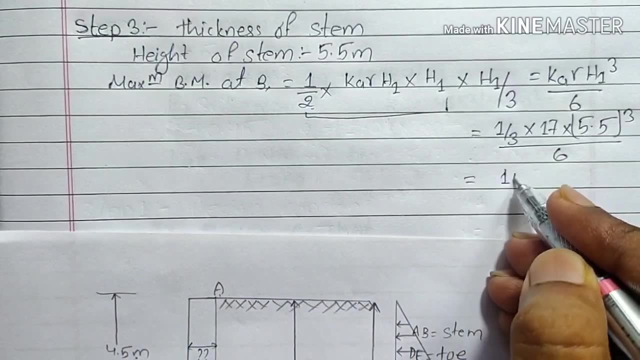 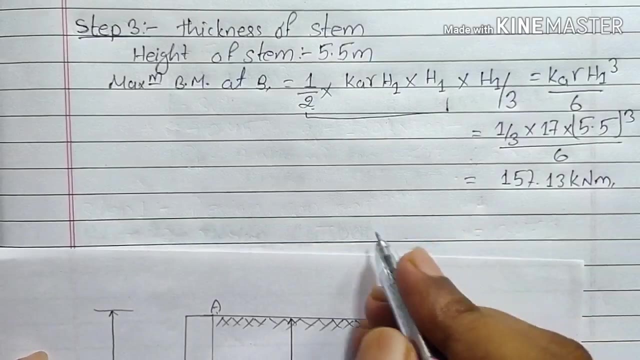 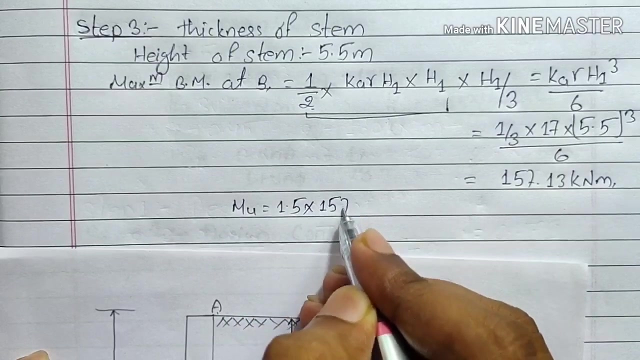 5.5 to the power 3, divided by 6, we will get the value of maximum bending moment as 157.13 kilo newton meter. similarly, we need to apply the factor of safety for finding mu, so mu is going to be 1.5 times 157.13. then the finally, we will get mu equals. to 235.69 kilo newton meter. now time to find the effective depth. now we have a formula for finding effective depth that is: d equals to root under mu upon ru times b. so put down the value we have. mu equals to 235.69 into 10, to the power 6 divided by ru. 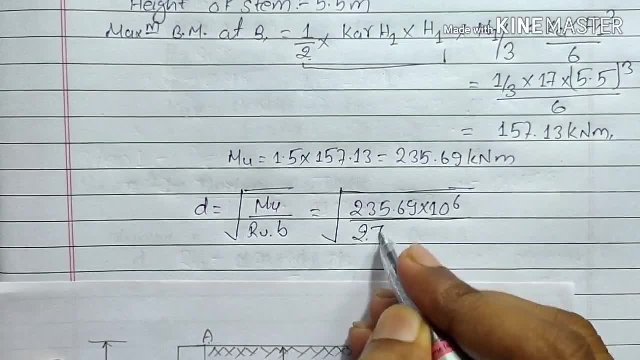 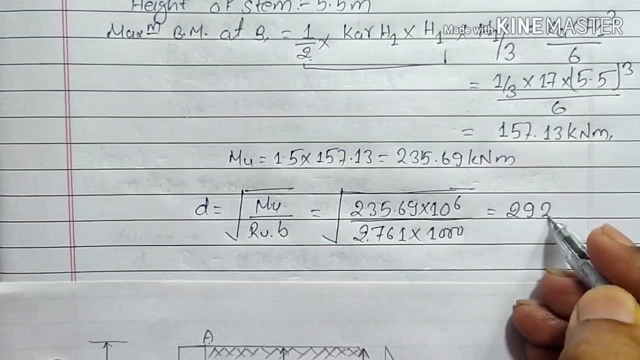 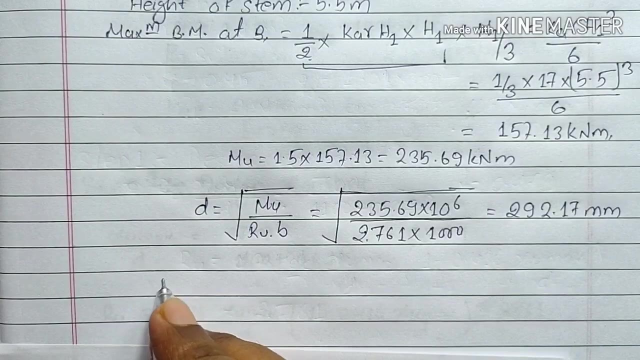 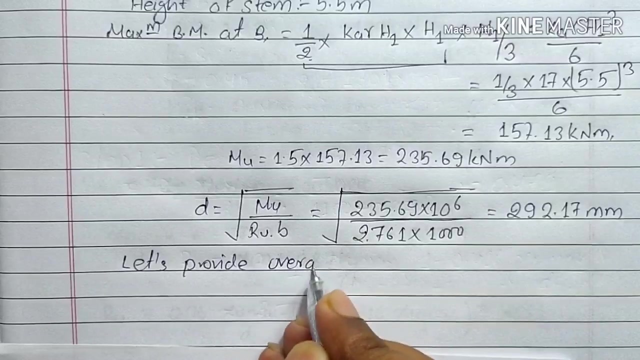 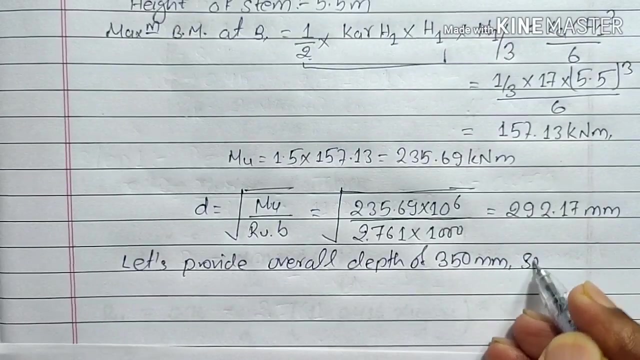 the value of ru is 2.761 into thousand and from here we will get the value of small d as 292.4 into 0.17 millimeter. now let's provide overall depth of 350 millimeter, so let's write it down. let us provide overall depth of 350 millimeter so that 60. 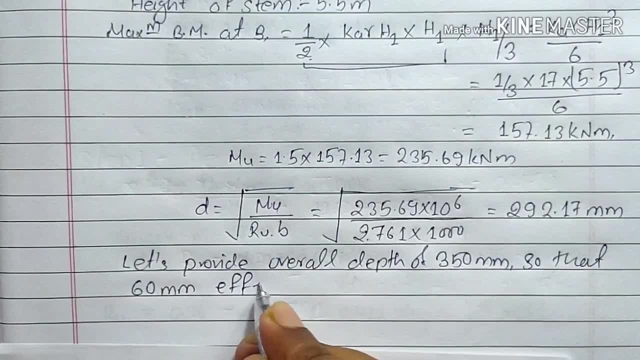 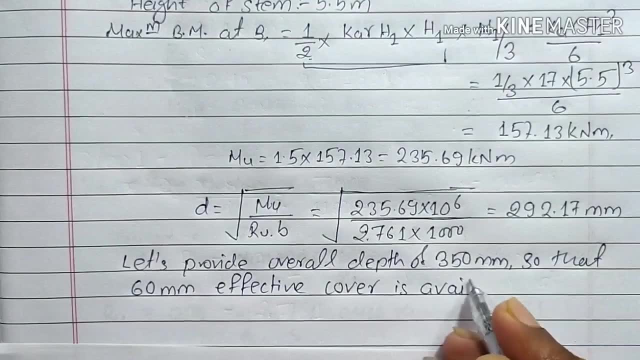 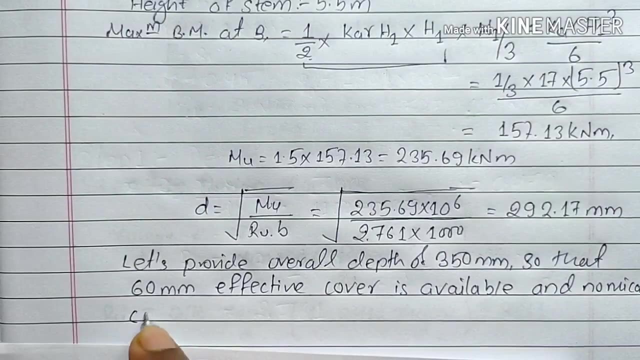 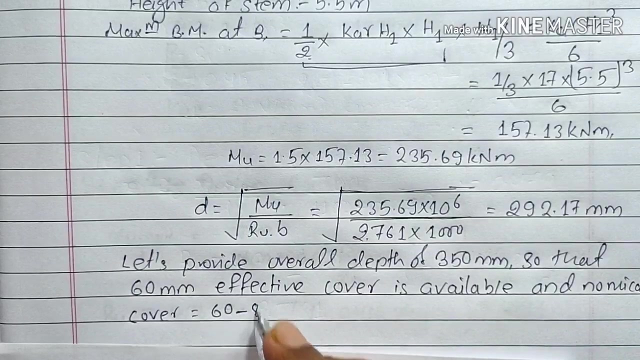 millimeter effective. effective cover is available and nominal cover equals to 60 minus 8 means we are providing 60 millimeter dia bar, and this is D by 2 actually. so this is going to be 52 millimeter using 16 mm dia bar. 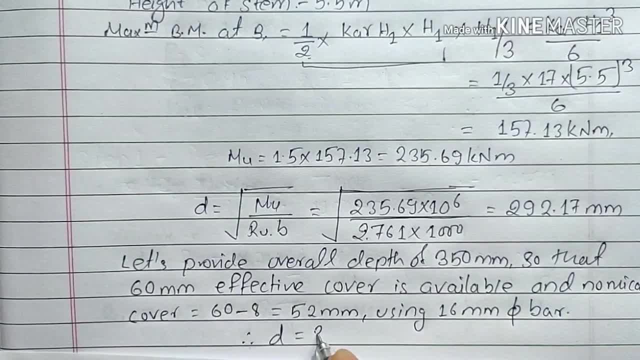 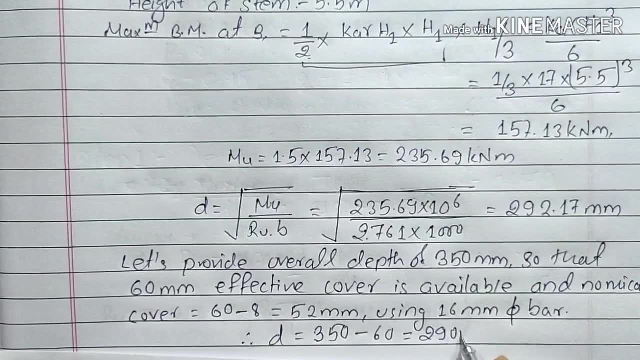 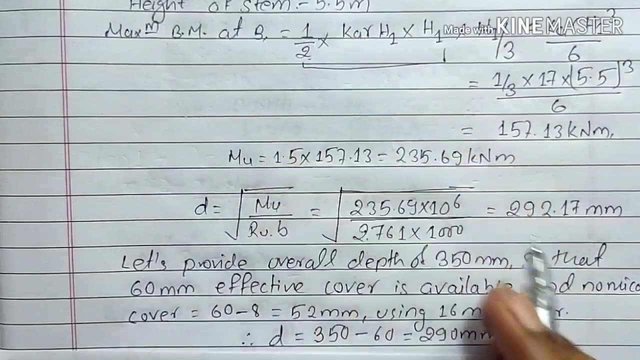 so, therefore, we will have effective depth equals to 350, which is our overall depth, minus nominal cover 60, which is going to be 290 mm. now let's move towards step 4, and later we will design the reinforcement of the steam. so let's move towards step 4 now. 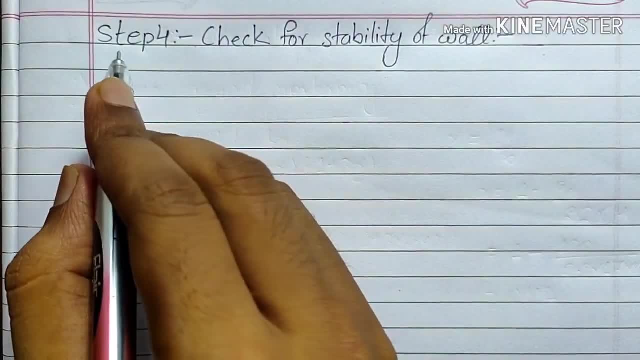 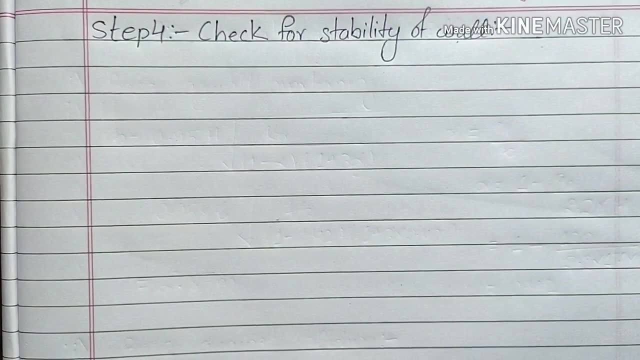 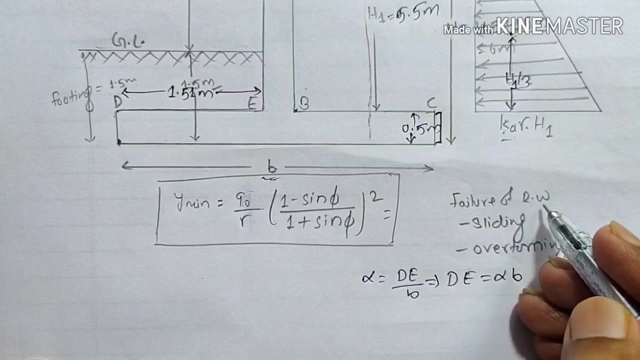 now here our step 4 is going to be check for the stability of wall. here, in this step, we will check whether our retaining wall is stable against sliding and overturning or not. here, as i told you that the failure of retaining wall mainly occurs either by sliding or by overturning, 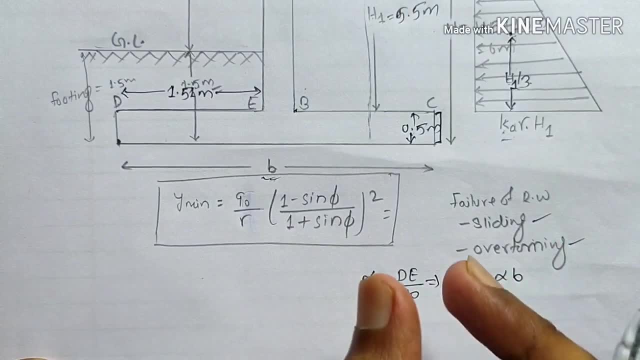 so in this step, we will check that the dimension which we have chosen for our retaining wall is suitable or not. that is protecting our retaining wall. so we will check whether our retaining wall is stable or not against sliding and overturning or not. so let's see how this is done. 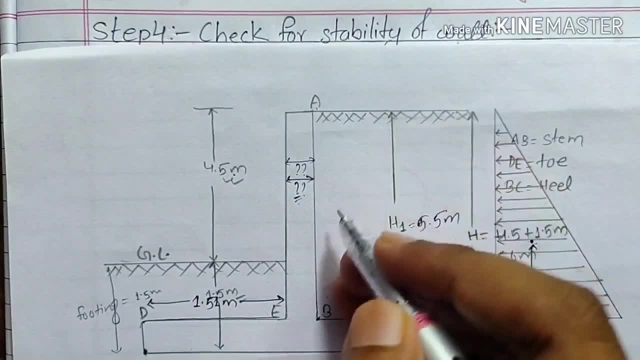 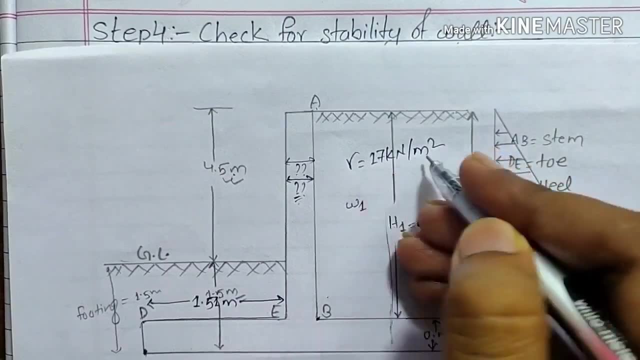 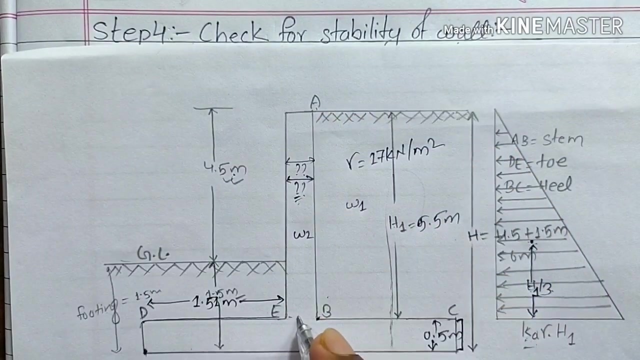 now, let the weight of this soil portion be w1 and its unit weight gamma equals to 17 kilo newton per meter square, which is given, and let the weight of this steam be w2 and let the weight of this w3, and we have come to know that the span 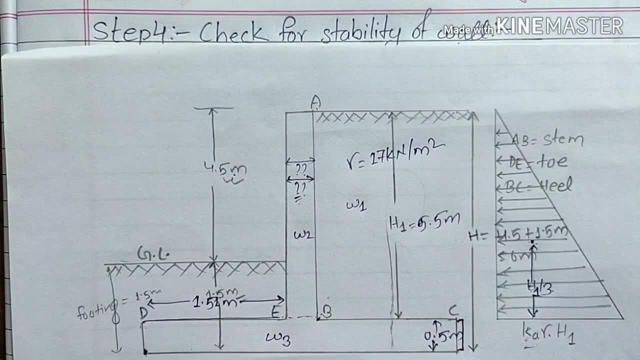 we have calculated the span be, which was 350 millimeter, means 0.3 meter, and we know that the b equals to 3.6 meter, which we have calculated in second step, and subtract, subtract 1.5, 1 and 0.35 from from 3.6, then we will get: 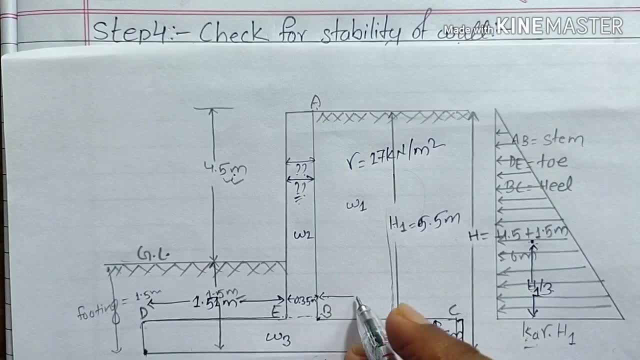 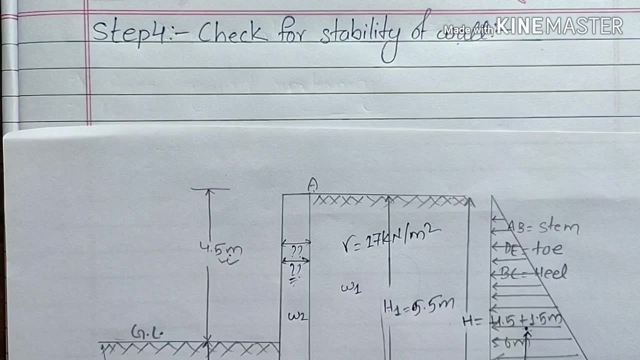 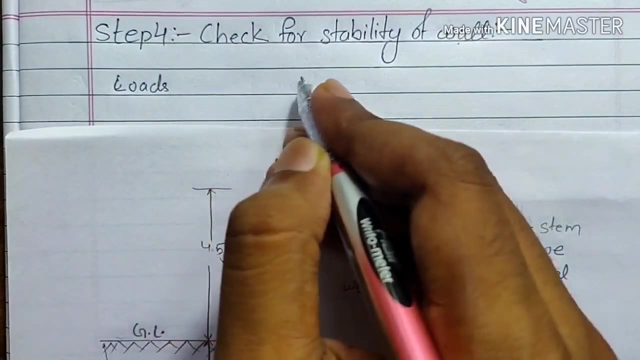 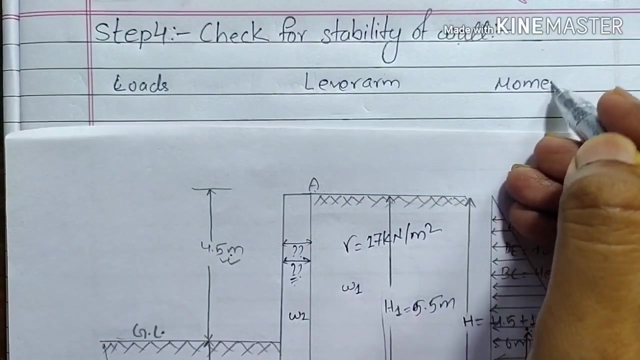 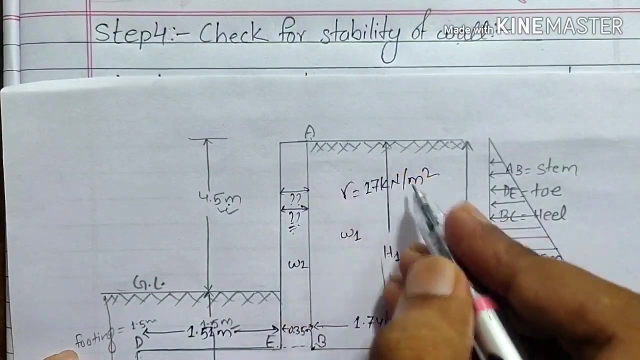 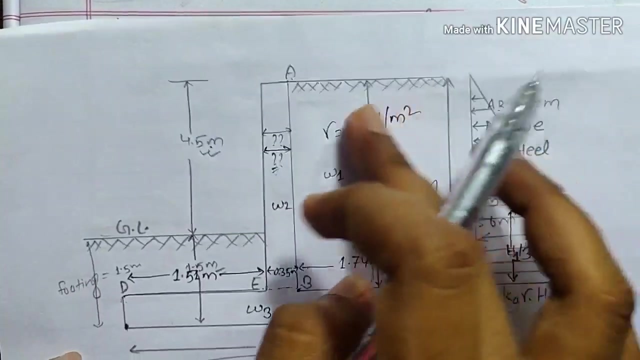 the value of span B BC, which will be equals to 1.74 meter. now let us draw a die, a table mentioning loads, lever, arm and moment. and for load, as we have assumed that the load of, we have denoted the load of soil as w1, so load w1 is equals to. this is rectangular. 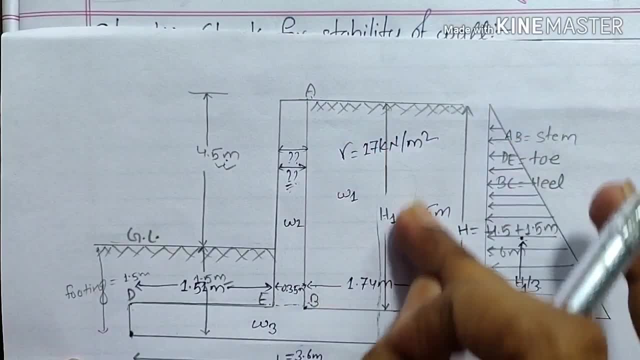 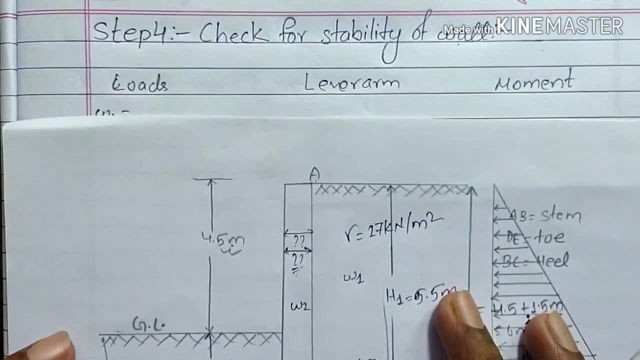 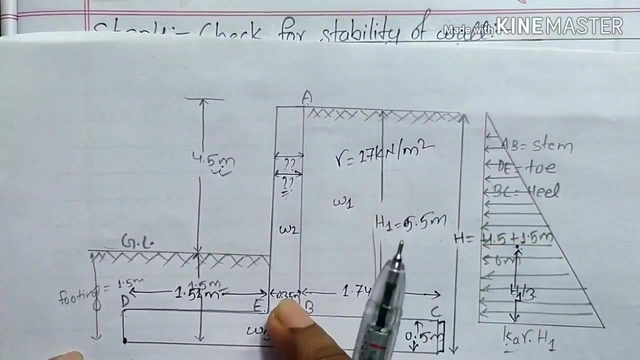 portion. so we need to multiply the area of rectangle into the unit weight of soil, which is 17 kilo Newton per meter square, to get the weight of soil. then we will have here 1.74 into height of soil. height of soil is height from this. bottom portion up to here we have the bottom channel. then we have the bottom channel, the bottom plate, which is the smaller part. now it is going to be 1.74 into height of soil, height from this bottom portion up to here. we will have here 1.74 into height of soil. height of soil is height from this bottom center up to here. sh мне câlSTEAM. 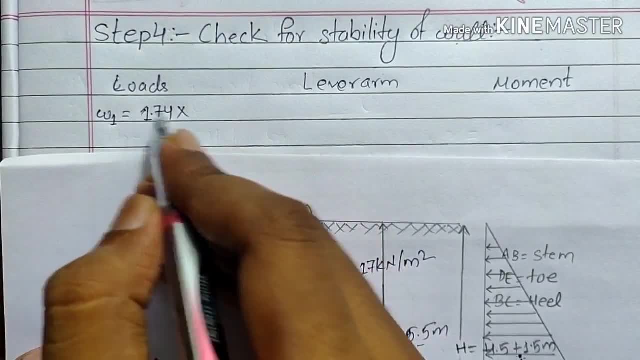 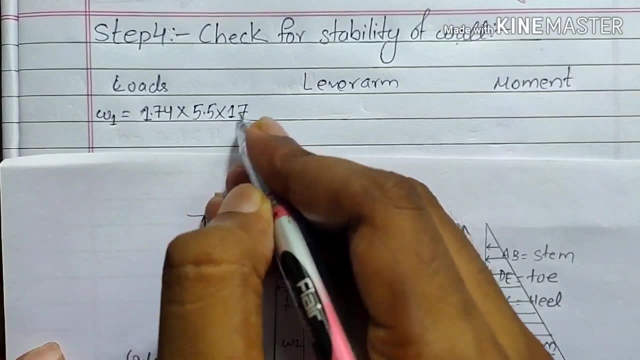 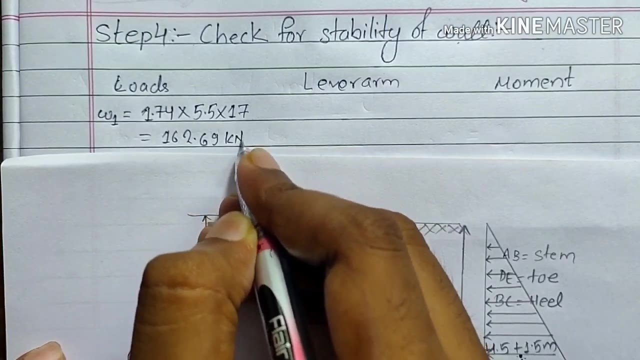 is our 5.5 meter. so multiply this 1.74 by 5.5 meter into unit weight of soil is 17, so we will get w1 equals to 162.69 kilo newton per meter. now time for lever arm. lever arm is actually the 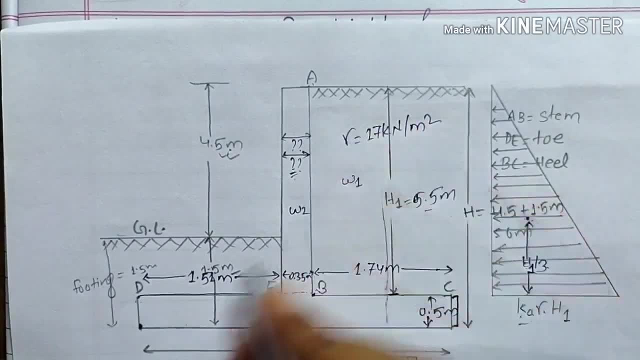 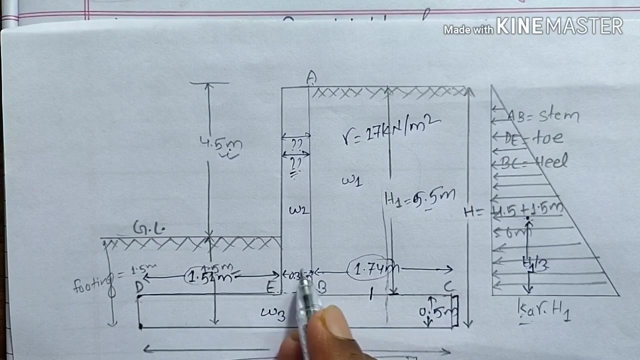 distance of the cg- cg of the soil from the point d. now the cg will be acts as the center of 1.74 meter. so from d, from the point d, the cg will be equals to 1.51 plus 0.35 plus 1.74 divided by 2. 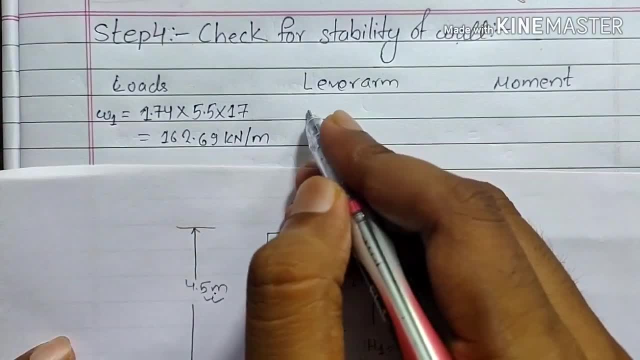 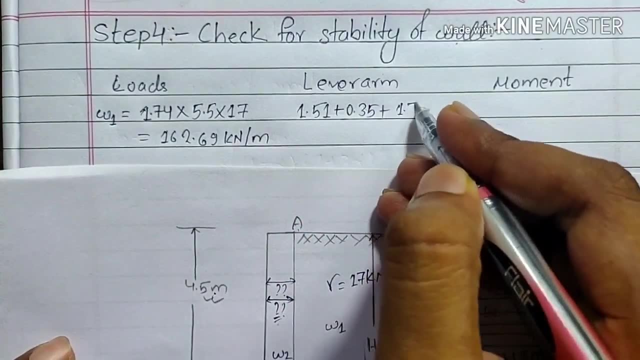 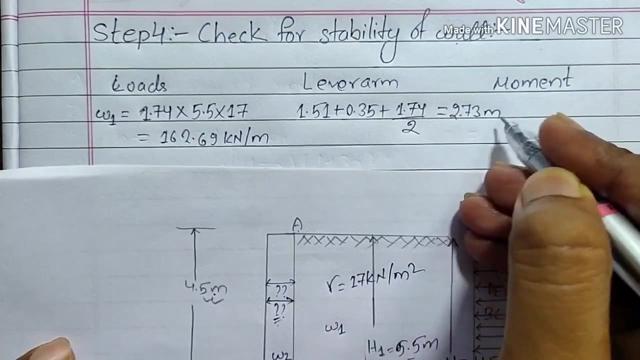 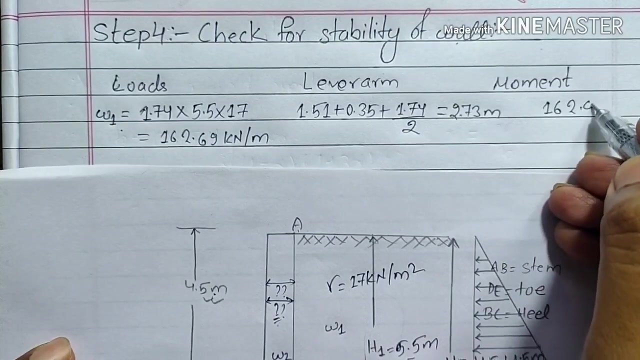 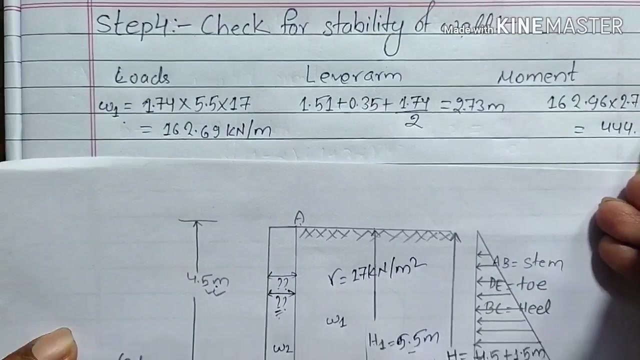 what i said. cg of w1 will be 1.51 plus 0.35 plus 1.74 divided by 2, which will be equals to 2.73 meter. now, for moment, multiply w1 into lever arm, then we will get 162.69 into 2.73, which will be equals to 444.14 kilo newton meter. similarly, 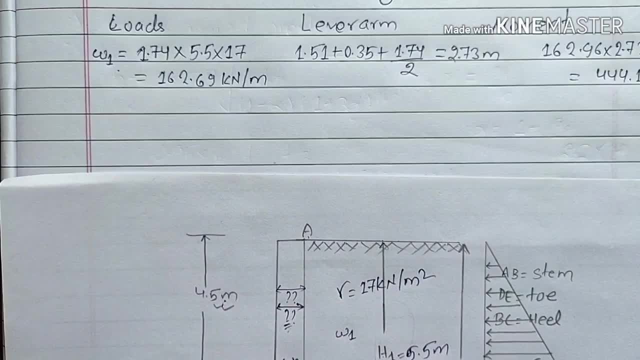 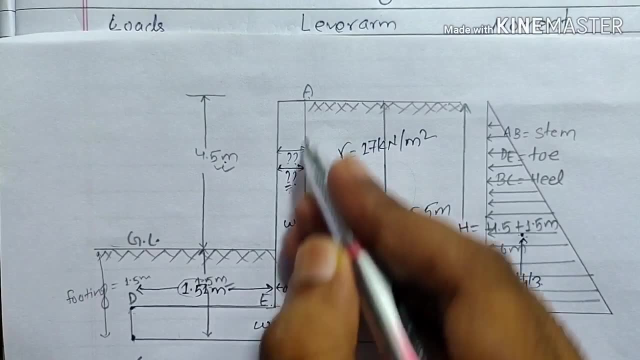 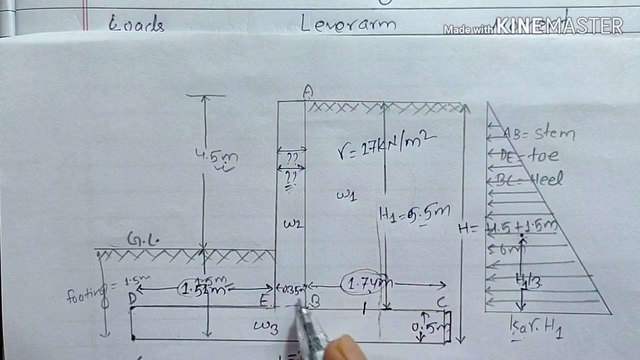 let's find do for load w2 here. for w2, what we need to do is, again, this is rectangle, so multiply base into height and then multiply this by your the unit weight of concrete, because we are using concrete for making the retaining wall. it was soil, and these two w in w2 and w3, we will be using the unit weight. 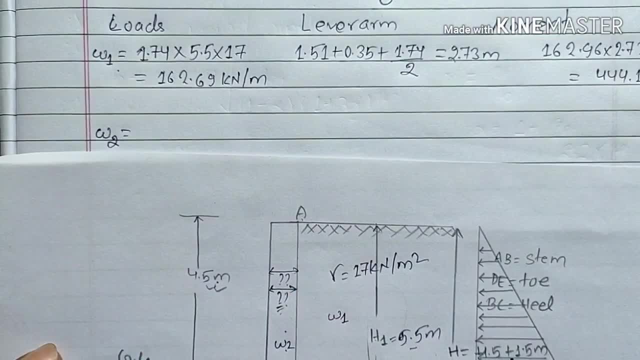 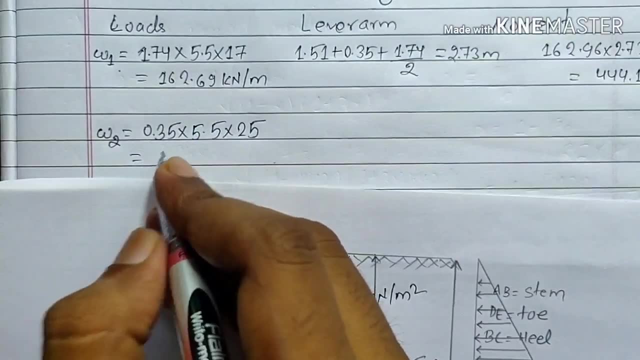 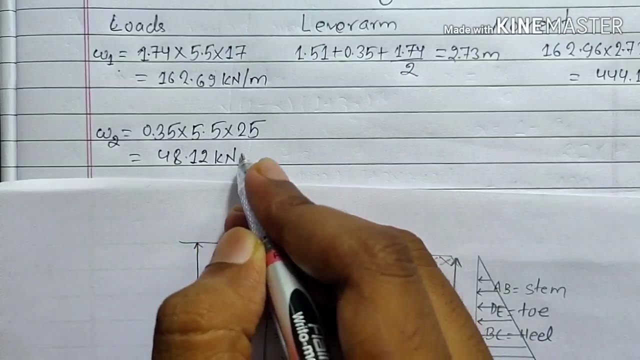 of soil newton per meter square. so do this. we have w2 equals to 0.35 into height is 5.5 meter, and so we will get w2 equals to 48.12 kilo newton per meter, and the lever arm. 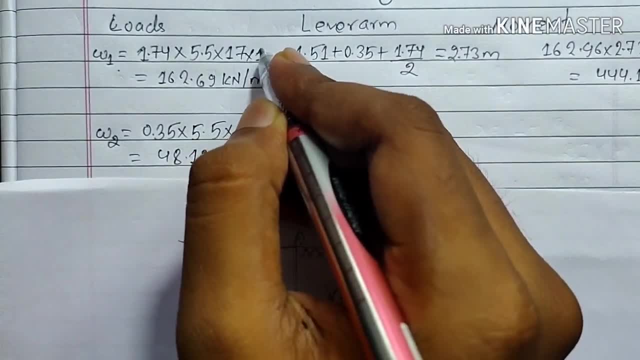 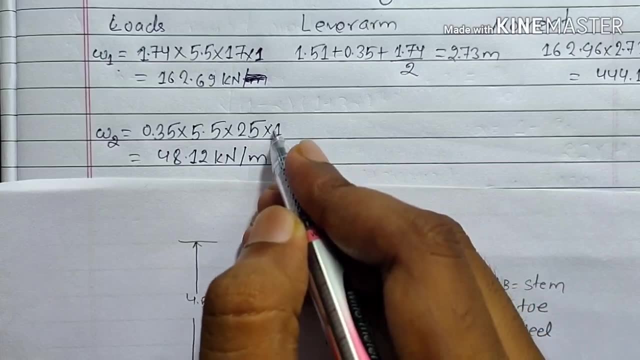 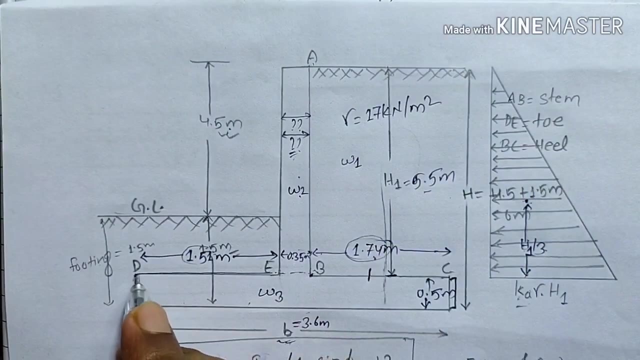 one thing here i am taking for unit length. so multiply this for one meter so we will get this in kilo newton. only multiply this per meter length, so we will get it in kilo newton. now again, the the lever arm means we need to find the distance, take the distance up to the cg of this. so here 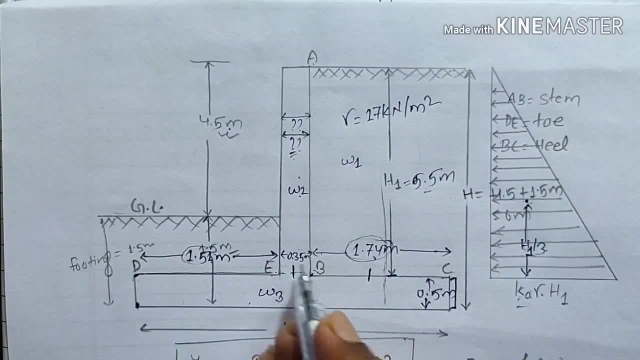 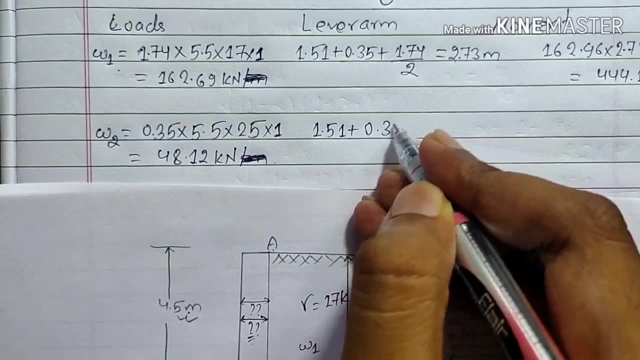 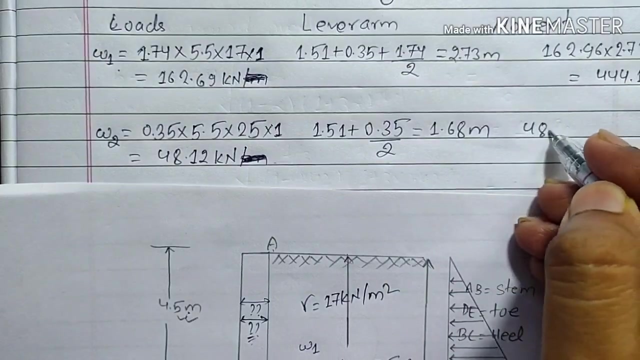 the cg of this rectangular portion will be 1.51 plus 0.35 divide by 2. so write it down here: 1.51 plus 0.35 divide by 2.68 meter. now for moment, multiply this 48.12 into 1.68, we will get. 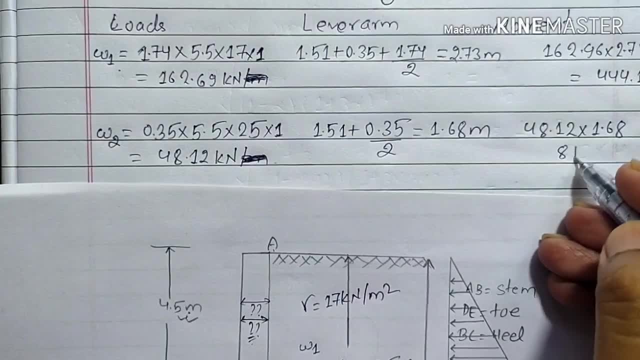 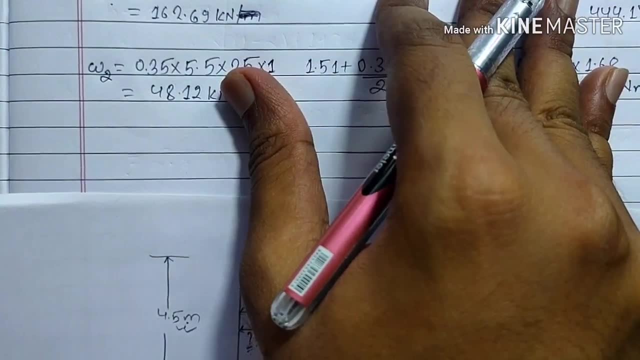 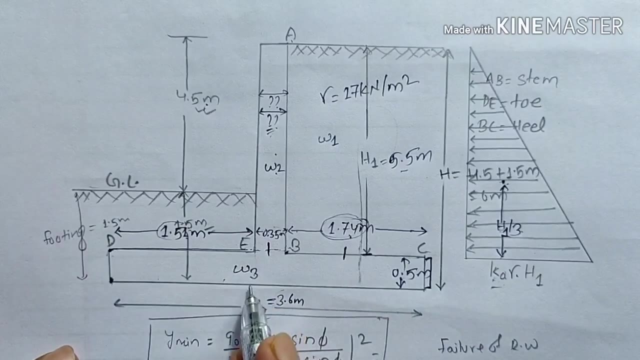 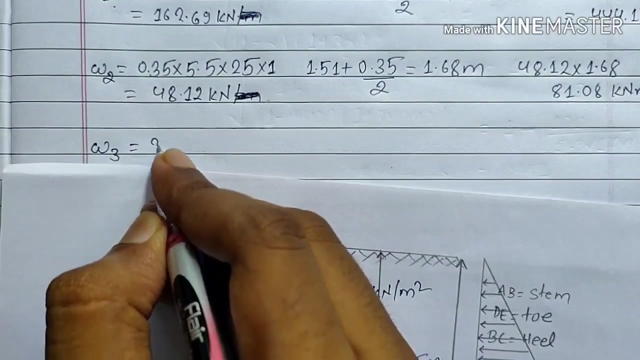 moment equal to 81.08 kilonewton meter. similarly, time for w3 and for w3 we have: w3 is the weight of the base slab, which is w3 means again this is rectangular portion. so multiply base into height, then we will do here 3.6 into 0.5, into unit weight of concrete 25. 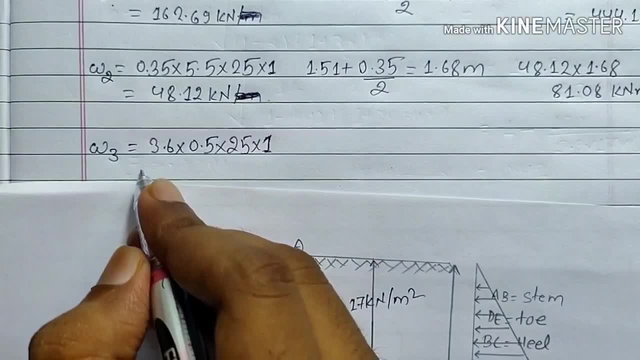 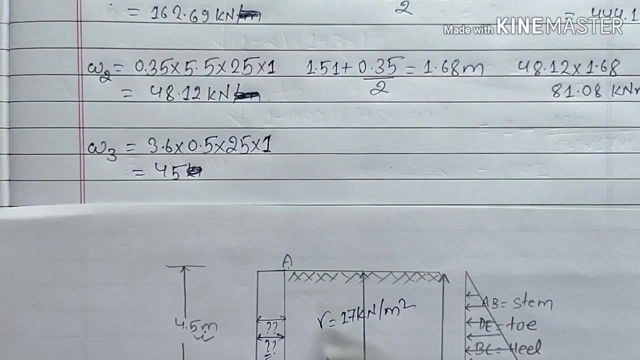 and we will do here 3.6 into 0.5 into unit weight of concrete 25, and we will do here 3.6 into 0.5 into unit weight of concrete 25 for one meter length, into one which will be equals to 45 kilo newt, sorry, 45. 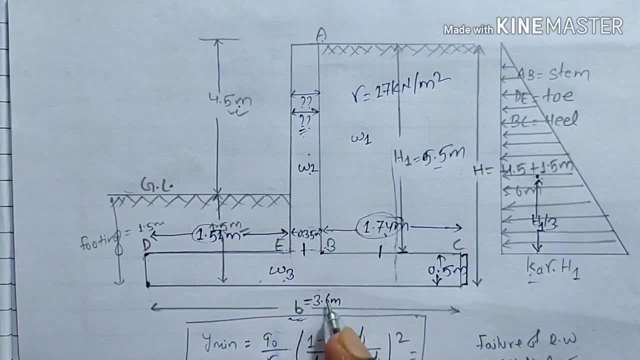 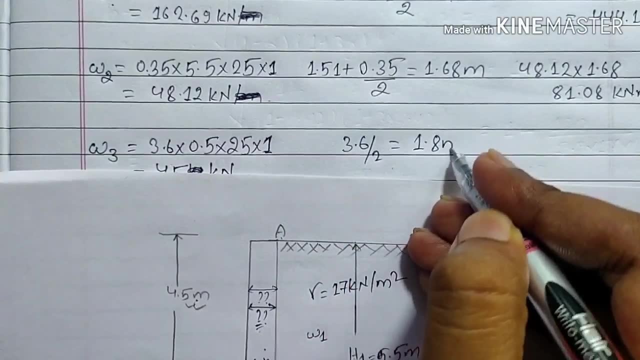 kilo Newton and the lever arm is going to be half of 3.6 meter, so it will be 3.6 divided by 2 equals to 1.8 meter. now, for moment, multiply 45 into 1.8, 45 into. 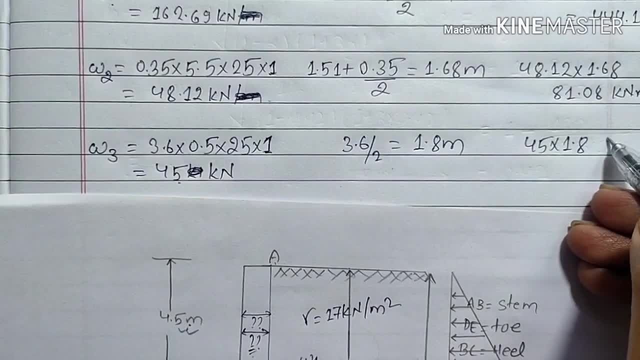 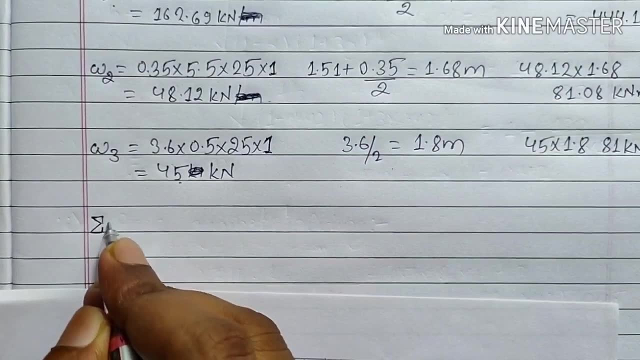 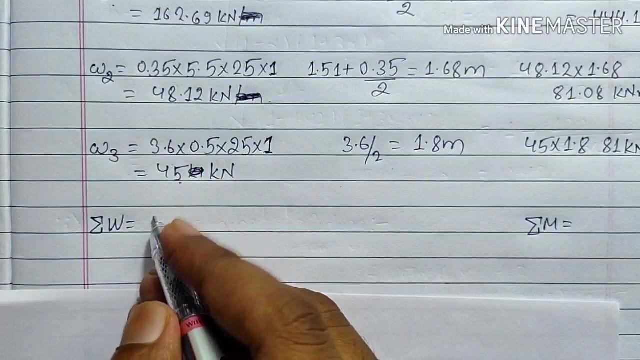 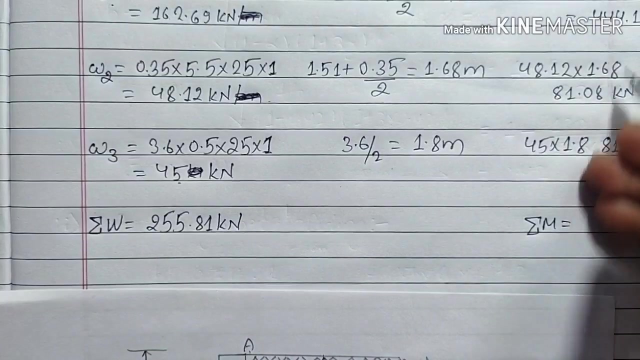 1.8, we will get moment equals to 81 kilo Newton meter. now take the sum of overall load and the sum of overall moment at these all we will get summation W equals to 255.81 kilo Newton, and sum of moment means this plus this. 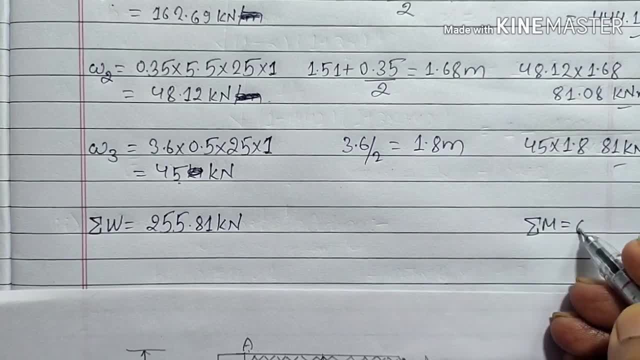 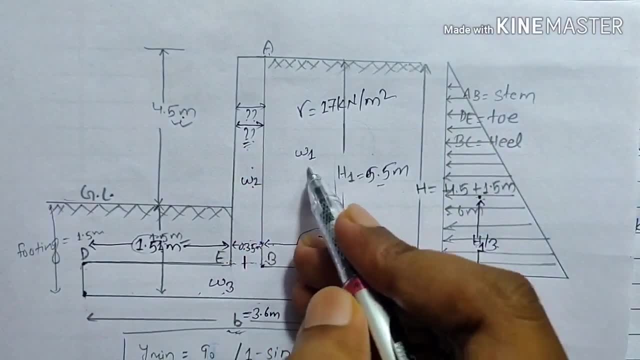 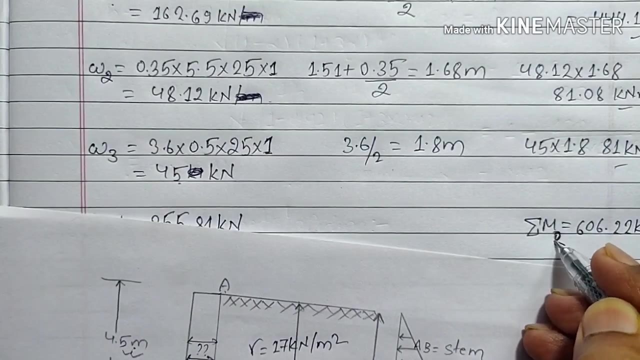 plus this, we will get sum of moment equals to 600, 6.22 kilonewton meter, as we all know that w1, w2, w3 are acting downward. so this is going to be our resisting moment, which will be denoted by mr. also, this is a sum of moment, which is also 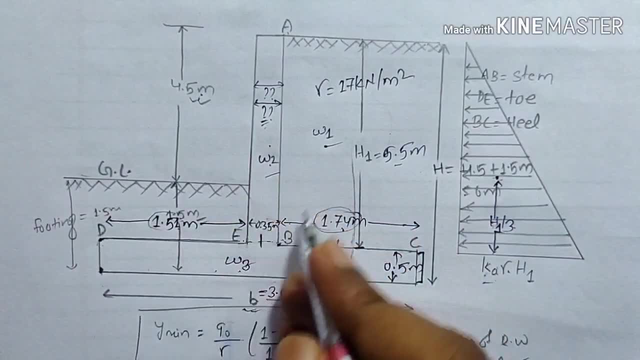 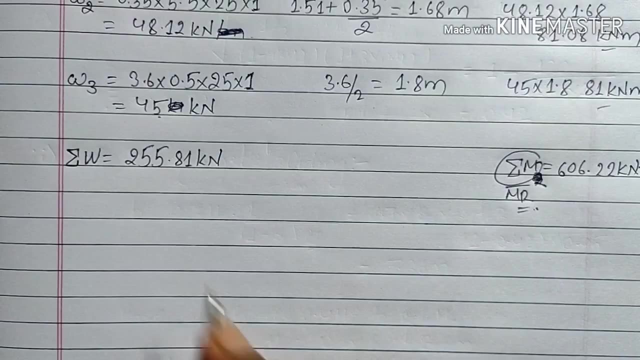 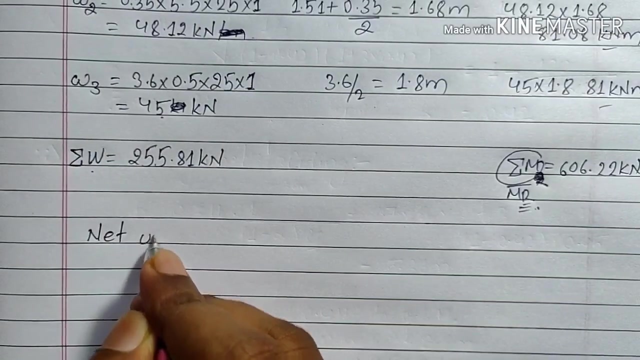 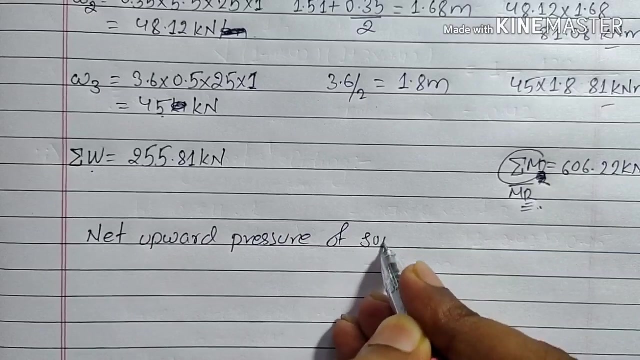 our resisting moment, because all these moments on and the load are acting in downward direction. so this is going to be our resisting moment. now, after finding summation w and the resisting moment, let's find out the upward pressure of the soil. so net upward pressure of soil. 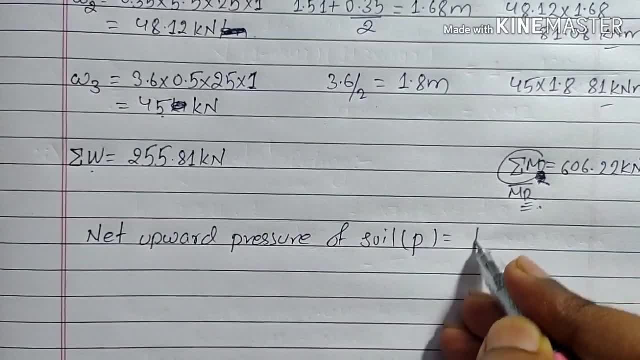 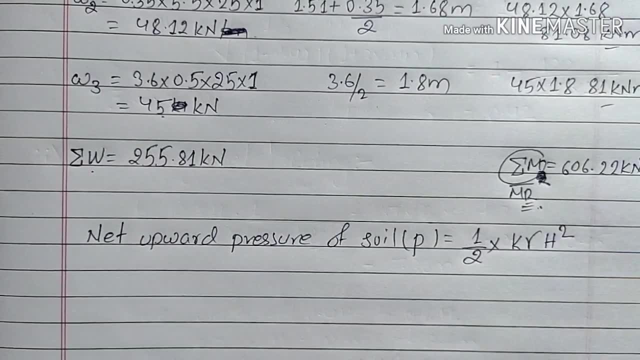 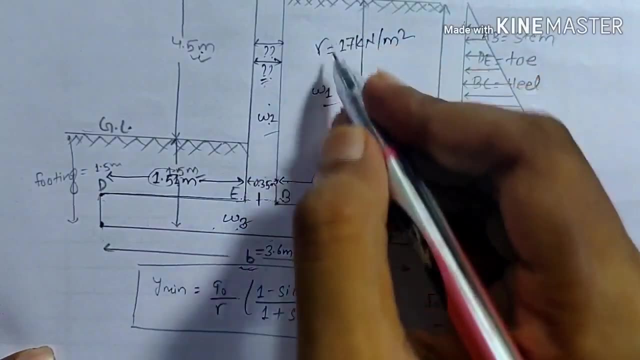 which is denoted by p equals to 1 by 2 into k a gamma h square. this is because this is denoted by p equals to 1 by 2 into k a gamma h square. this is because, see here, this was the pressure exerted by this soil portion and the soil which is bought below. 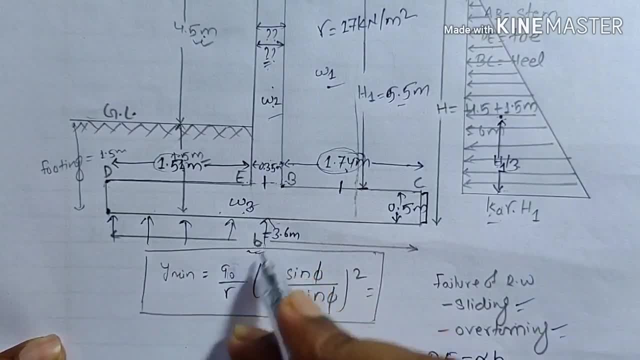 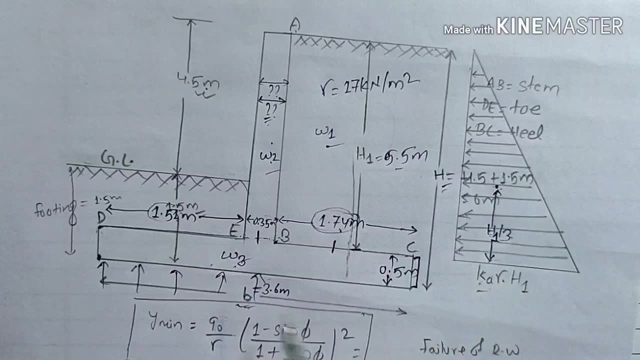 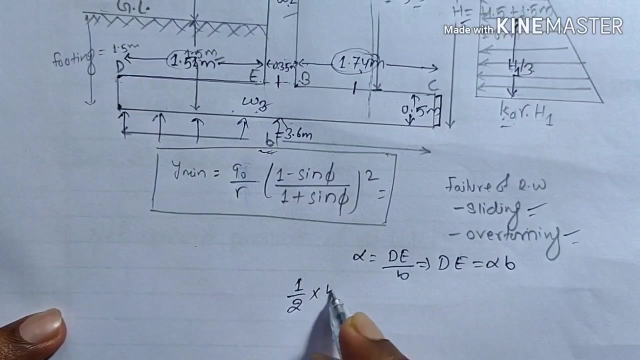 the retaining wall is also exerting some pressure which is acting in upward direction, and it is. we need to take the height of whole retaining wall which is at. then again it will create a triangle and then we will have the formula half into base into height, so it will be half into 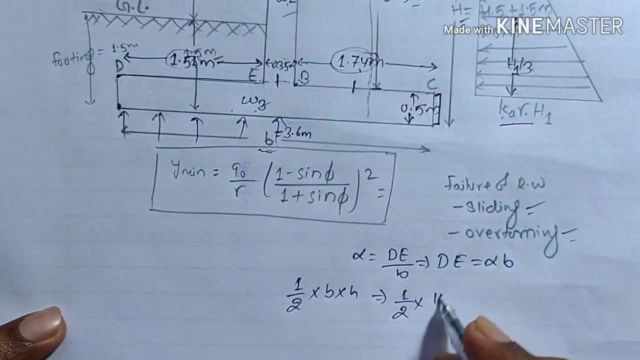 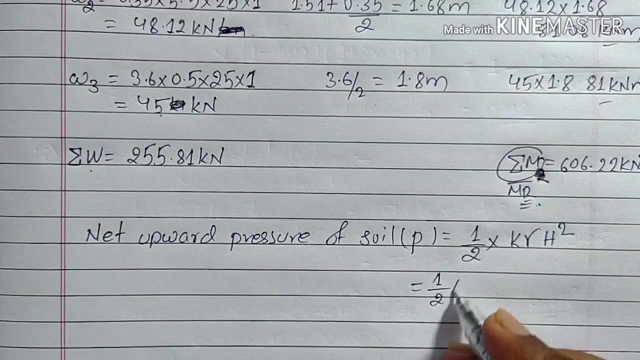 base means k a gamma h into height means whole height. so it will be equals to k a gamma h square by 2. so I have used this formula here. and on putting the value 1 by 2 into k a means coefficient of active earth pressure is 1 by 3 into gamma x: 17. 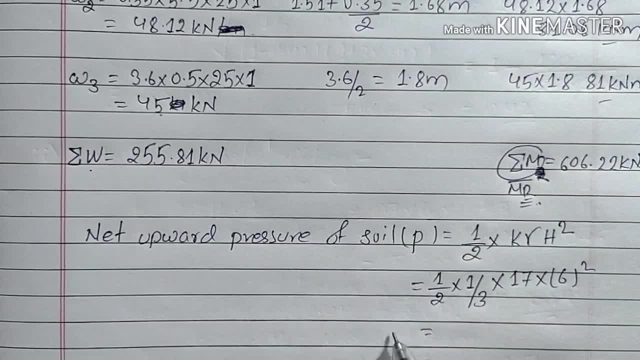 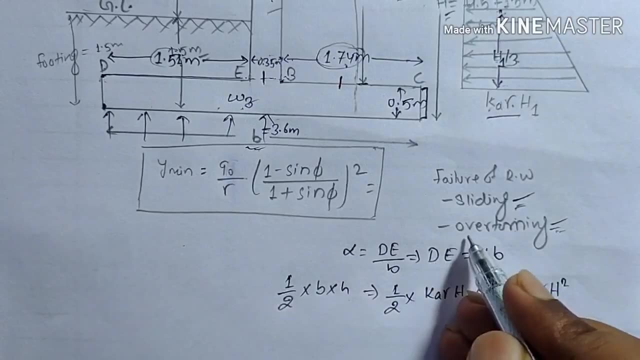 into height is 6 is squared, we will find the net upward pressure p equals to 100. Now, as I told you that the retaining wall will fail in either by sliding or overturning. So factor of safety against overturning should be greater than 2 and the factor of safety 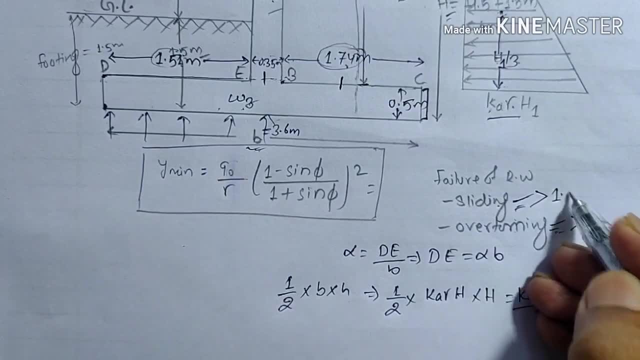 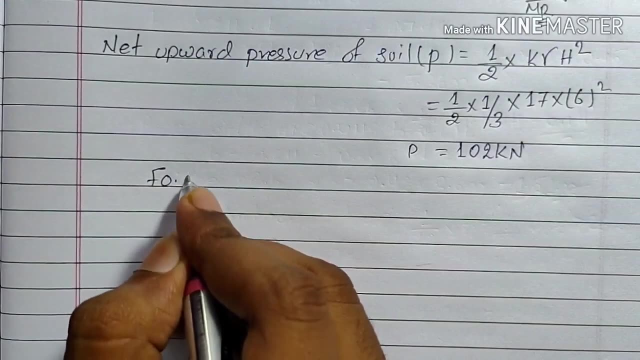 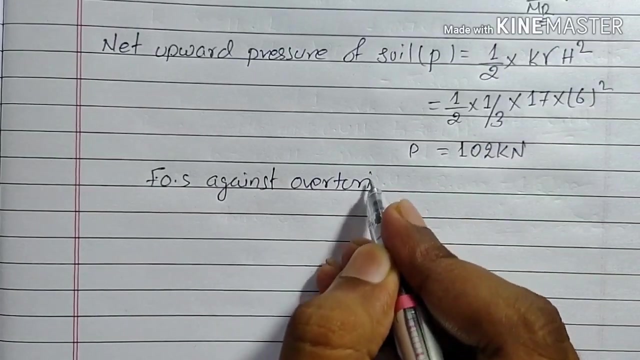 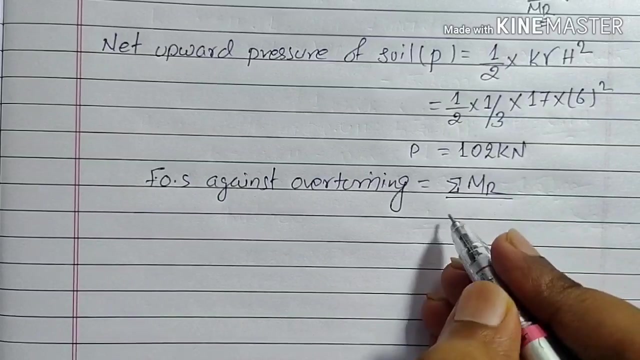 against sliding will be greater than 1.5.. So let's find out the factor of safety against overturning. So here, factor of safety against overturning. It is given by summation: MR means resisting moment. by summation, MO means the moment exerted. 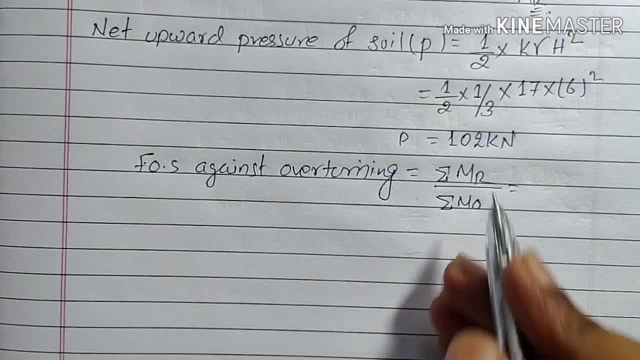 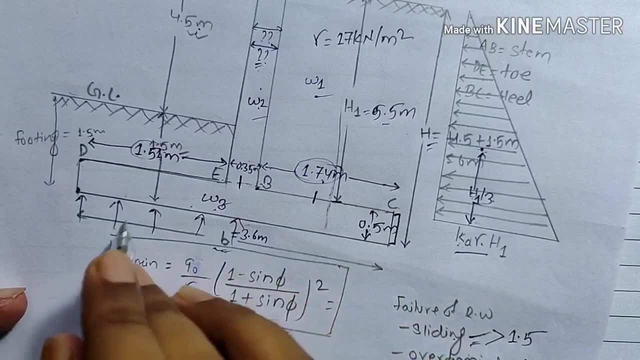 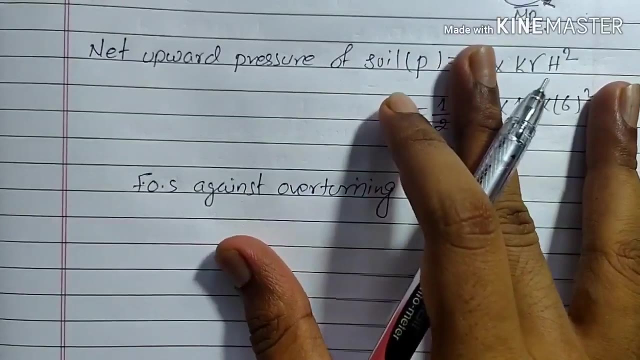 by the soil which is exerted from the bottom soil. This is MO. This is the moment exerted from the soil lying at the bottom of the retaining wall. So we have MR. MR is 600 here, MR is 606.22 kNm. 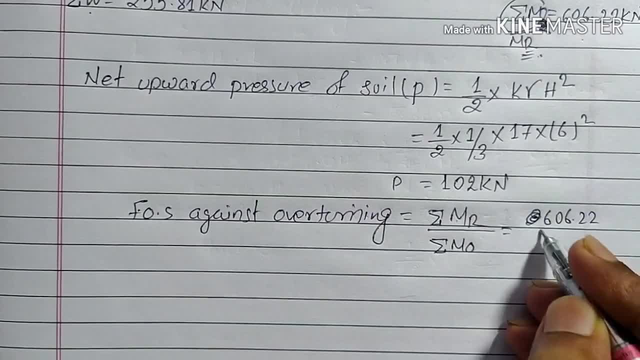 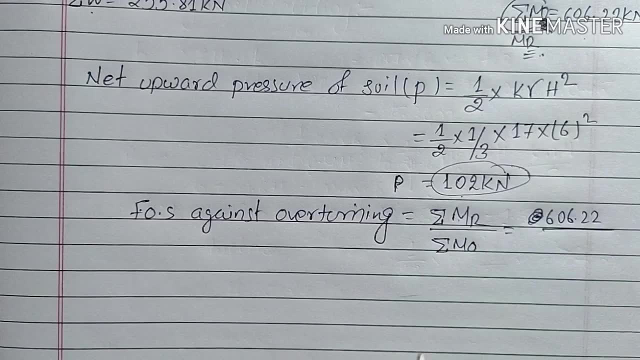 So write it down here: 606.22 kNm divided by MO. We have calculated the pressure. Now we need to multiply this by the distance up to the CG, Then we will get the moment. Then we will have MO equals 2.. 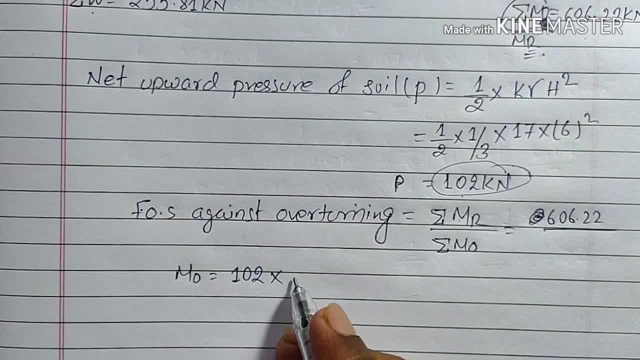 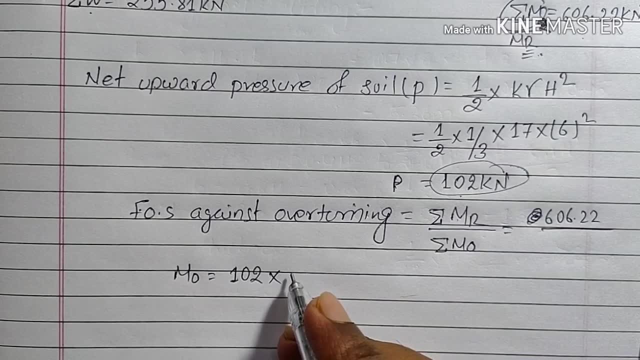 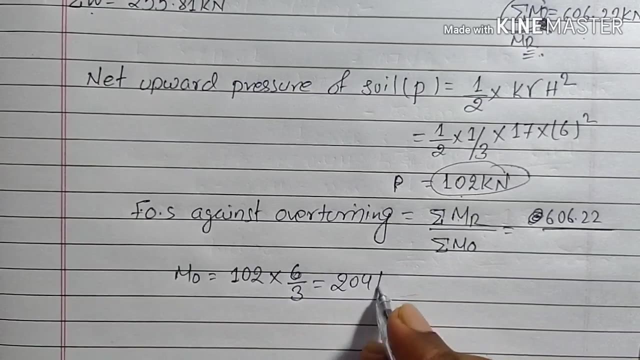 102, into which we will also again act at height: h by 3 into h by 3, and our h is 6 m. So divide this 6 by 3.. Then we will get this as 204 kNm. Now divide this by 204.. 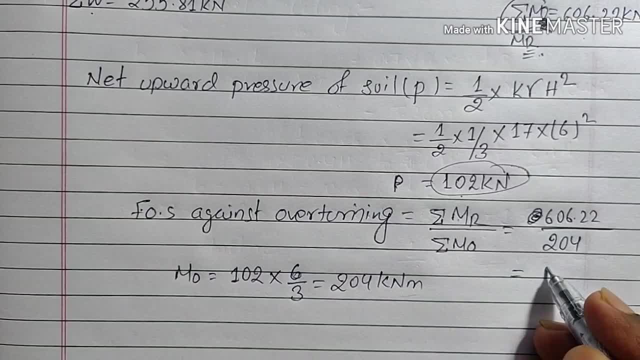 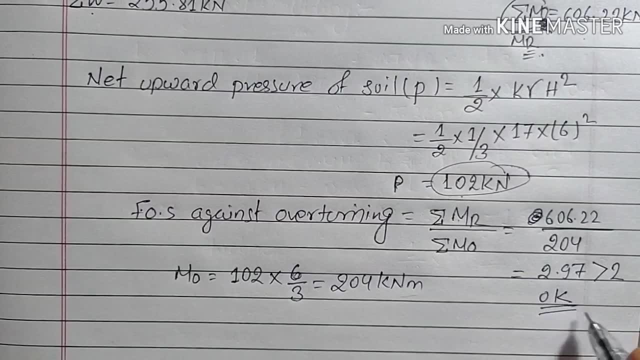 We will get factor of safety against overturning as 2.97.. Which is greater than 2.97. Which is greater than 2.97.. 2 means it is okay. Now time for the factor of safety against sliding. For that we have. 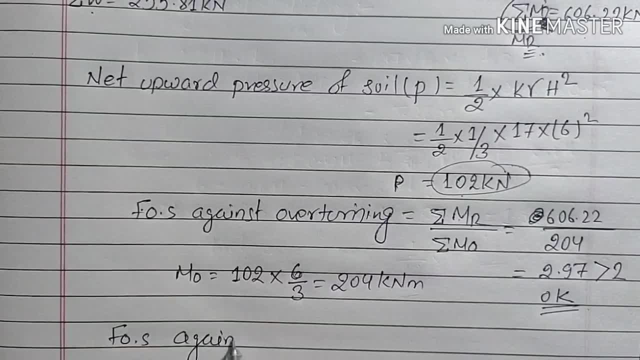 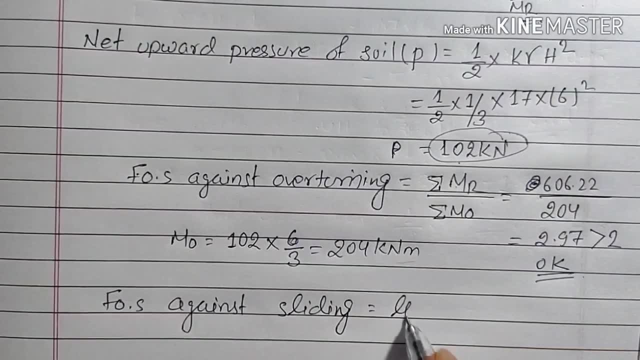 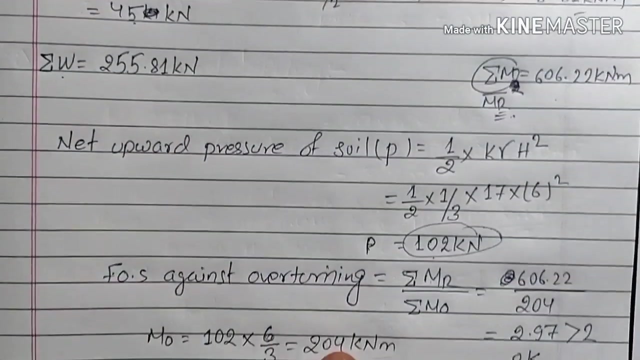 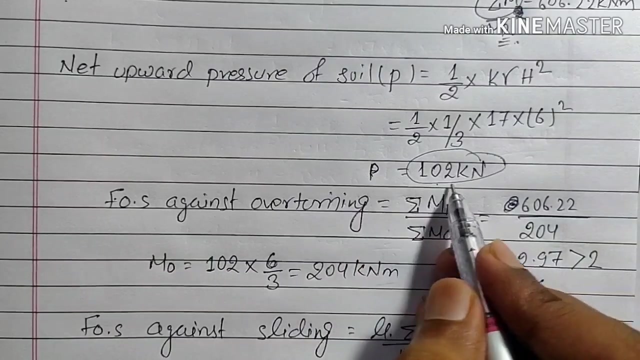 factor of safety against sliding equals to mu times summation w by p, and we have the value of mu as 0.45 into summation w and we have calculated the value of summation w as 255.81.. So write it down here: 255.81 divided by p and the p is 102 kN. So write it down. 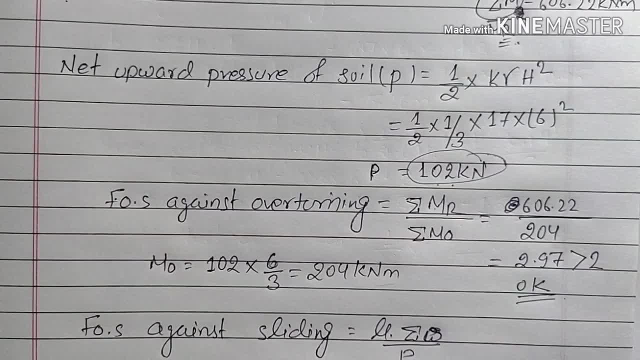 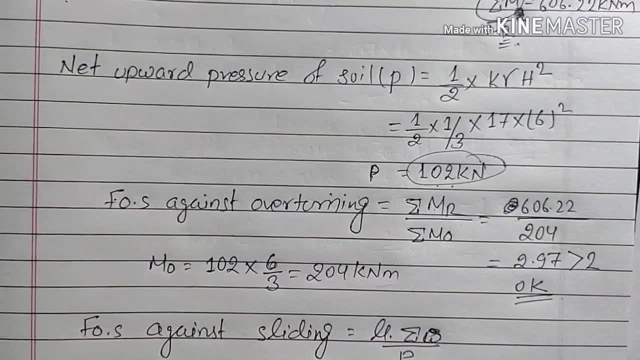 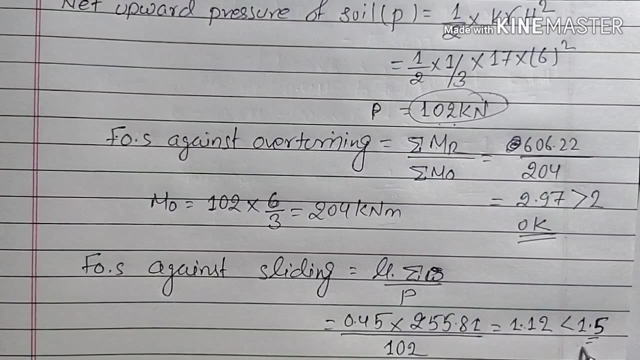 here 102.. We will get the factor of safety against sliding as 1.12 here, So as 1.12 is less than 1.5. Okay, Okay, Which is less than the minimum requirement of the factor of safety. See here, guys, It. 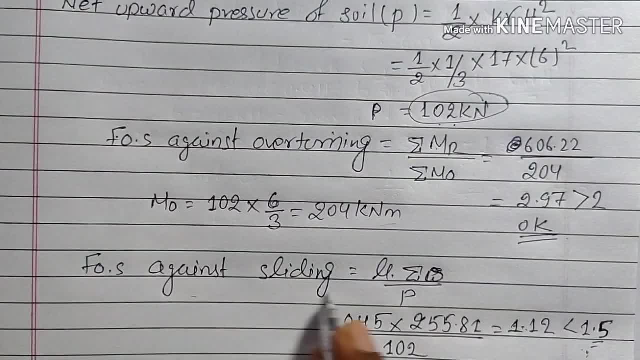 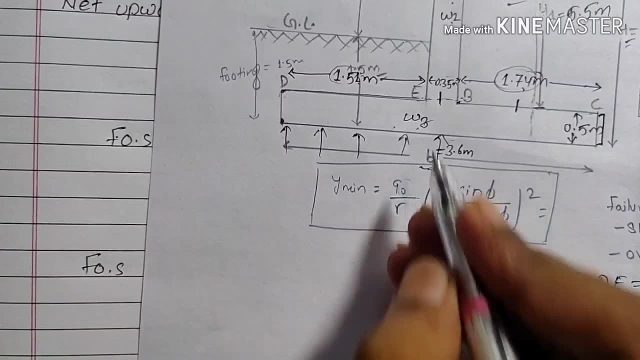 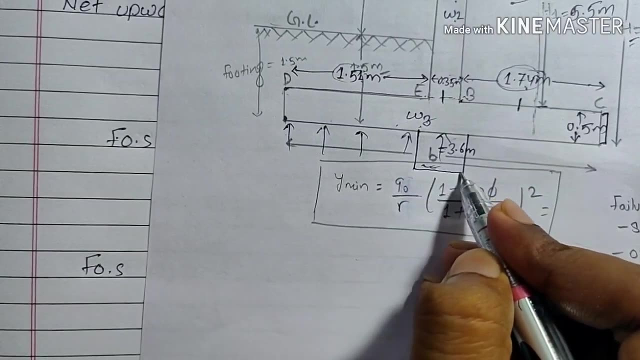 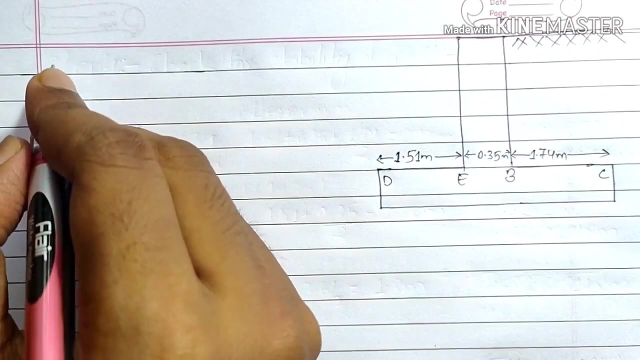 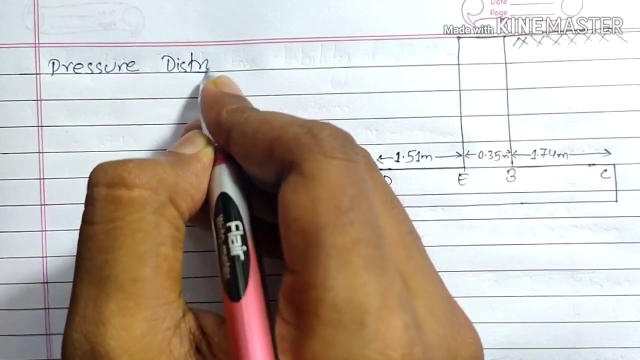 means our retaining wall is failing in sliding condition. So we need to provide a share key, and the share key will be provided here like this: We need to provide the share key to prevent our retaining wall from sliding. So here we will be finding the pressure distribution, Pressure. Pressure distribution and the pressure. 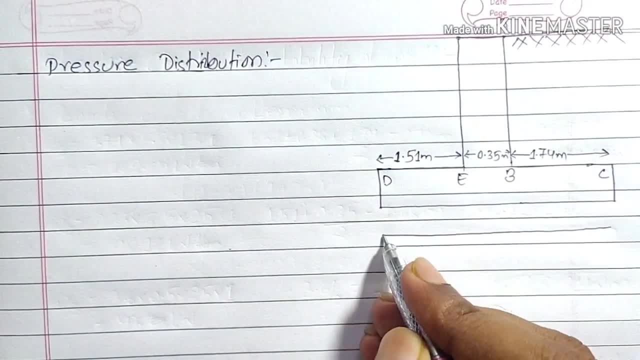 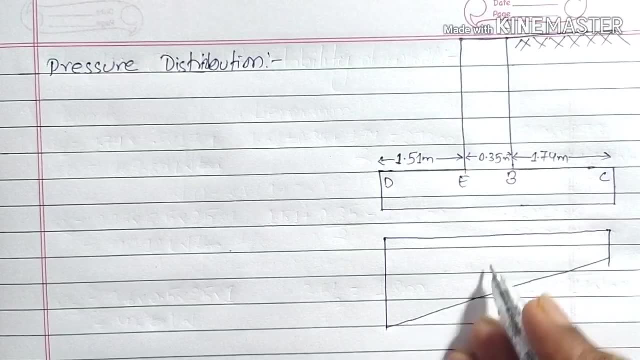 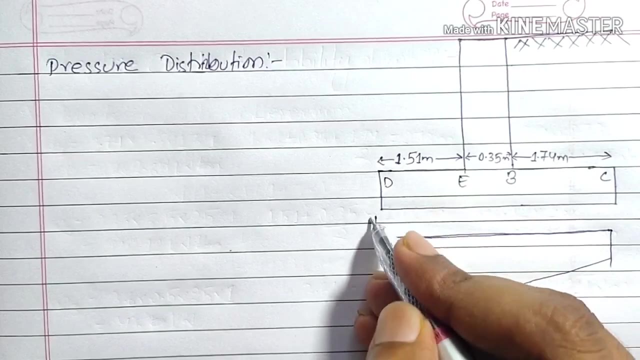 distribution in retaining wall is always in this pattern. This is upward soil pressure which is exerted by the soil on the retaining wall and which it is maximized. So this is maximum at toy portion. This is our toy, as I had already mentioned. let you know, while 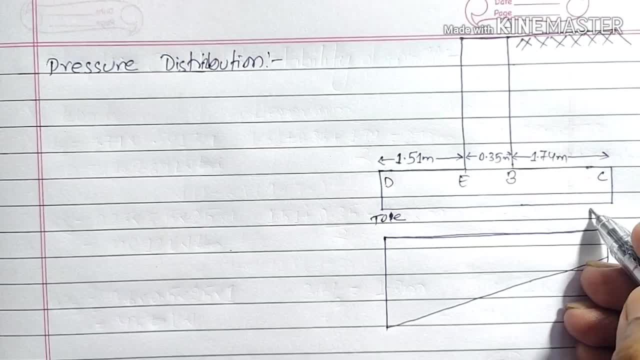 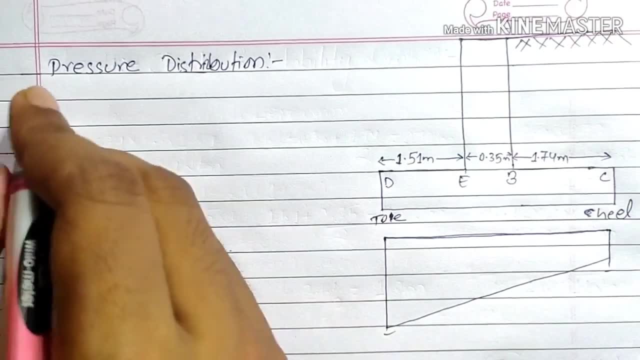 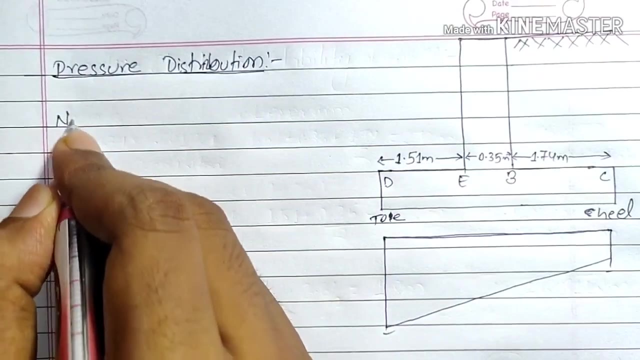 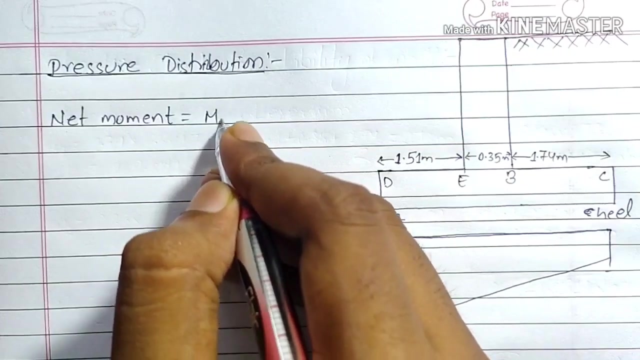 in the beginning of the video. and this is our hill, So let's find out the pressure distribution value here, and we have. we will begin taking the net moment. net moment. net moment is mentioned as a resisting, minor resisting moment, minus our turning moment and resisting moment. 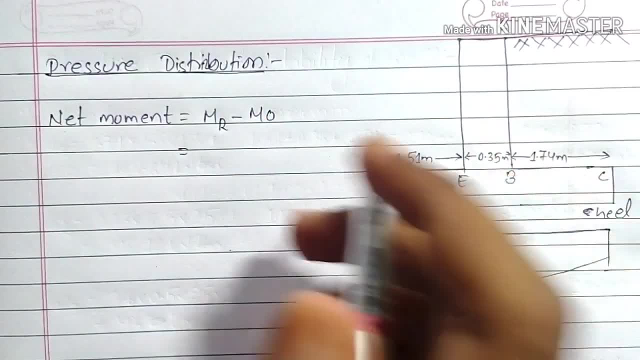 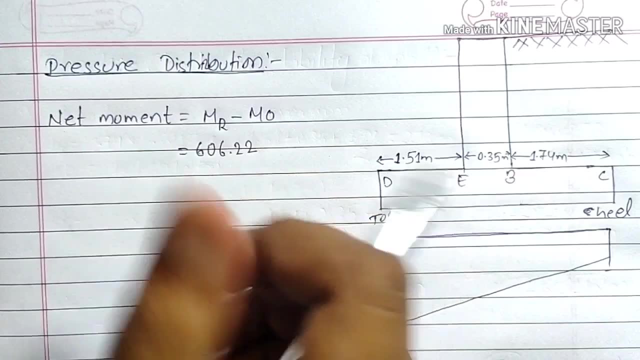 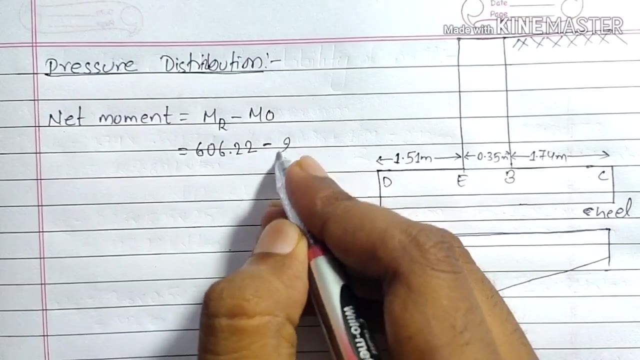 was the moment which was due to all the load acting downward and it was 606.22, which we have find out in the same step before this pressure distribution And our turning moment, which was 204 kilo Newton meter. and we have got net moment which is written as summation. 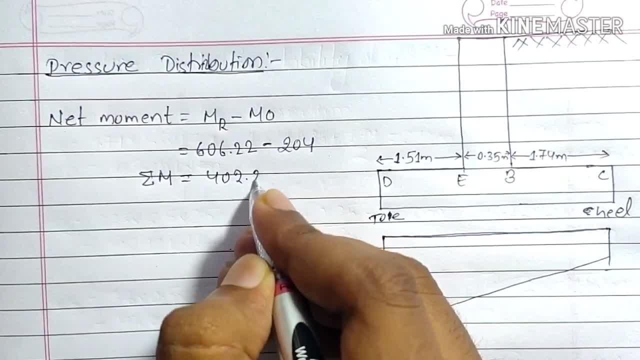 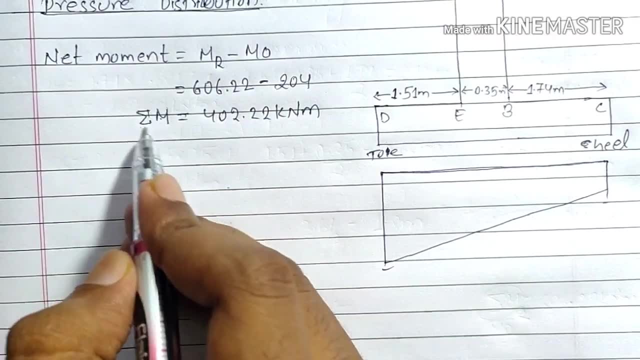 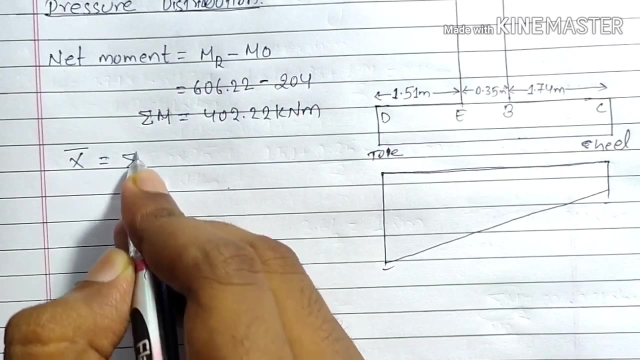 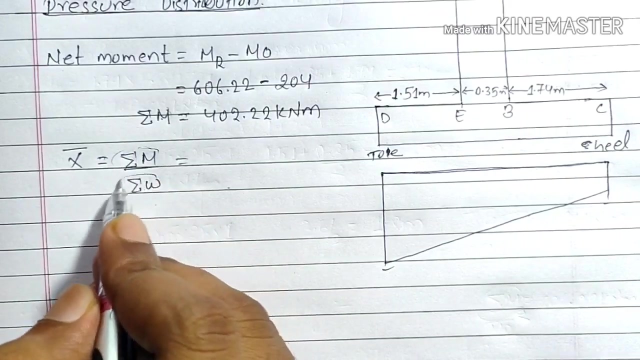 m equals to 402.22 kilonewton meter. Now let's find out the distance where this moment is acting. So this is acting as x bar, and which is written as x bar equals to summation m by summation w, because moment can be mentioned as weight into distance, and this is our resultant. 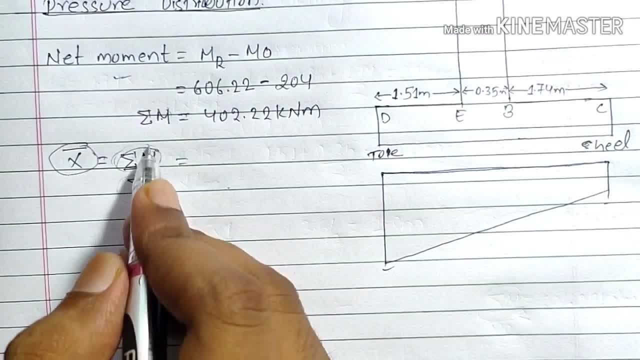 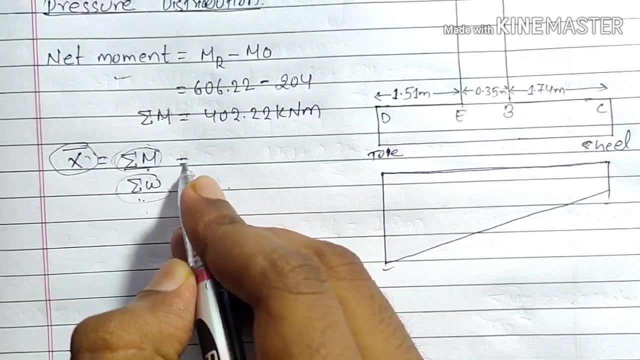 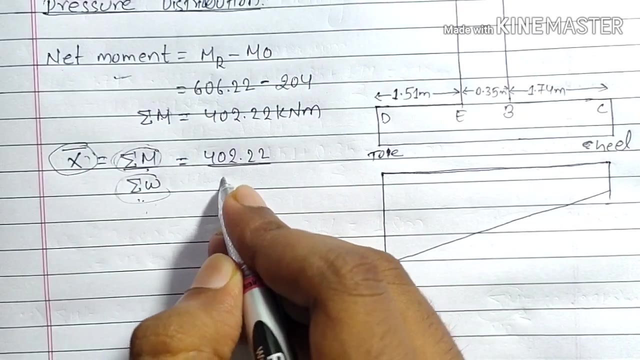 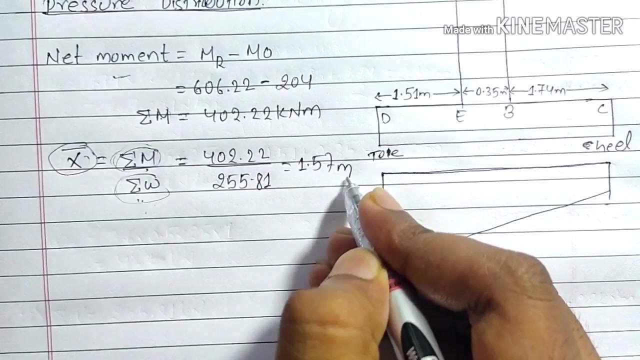 moment, which is also mentioned as net moment, which will be equals to the distance at which it is acting into total load acting in downward direction. So it will be: on putting the value, we will get 402.22 by 255.81 and it will be equals to 1.57 meter. Now let's find out. 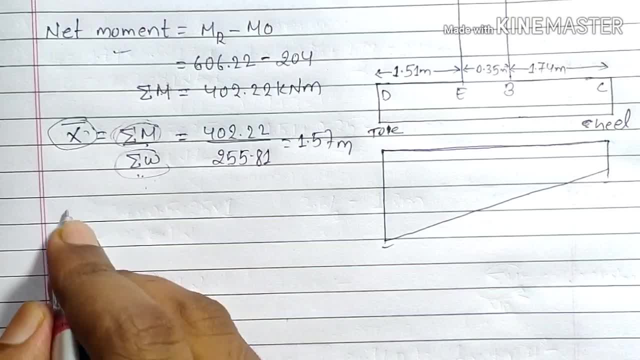 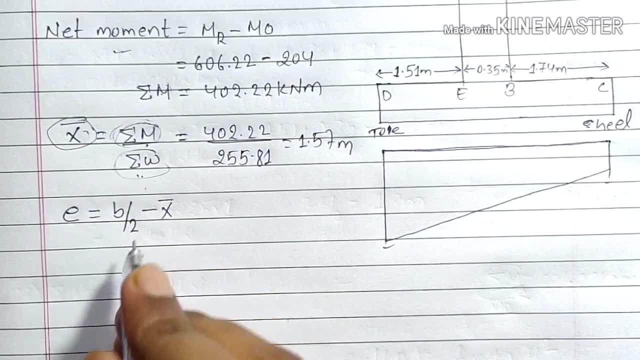 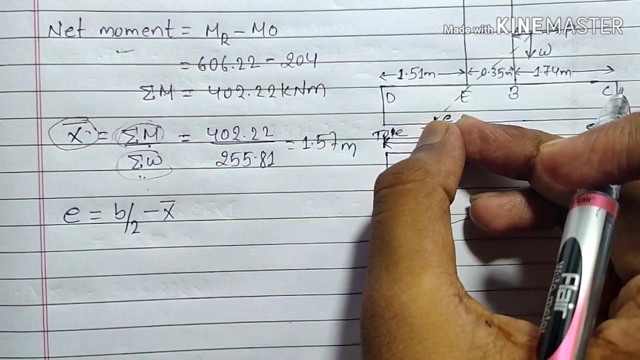 the eccentricity. And for finding out the eccentricity we have the formula. e equals to b by 2 minus x bar. Let me show you this in the diagram. So our this portion is b by 2 and this minus x bar, we will get the value of eccentricity. 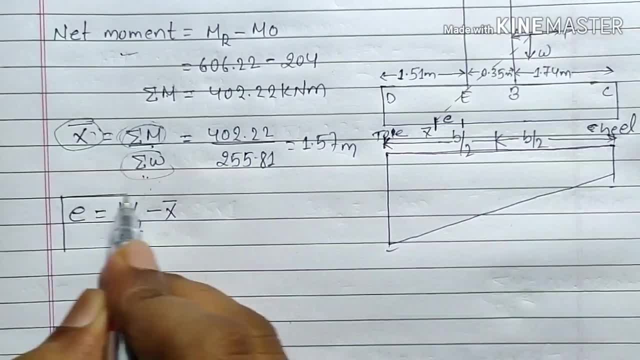 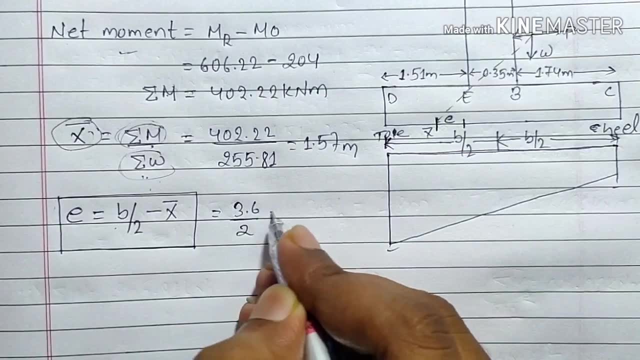 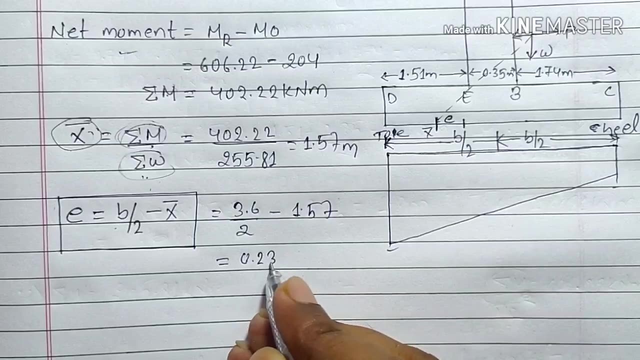 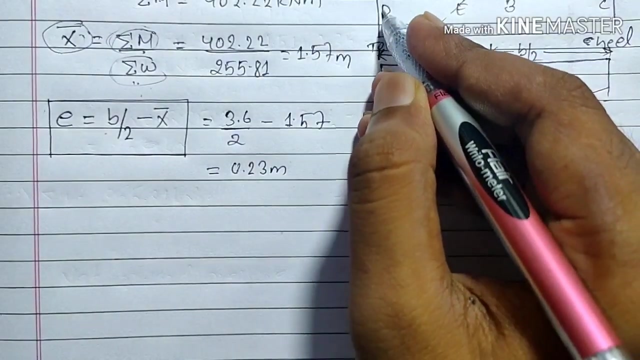 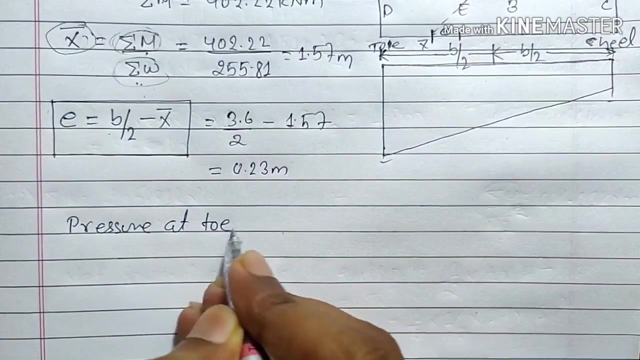 which is denoted by e. Just simply remember the formula and find out the value of eccentricity, which will be equals to 3.6 by 2 minus x bar is 1.57 and we will get the value of eccentricity as 0.23 meter. Now we need to find the pressure at this portion d. So pressure at toy is. 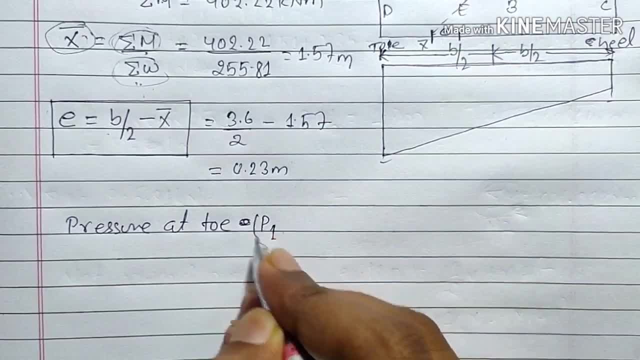 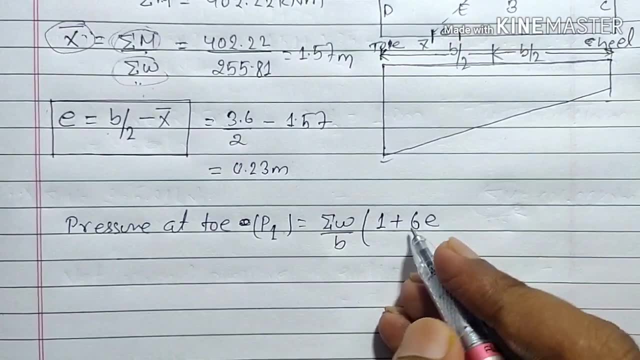 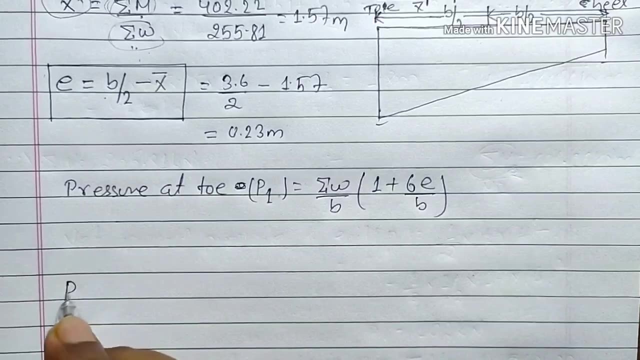 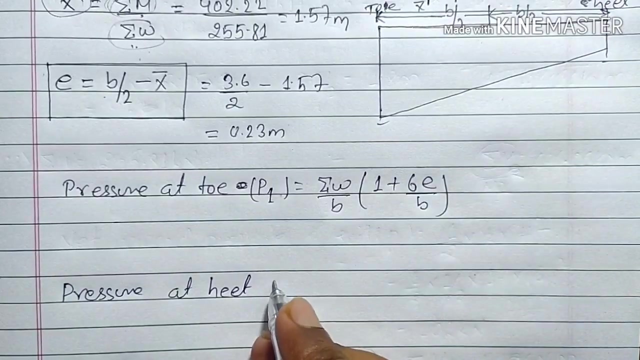 given by let. it is denoted by p1, then it will be equals to summation w by b times 1 plus 6e by b: 1 plus 6e. b b distribution at hill slab is given as pressure at hill, which is at point C, p2. 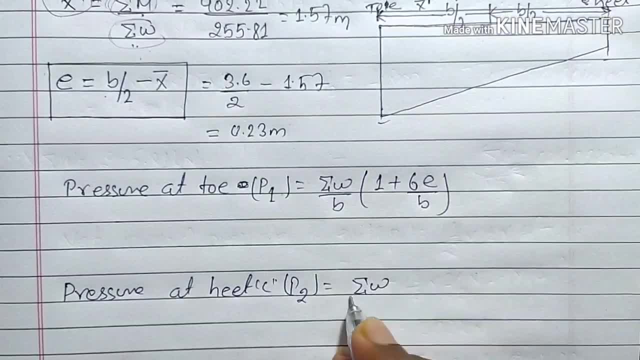 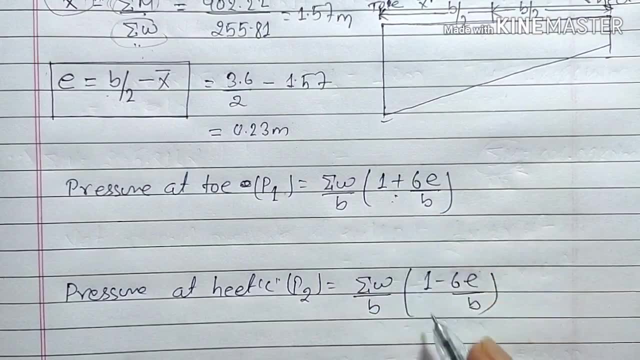 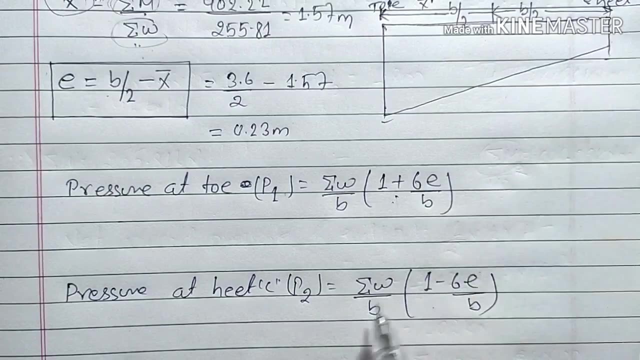 will be given by summation W by B times 1 minus 6 E by B. do not get confused between the positive plus and minus sign. always remember that pressure is maximum at toy and minimum at hill. so put positive sign for toy pressure and put negative sign for hill pressure. now put: 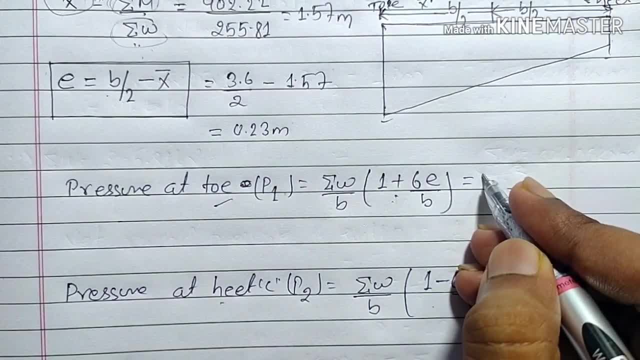 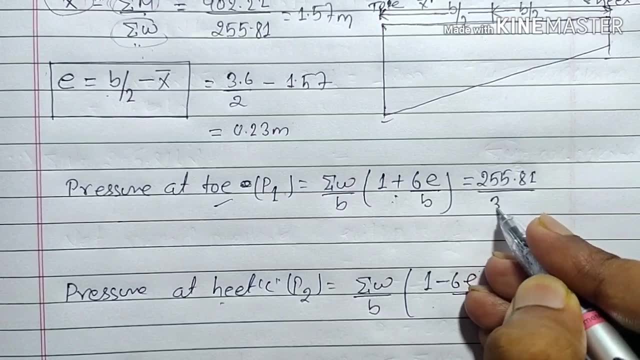 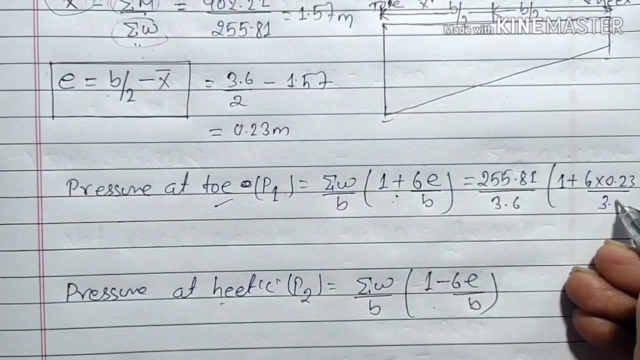 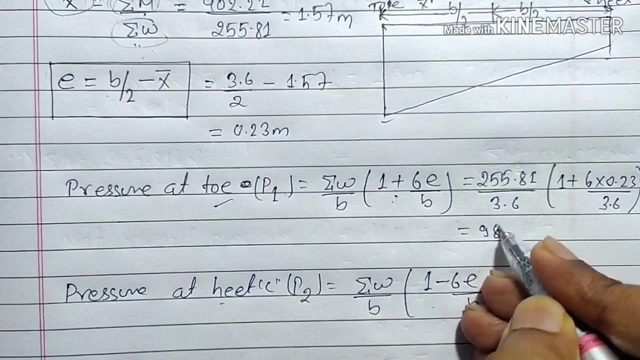 down the value which is equals to summation. W means 255.81 by B means 3.6 times 1 plus 6 into eccentricity, 0.23 by 3.6, and we will get the value of P1, which will be equals to 98.9- sorry, 29 kilonewton. similarly, put the value here and: 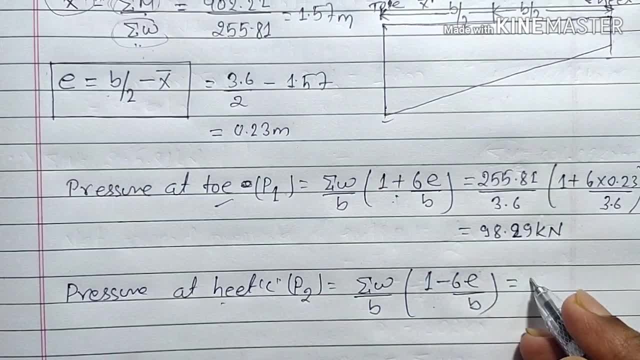 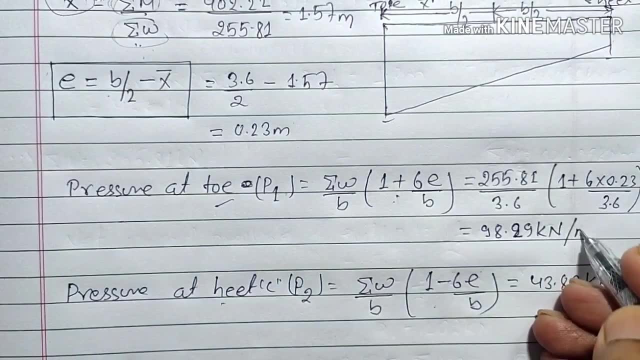 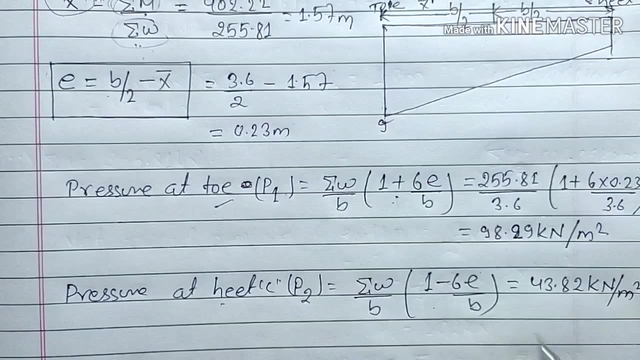 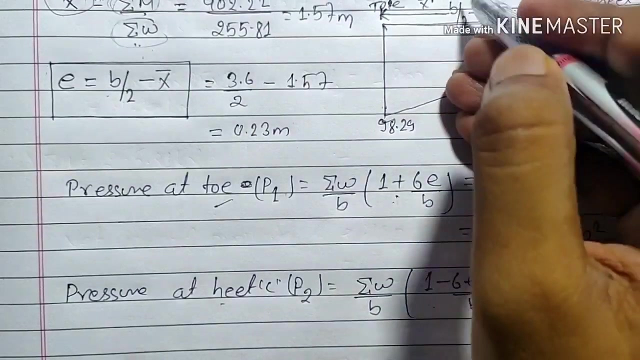 we will get the value of P2 equals to 43.82 kilonewton pressure. this is pressure, so kilonewton per meter square- again this will be kilonewton per meter square- means we have got the value here. this portion is 98.29 and this portion is 43.82. now time to find the pressure at. 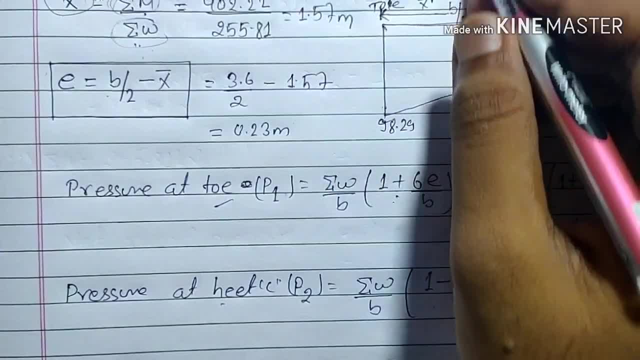 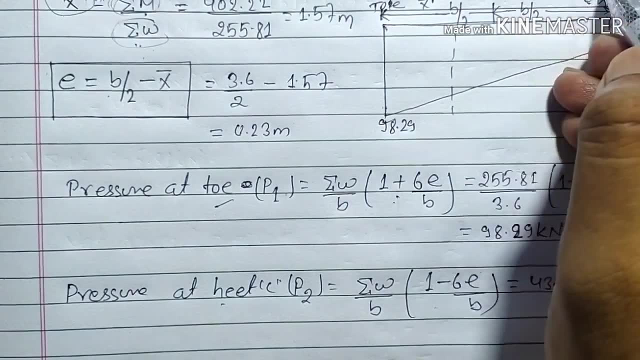 the junction of this toy slab and the steam means we need to find the pressure at E and again, we will be finding the pressure at the junction of this hill slab and the steam, which will be the pressure at point B. let's find it out. let's find it out. 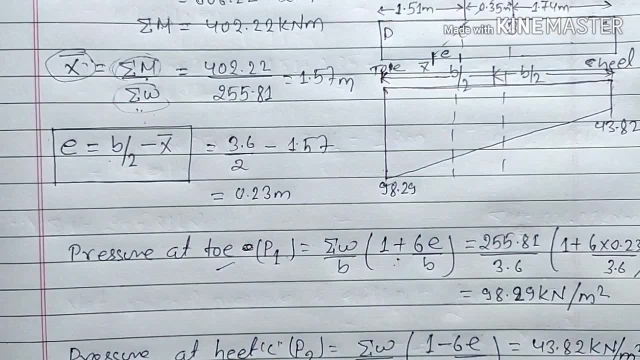 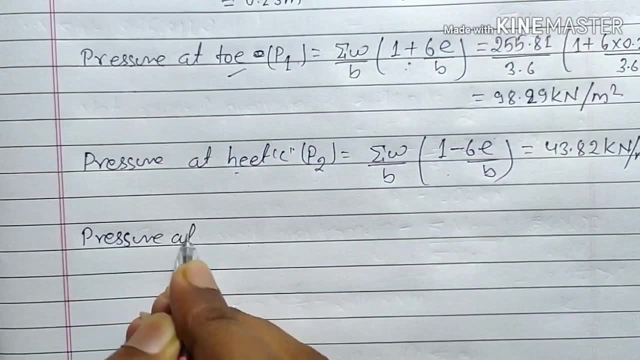 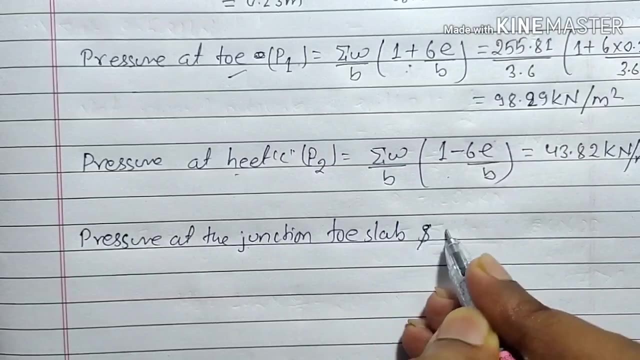 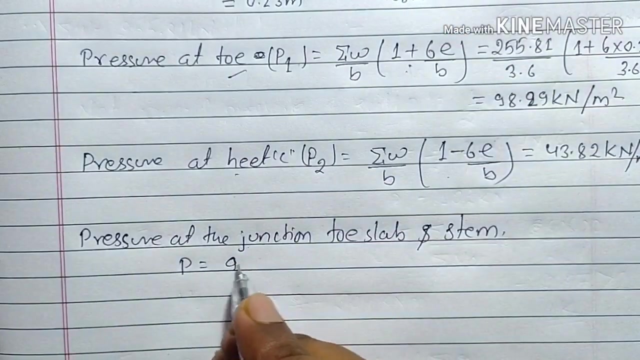 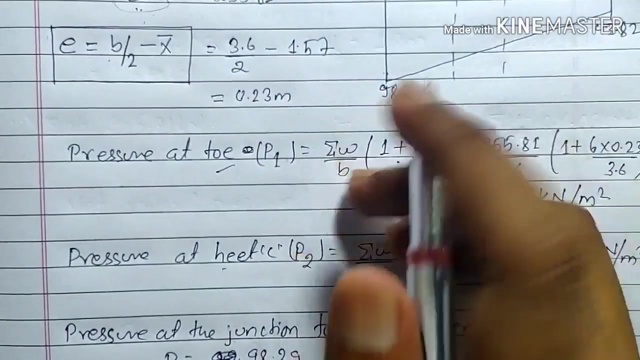 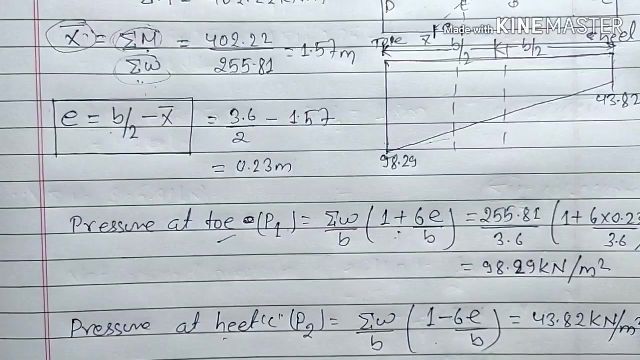 okay, okay, like this. so let's find out the pressure. pressure at the junction of toy slab and steam. we have P equals to 98, point, sorry 98.29, and the value is decreasing, as you see in diagram here the value is in decreasing, so write it down here: minus again here this: 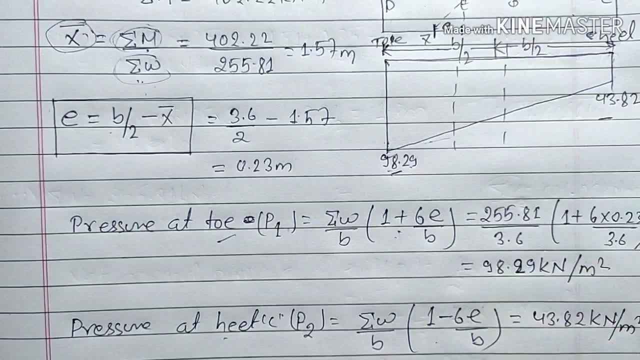 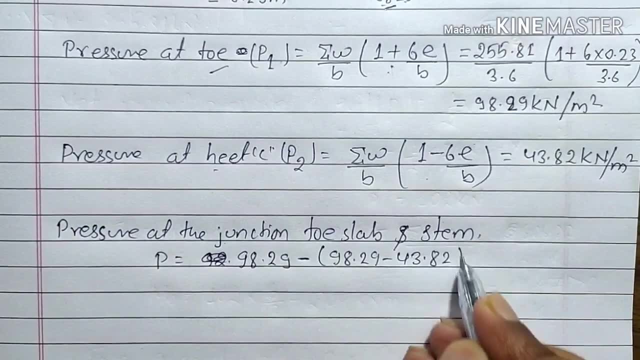 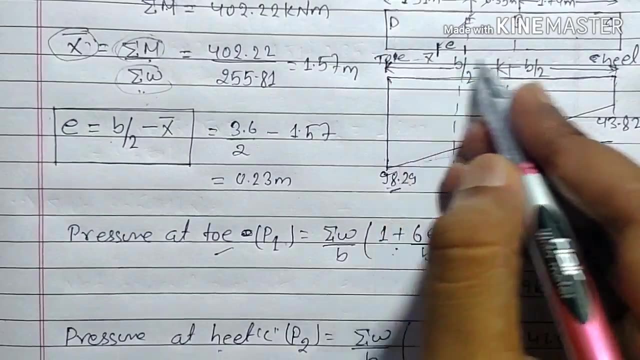 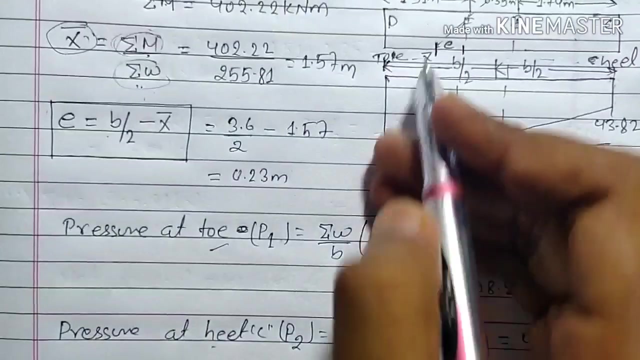 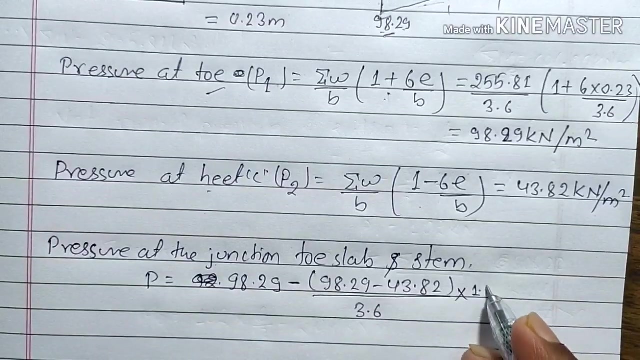 is 98.29 and here it is 43.82. so subtract it here: 98.29 minus 43.82 divided by whole base, and the whole base width is here. whole base width is 3.6 meter, so divide this by 3.6 and multiply this by span, 1.51 meter, so write it down here: 1.51 meter. on solving this, we will. 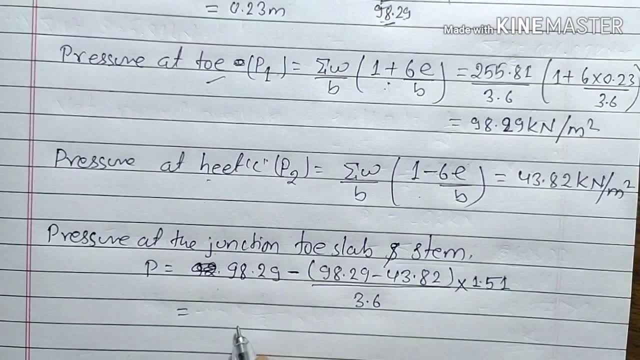 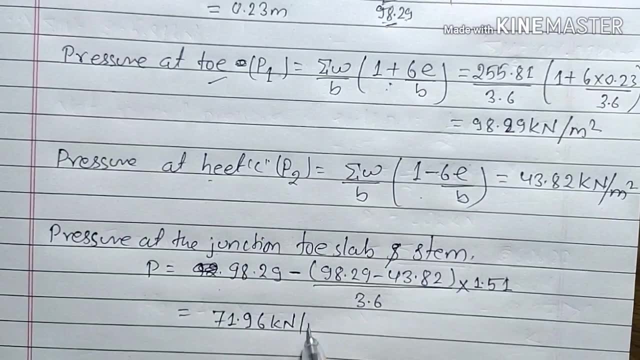 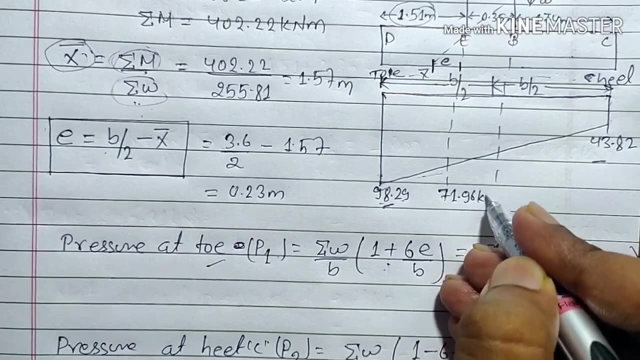 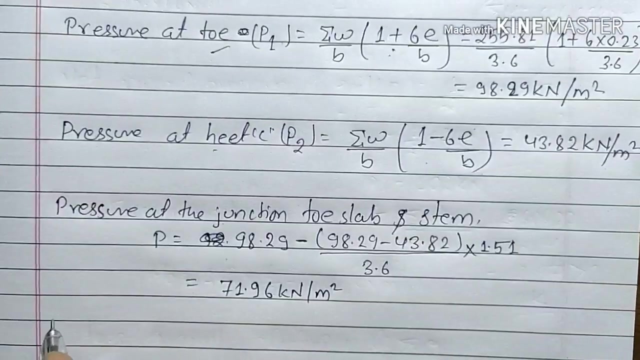 get the pressure at the junction of toy slab and the steam as 71.96 kilo newton per meter square and we have got it's value as 71 point nine six kilo Newton per meter square. similarly, let's find out the pressure at this person B. so again, we will write. 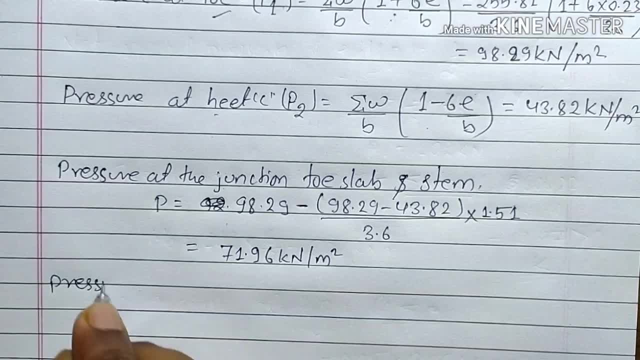 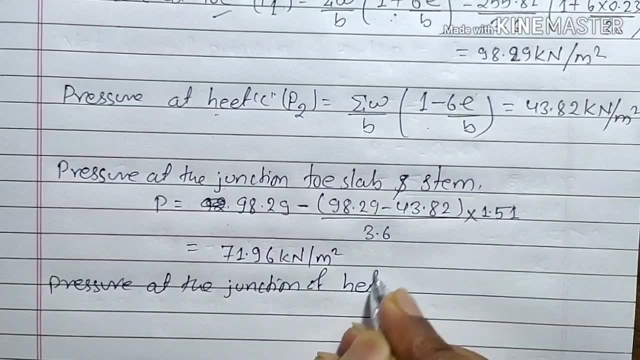 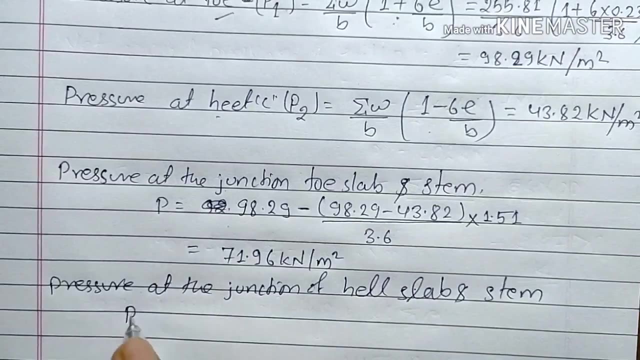 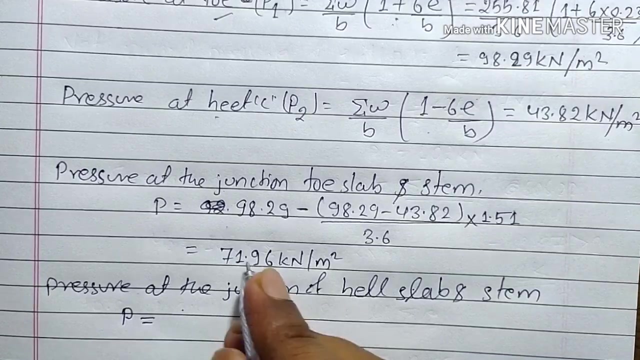 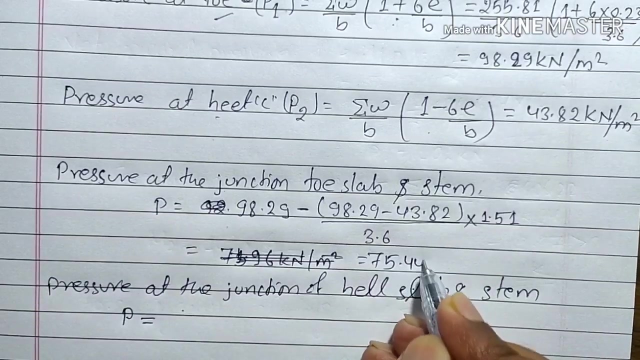 down here. pressure at the Junction of Hill slab, Hill slab and steam will be given as 71.96 neurological Newton per meter square. so our given value is 71.96. given by p equals to- sorry for this. here the value will be 75, 75.44 kilonewton per meter. 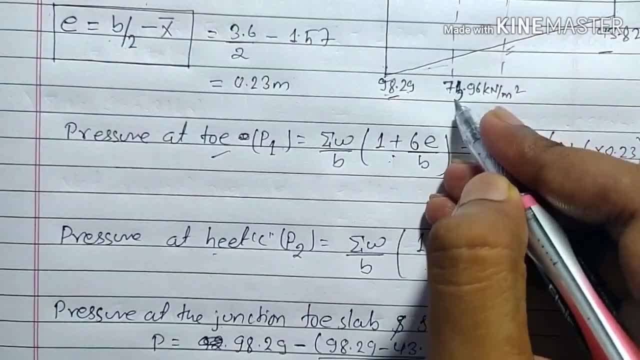 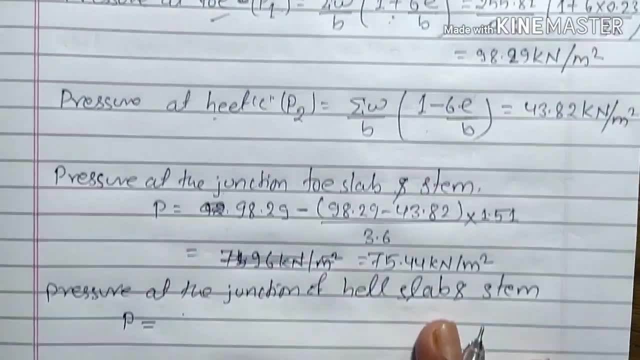 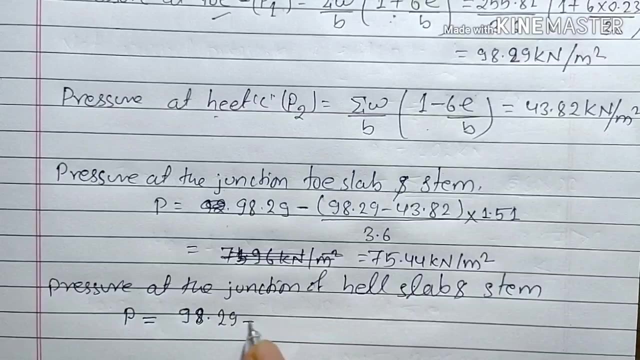 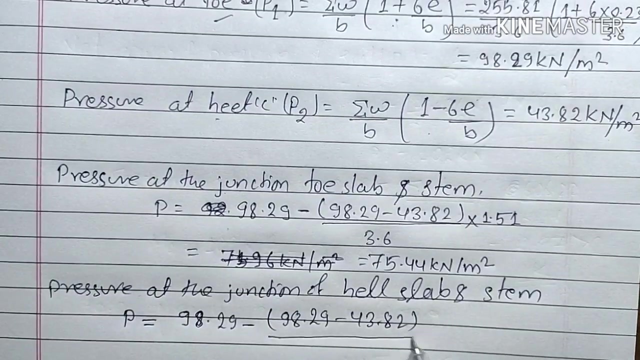 square. so this is our 75.44 kilonewton per meter square. similarly for p2, we will do again. do here 98.29 minus 98.29 minus 43.82 upon 3.6. similar to this, but we just need to change. 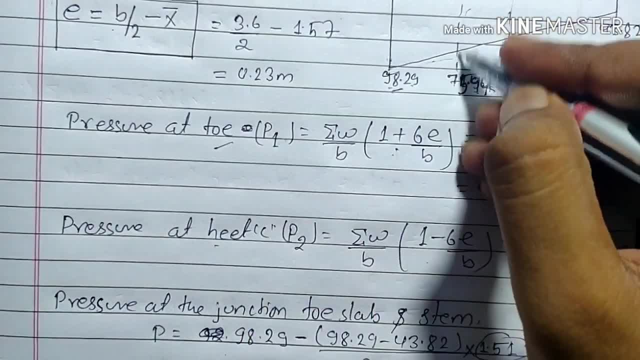 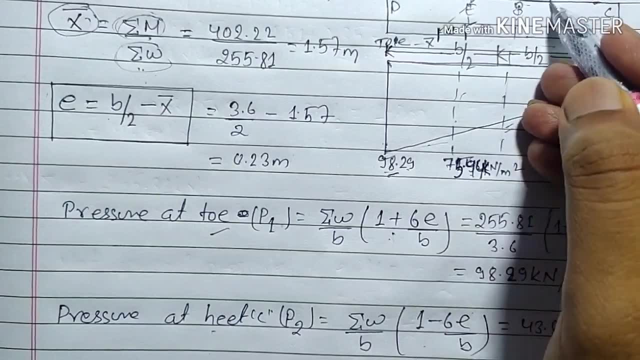 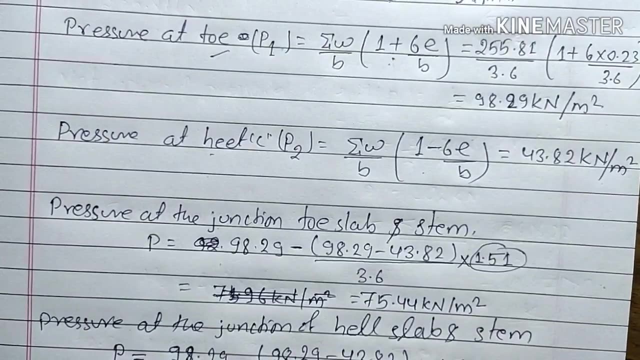 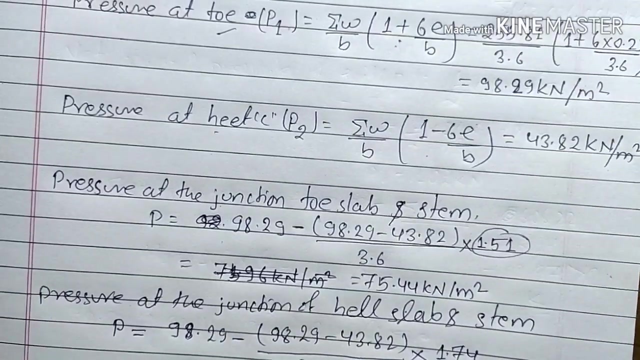 the span here, while finding the pressure at this portion at e. while finding the pressure at e, we took this span. now for finding pressure at b, we will take this span, which is 1.74 meter, Now, write it down here into 1.74 and we will get the value as p equals to 71.96 kilonewton. 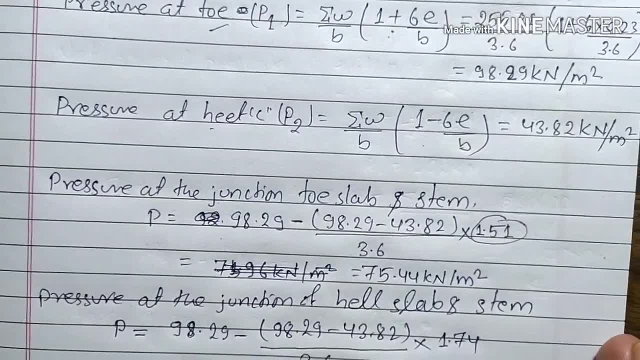 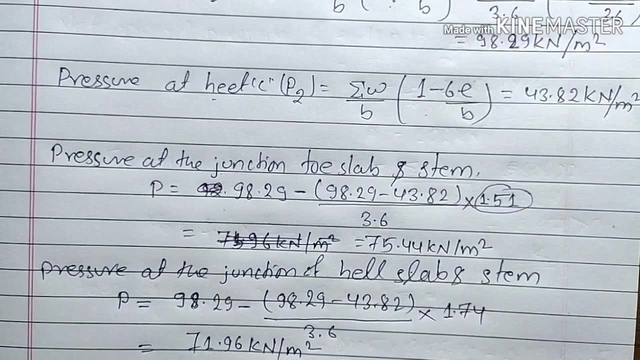 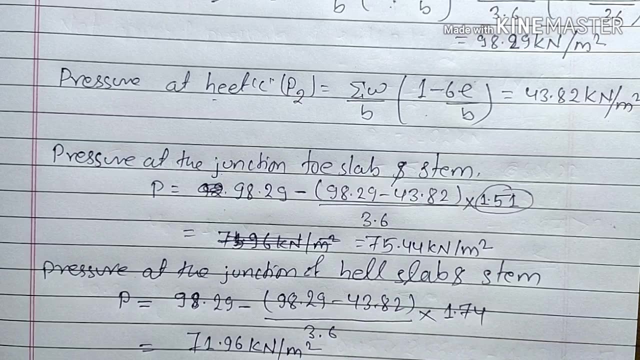 per meter square. now let's move toward the new step, which is our step 5, this much up to step 4, in which we have checked the stability of the wall and find out the pressure at the junction as well, at the end of the toy and hill slab. 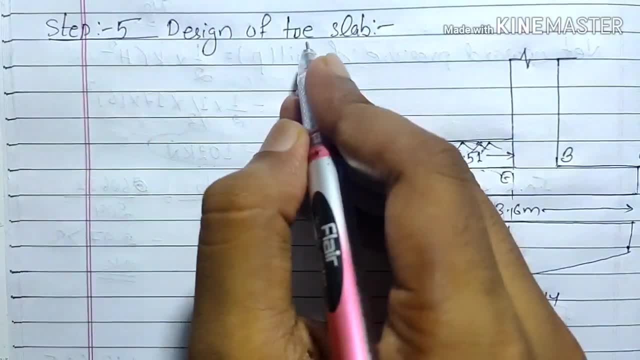 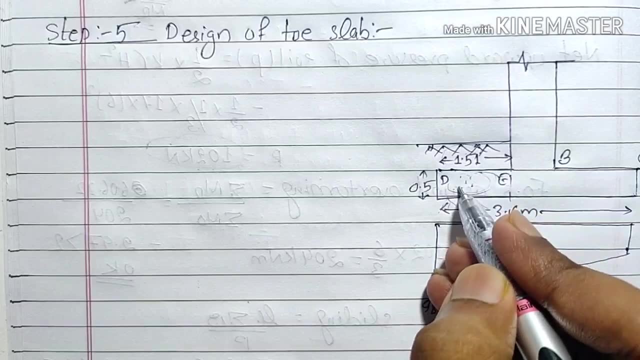 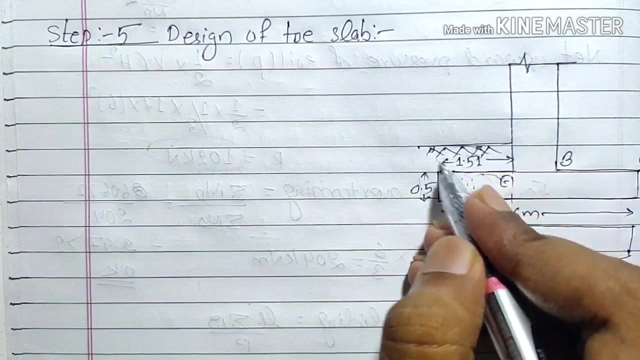 Let's move toward step 5. In which we will design the toys. here in step 5, we will be designing the toy slab, and for toy slab we will consider the downward weight of the toy slab and the upward pressure of the soil. so we will and we will neglect the weight of the soil which is lying above the. toy slab. what we will consider downward weight of slab and second upward weight of slab and second upward weight of slab. So we will spend upward pressure of soil, so we will have downward weight of slab. per unit area means 1 meter squared area. unit area it will be given as 0.5 into 1, into 17.9. 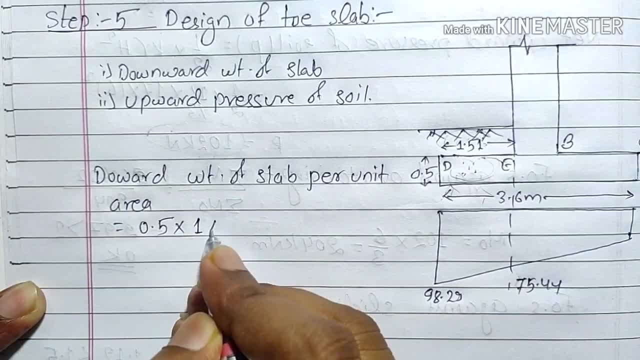 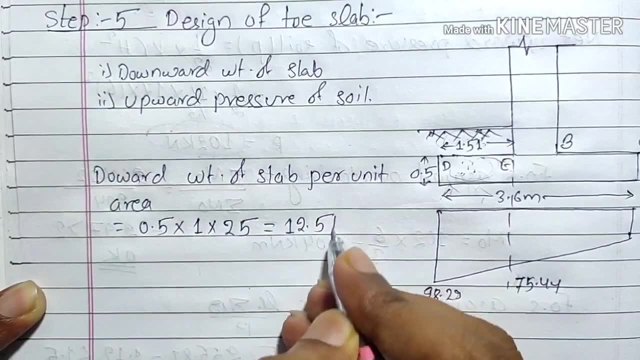 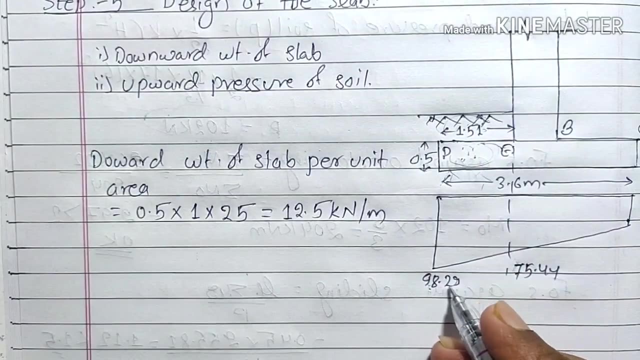 kilo buyyl of the suspended in one meter square area. this will be given as its all inside this unit area. unit weight of soil- or sorry, concrete- is 25, so we will get here 12.5 kilo newton per meter and the pressure at point d and e are respectively 9.2, 98.29 and 75.44. 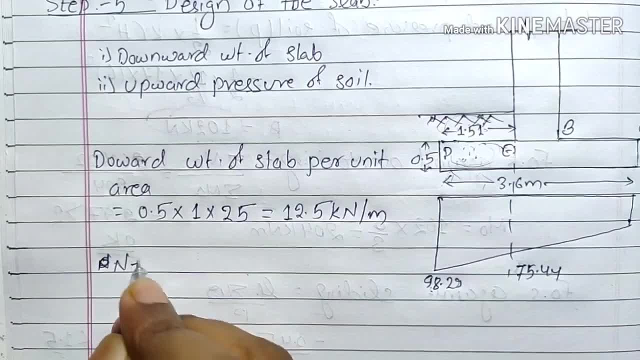 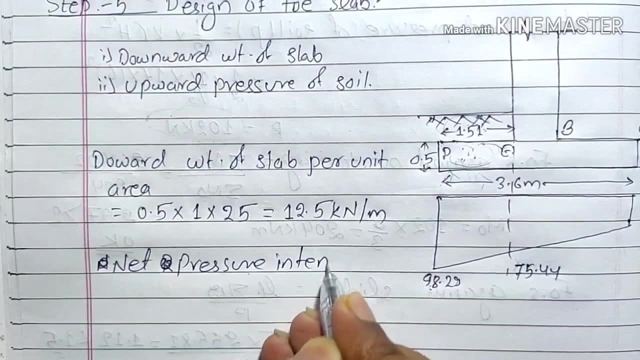 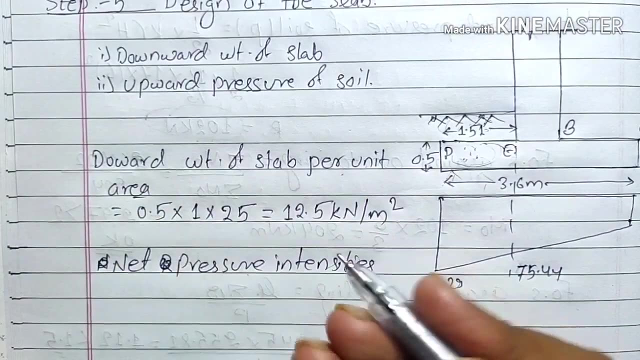 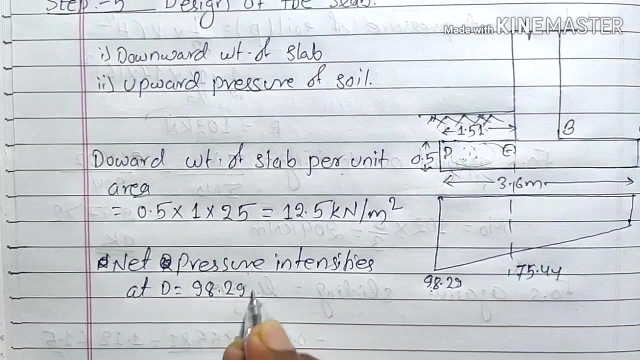 so resultant or net pressure intensities. net pressure intensities is it is met kilo newton per meter square for unit area. area means its meter square and net pressure intensity at d will be equals to 98.29 minus 12.5 and similarly at e will be. 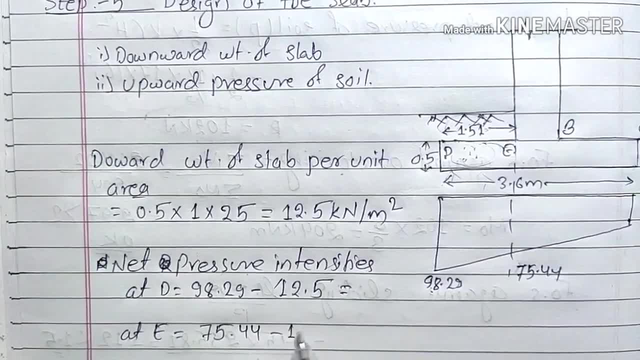 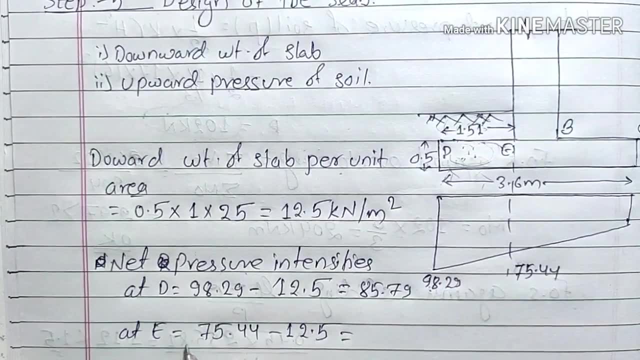 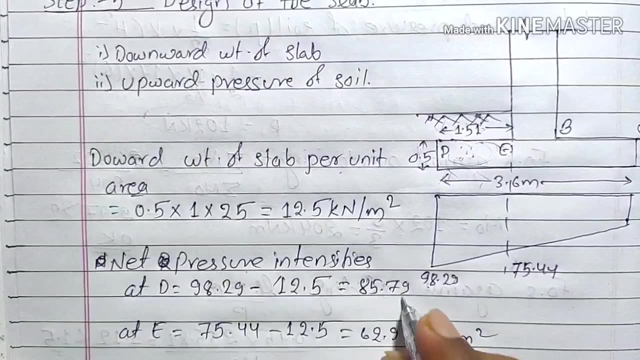 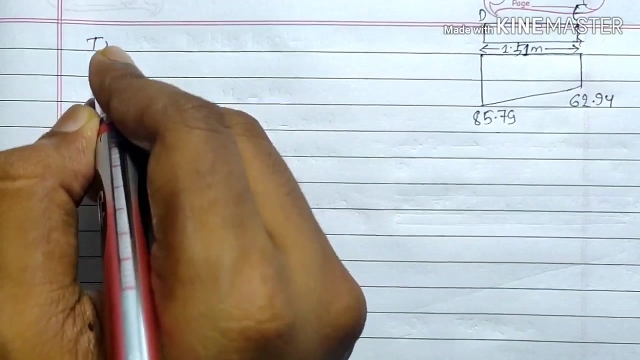 equals to 75.44 minus 12.5 and we will get here 85.79, and at e it will be 62.94 kilo newton per meter square. kilo newton per meter square. now let's find out a total shear force at e. so write it down here: total. 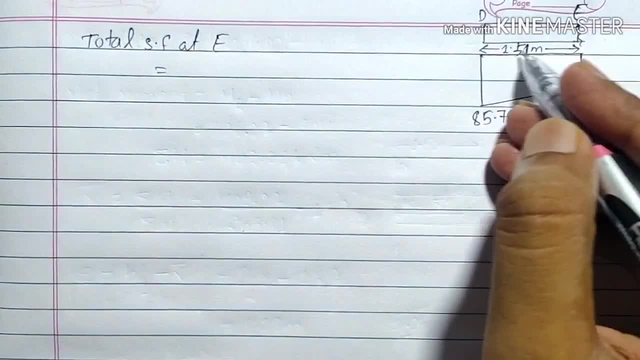 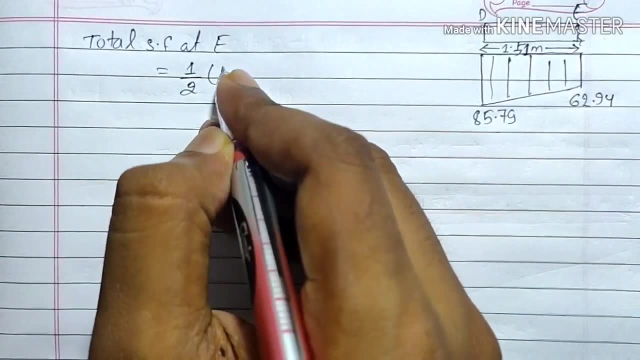 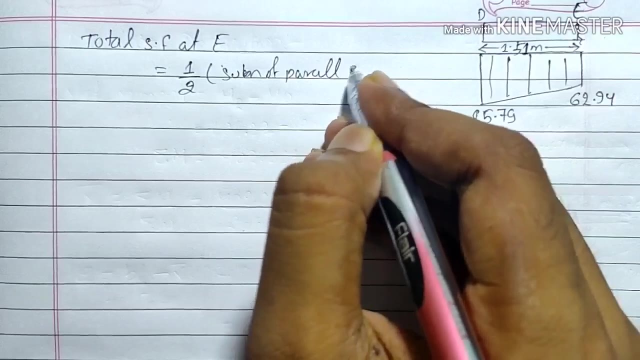 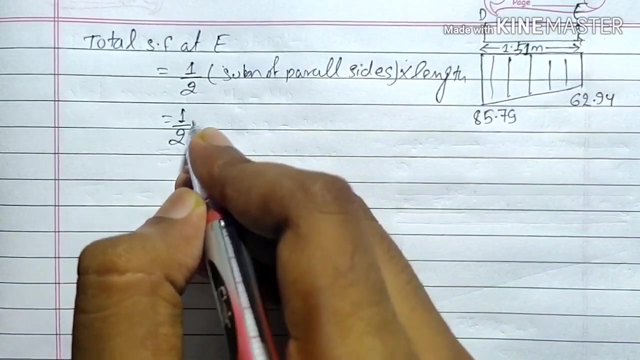 shear force at e, which will be equals to the area of this trapezium. and we have the formula for finding the area of trapezium, which will be equals to half into sum of parallel sides. this sum of parallel sides, sum of parallel sides, into length. so we will have here half into 85.79 plus 62 point. 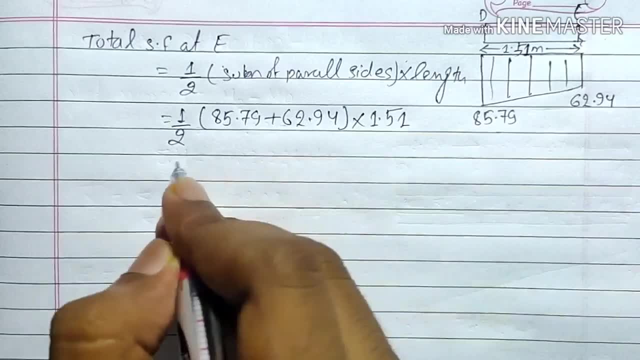 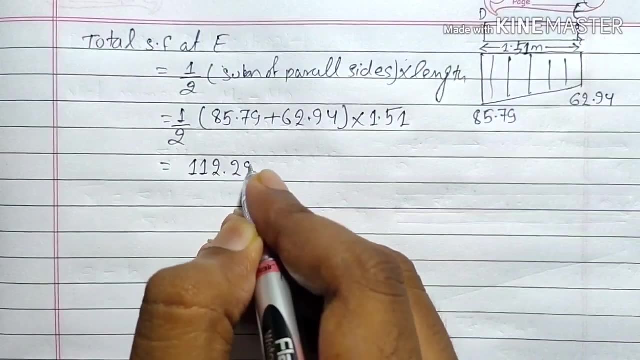 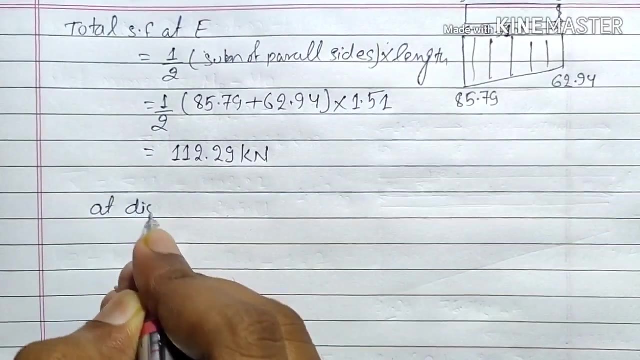 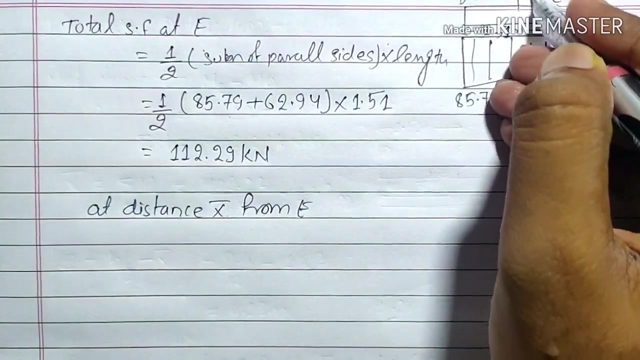 94 into 1.51 and this will be equal to 112.29 kilo newton, and the shear force is acting at distance x bar from e, distance x bar from e. now we need to find the value of x bar. for that we need to multiply this. 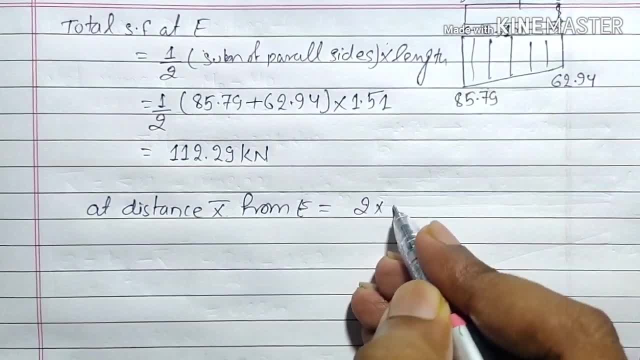 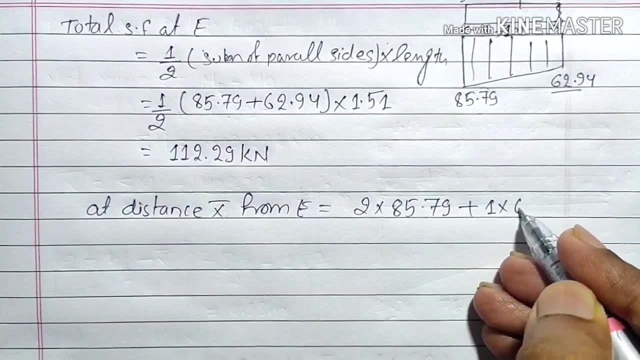 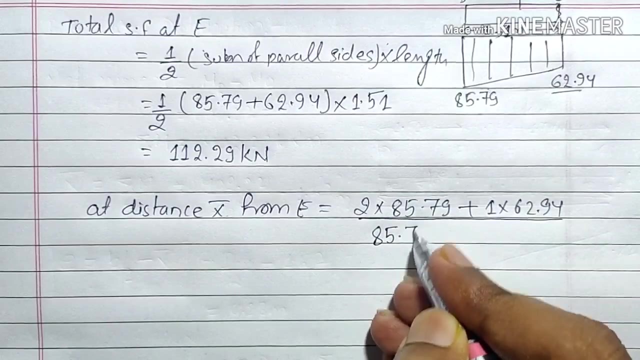 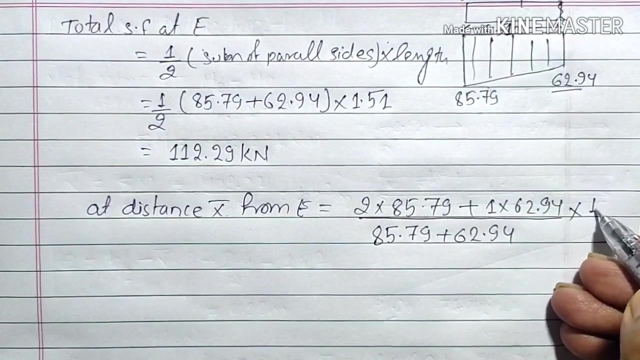 outer on pressure by two times, so it will be written as 2 times 85.79 plus 1 times 62.94. by the sum of the forces: 80, some of the pressures: 7. 85.79 plus 62.94 times span means 1.51 divided by 3.. you can work it. 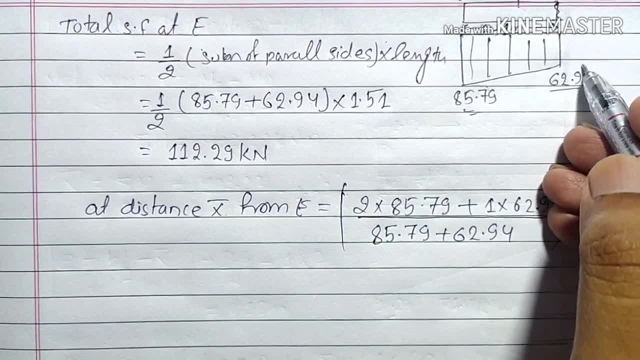 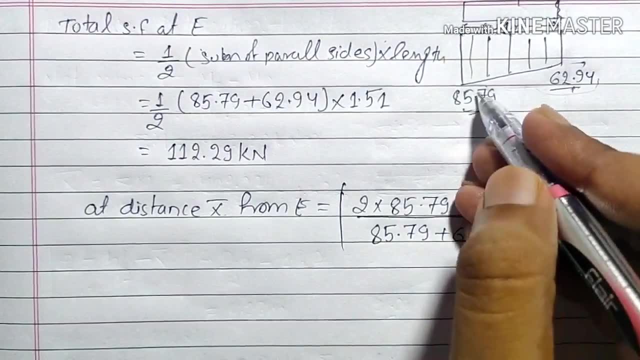 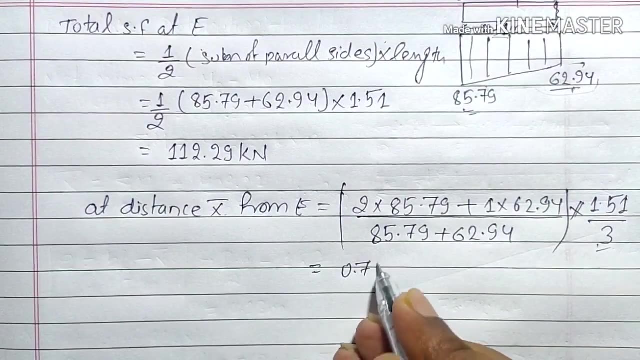 it just multiply the outer by twice and then add one times inner and then divide by the sum of both into multiply by the span and then divide by 3. then we will get the value of X bar at 0.79 meter, which is from E. now for bending moment. 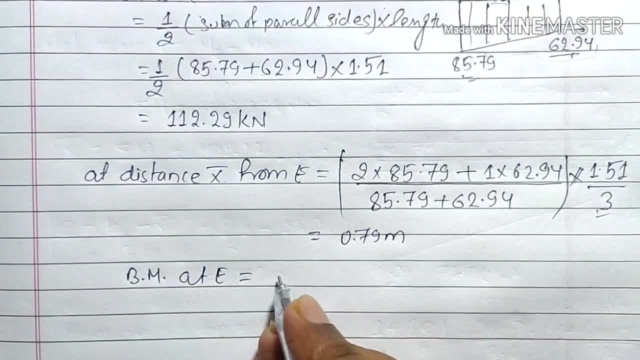 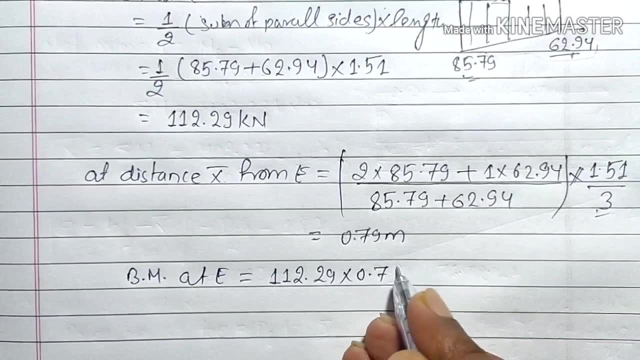 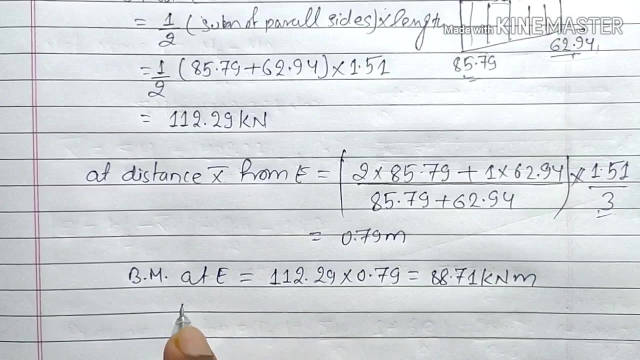 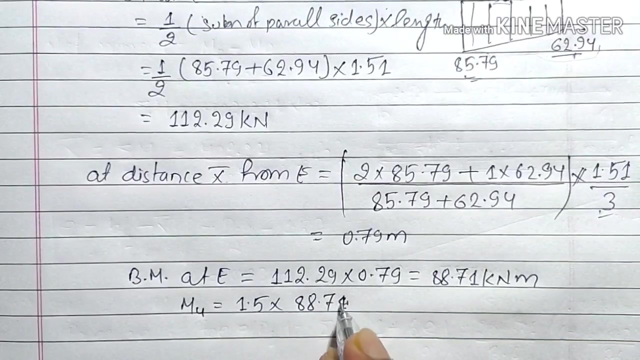 at E we will have one one, two point two, nine into zero point seven nine, which will be equal to eighty eight point seven, one kilo Newton meter, and MU, equals to one point five, into eighty eight point seven, one which will be equals to one hundred thirty three kilo Newton. 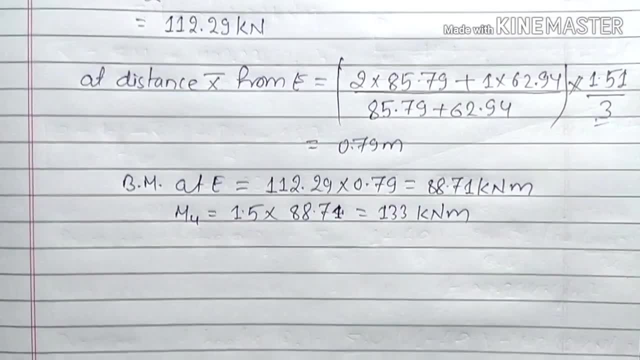 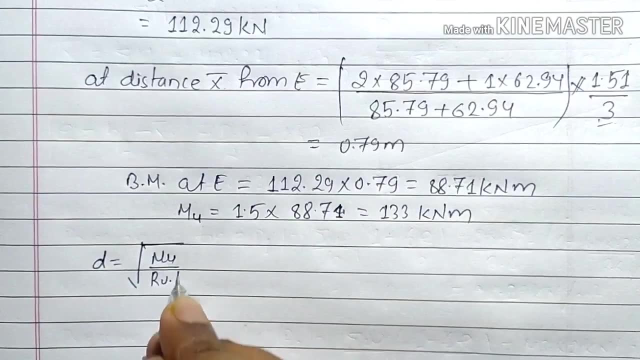 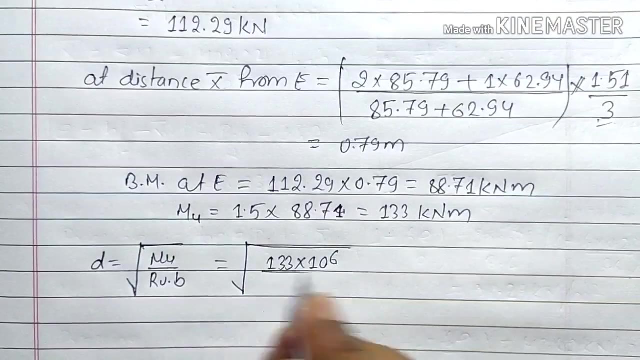 and meter. now time for finding the effective depth. and for effective depth we have a formula: D equals to root under MU by RU into B. so put the value here, 133 into 10, to the power. 6 divided by RU means two point seven, six, one into thousand and. 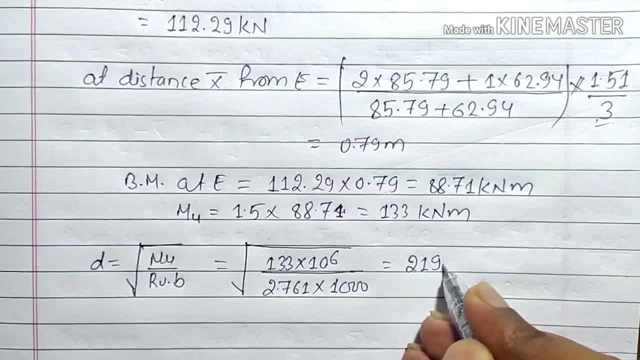 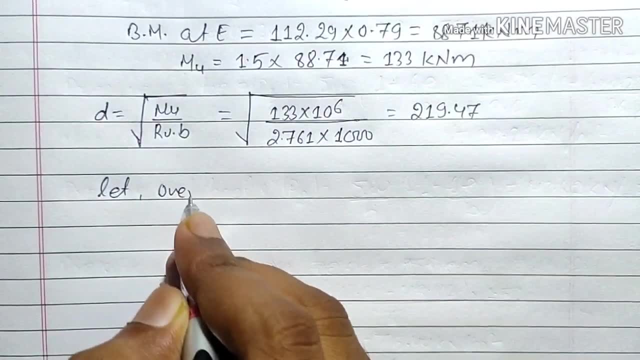 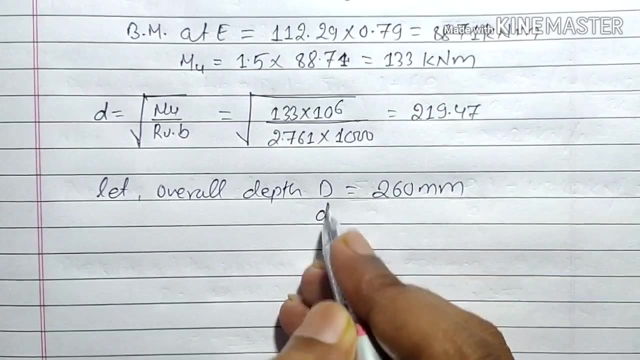 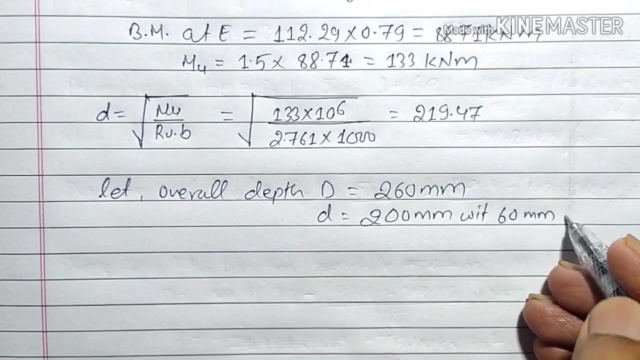 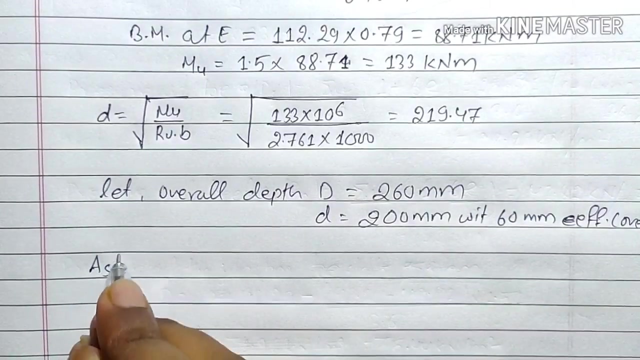 here we will get the value of effective depth as two hundred nineteen point four seven. now let us take overall depth. let overall depth, capital D equals to 260 millimeter and effective depth equals to 200 millimeter width. sixty millimeter effective cover, 60 millimeter effective cover. so now find out the AST for AST. we 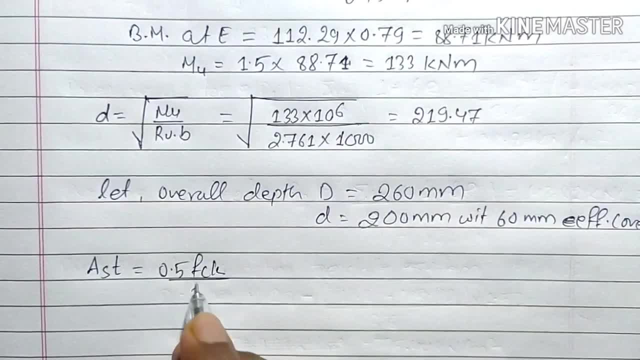 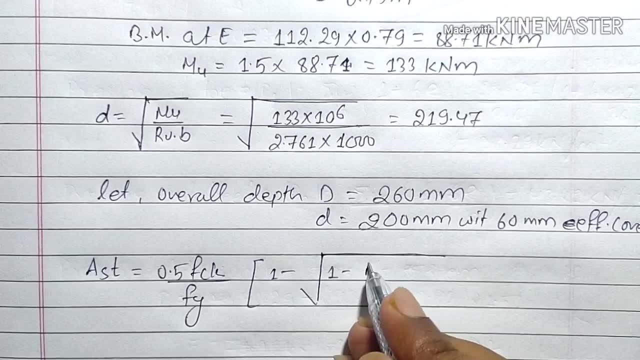 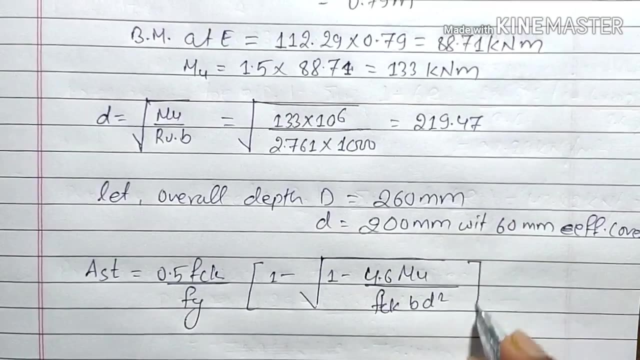 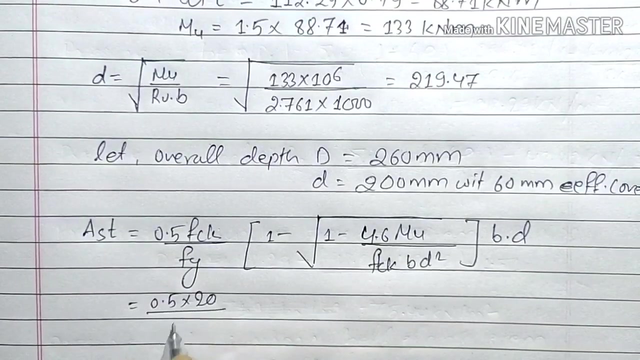 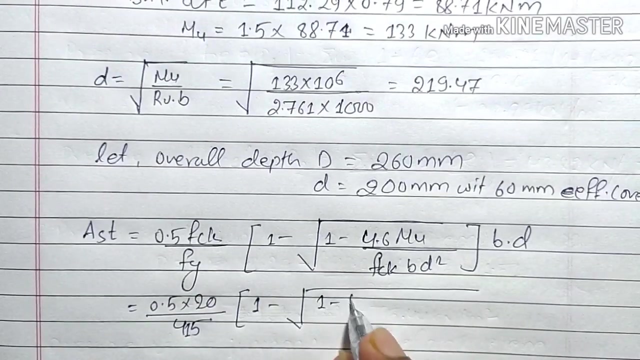 have a formula zero point five: FCK by Fy times 1 minus root under 1 minus 4.6 MU by FCK, BD square times B into D. now put the value here 0.5 into 20 by 415 times 1 minus root under 1 minus 4.6 into. 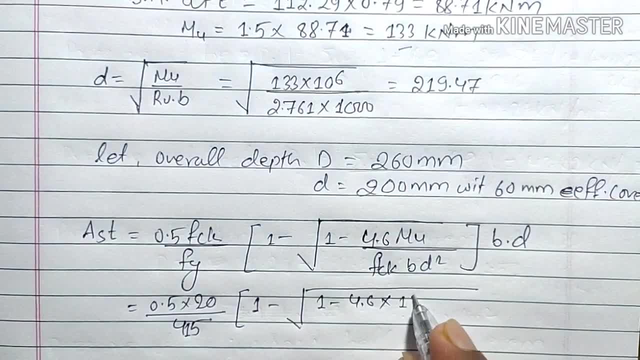 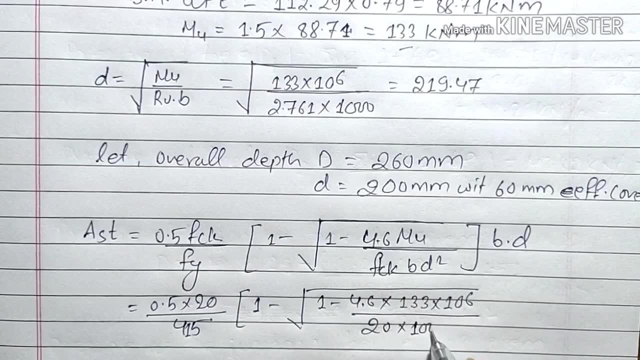 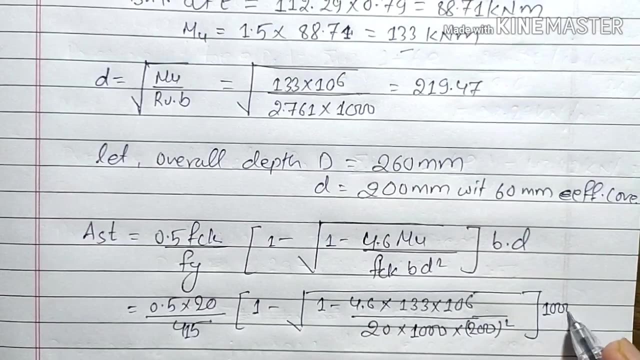 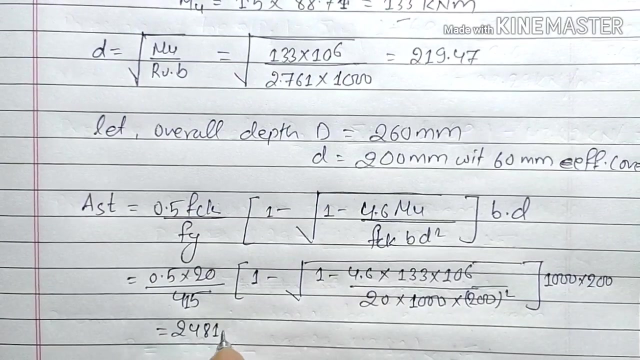 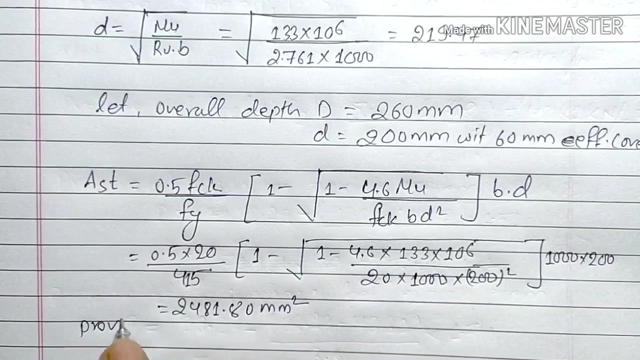 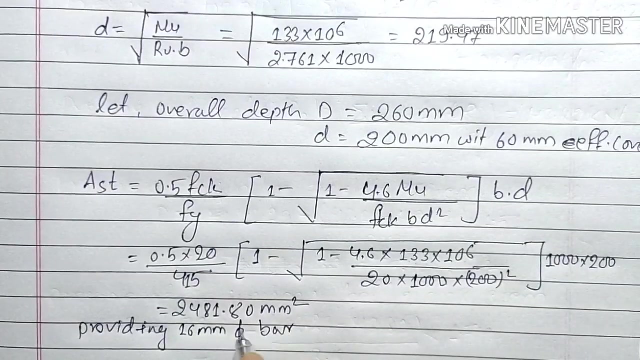 and the value of MU here is 133 into 10 to the power 6 divided by 20 into 1000, into 200. square times 1000 into 200, then we will have here AST equals to 2481.80 millimeter square and providing 16 millimeter bar, 16 millimeter dia bar. 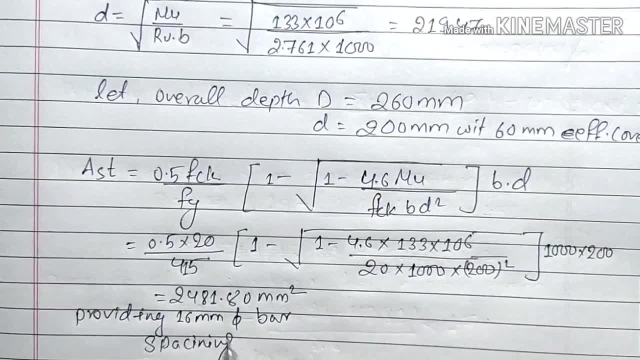 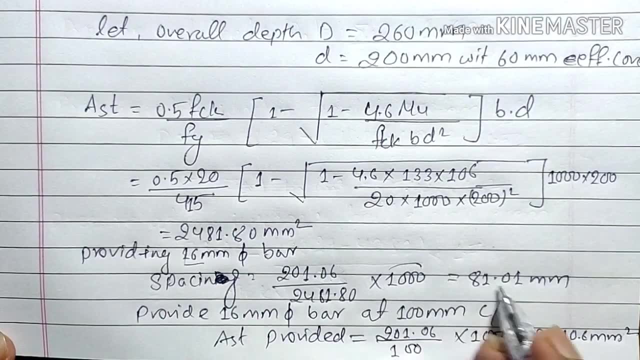 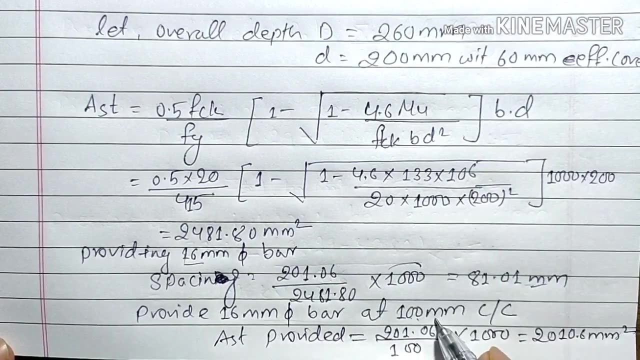 spacing equals to spacing equals to AST of 1 bar of 16 millimeter diameter divided by total AST in 2000, then we will get here AST equal to 0.01. we are providing 16 millimeter dia, so let's provide it at hundred-hundred. 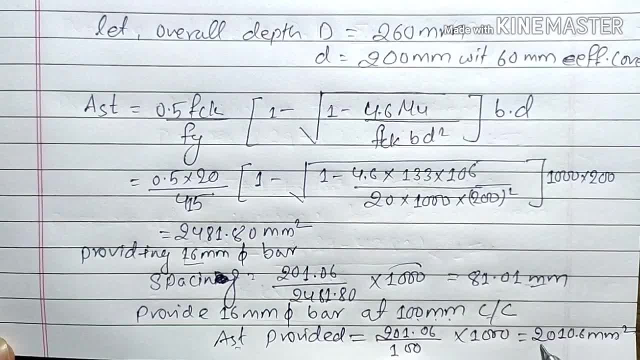 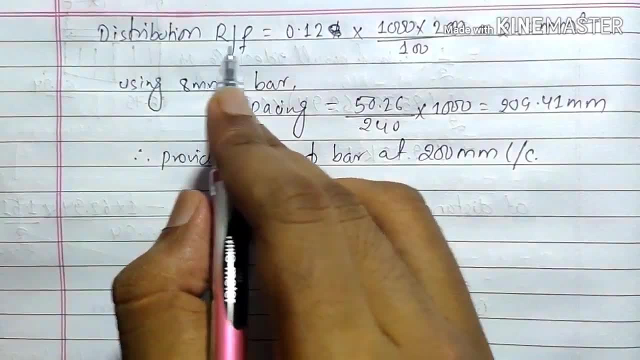 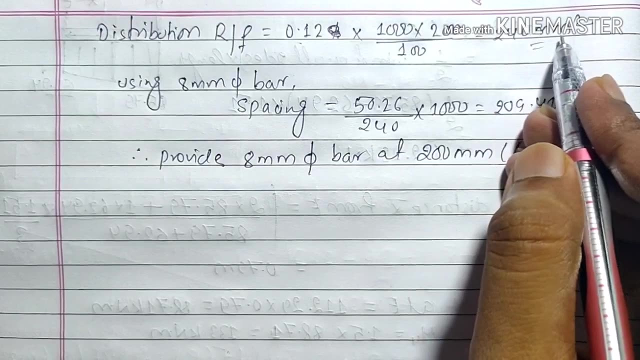 millimeters sensor to center. so AST provided will be two to zero, one six, one 0.6 millimeter square. now let's design the distribution reinforcement. so distribution reinforcement is usually taken as Putin percent of the gross area divided by 100. we will get here 240 millimeter square, providing 8 millimeter. 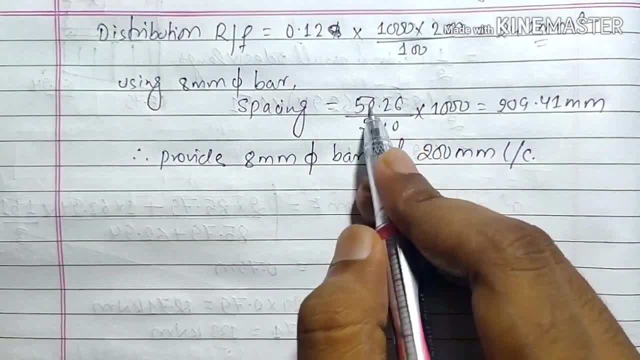 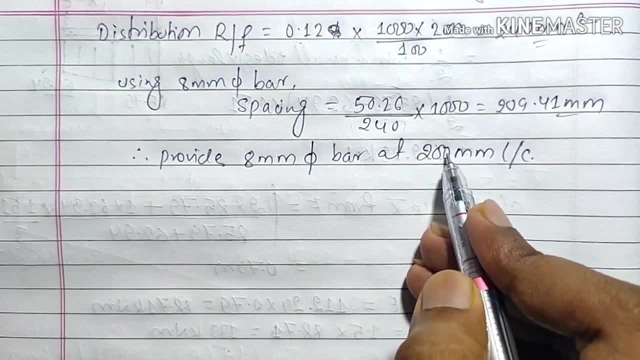 dia Bar is given by AST of 1 bar of 8 millimeter divided by total AST into thousand, we have got this. so we have provided 8 millimeter dia bar at 200 millimeter center to center. now let's move toward the design of a steps. design of hill. 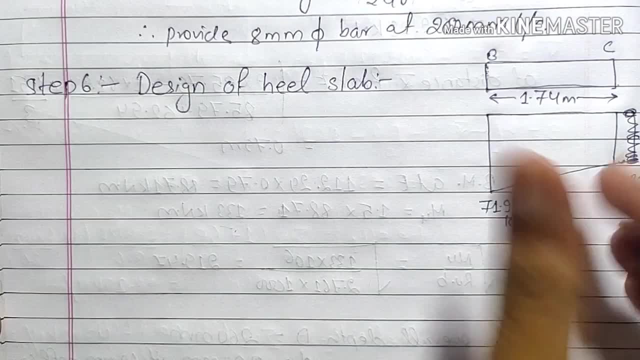 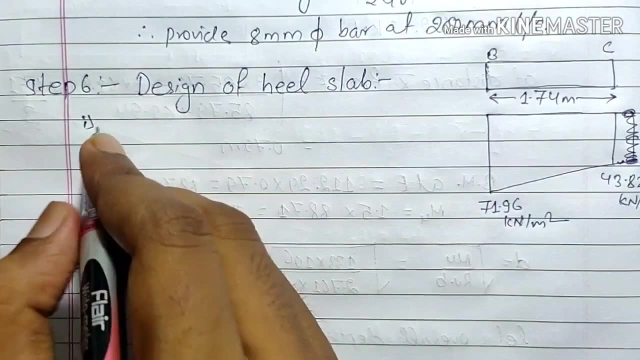 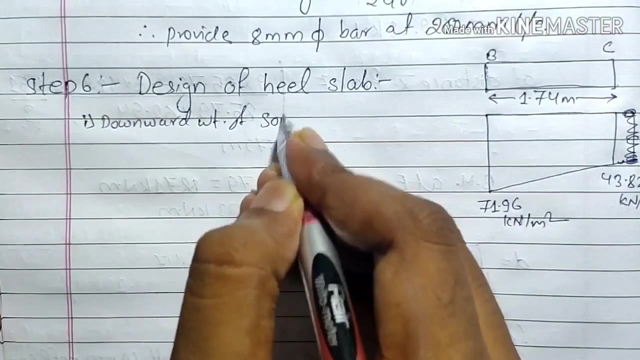 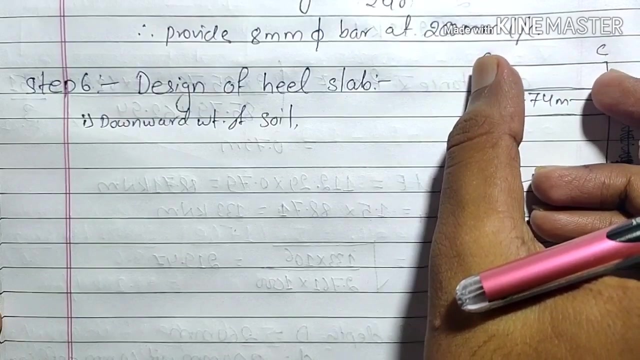 slab which is going to be our step 6. here I have drawn the small portion of the hill slab and here three things will. three weight will be taken into consideration. that is, our downward, downward weight of soil, as we have seen in the in overall diagram there that our hill slab was loaded with some soil up. 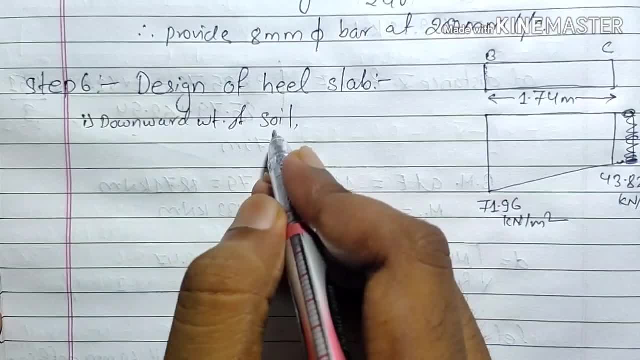 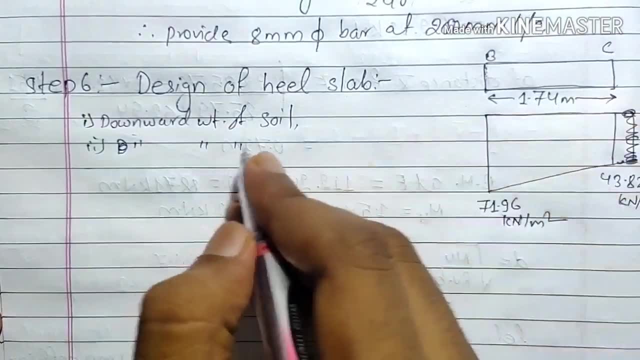 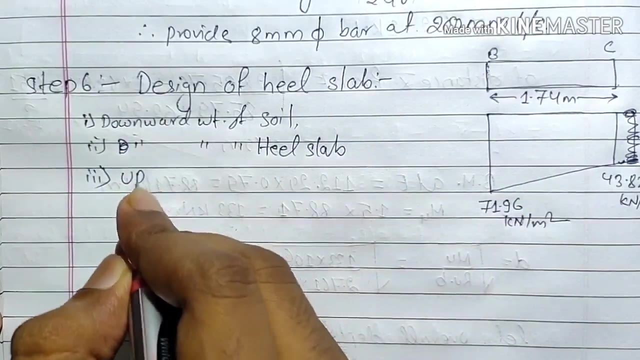 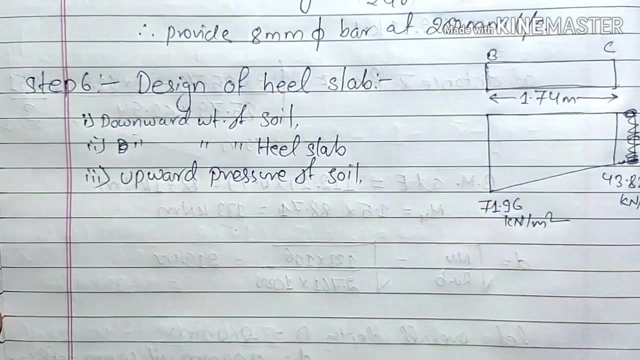 to the height h1. so we need to consider the downward weight of soil. second thing, we will consider the downward downward weight of hill slab, hill slab. and the third thing we will be considering is upward pressure of the soil. so let's begin the step now, so we will have the way. downward weight of 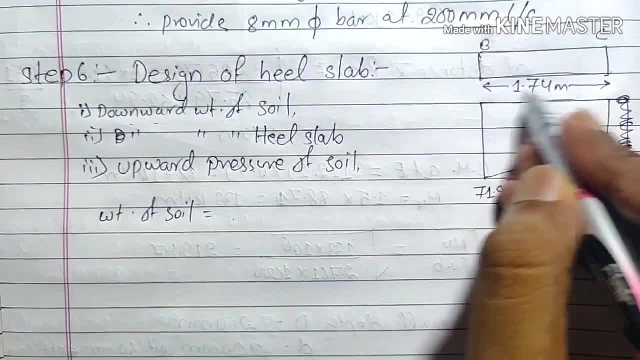 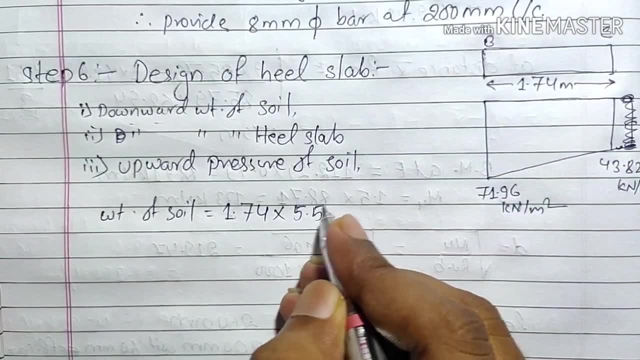 soil equals to this span means area of rectangle 1.74 and the height of soil was 5.5 meter. into unit weight of soil will be. the height of the soil will be 5.5 meter. into unit weight of soil will be. the height of the soil was 5.5 meter. into unit weight of soil will be. 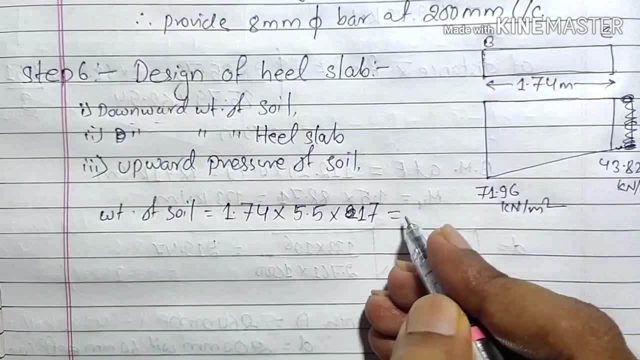 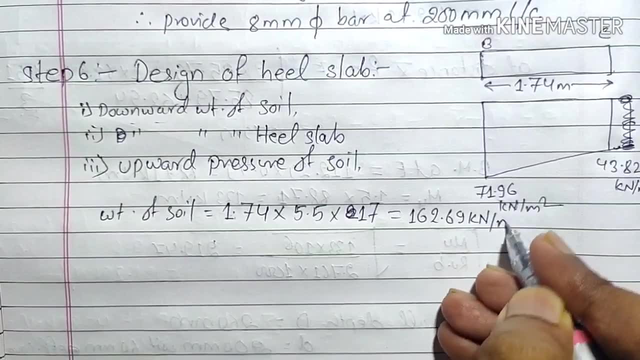 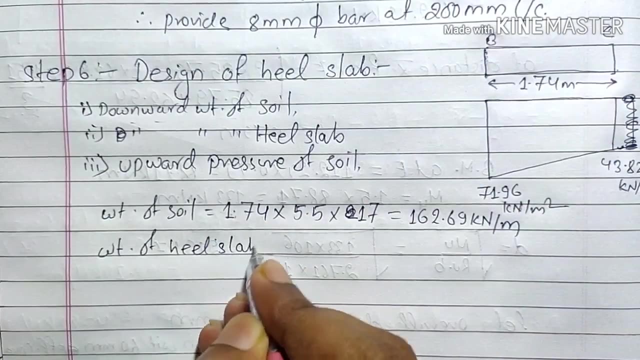 17 kilo Newton per meter square. so we will have the weight of soil as 162 point 162 point 162 point 6, 9 kilo Newton per meter. similarly, weight 6, 9 kilo Newton per meter. similarly, weight 6, 9 kilo Newton per meter. similarly, weight of hill slab equals to this 1.7, 4. 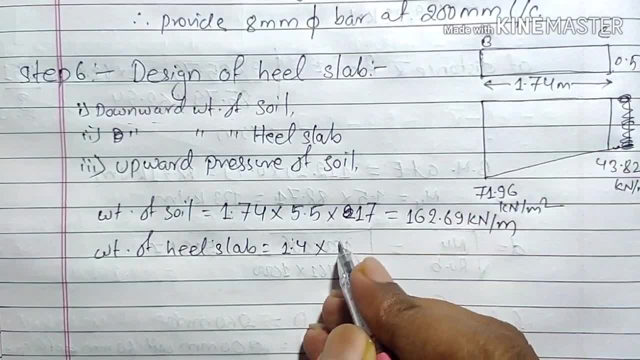 of hill slab equals to this: 1.7 4 of hill slab. equals to this: 1.7 4 into. thickness is 0.5- 1.7 4 into 0.5 into. into thickness is 0.5- 1.7 4 into 0.5 into. 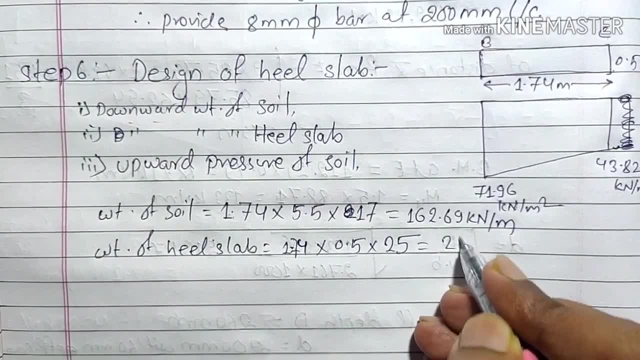 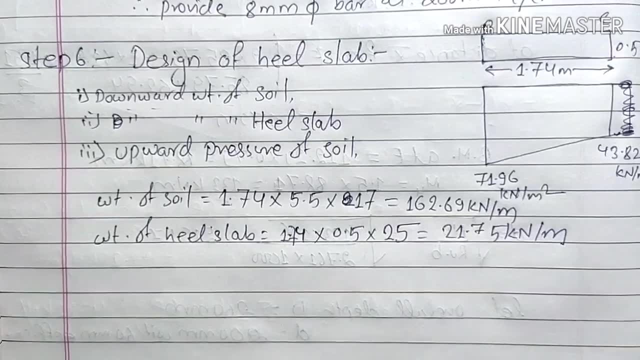 into thickness is 0.5, 1.7, 4 into 0.5. into unit weight, which will be equals to 21 point unit weight, which will be equals to 21 point unit weight, which will be equals to 21 point 7, 5 kilo Newton per meter, and again, 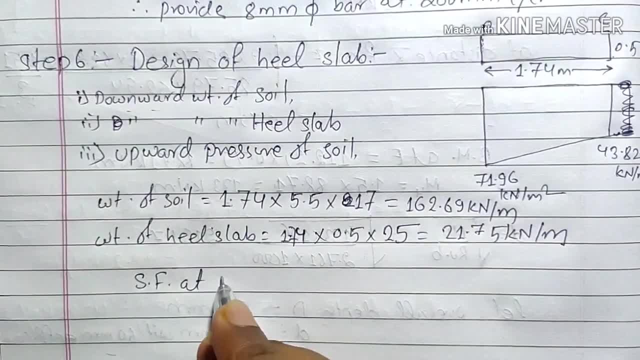 7, 5 kilo Newton per meter, and again 7, 5 kilo Newton per meter, and again the shear force at B, shear force at B. the shear force at B. shear force at B, the shear force at B. shear force at B equals to this multiply the outer outer. 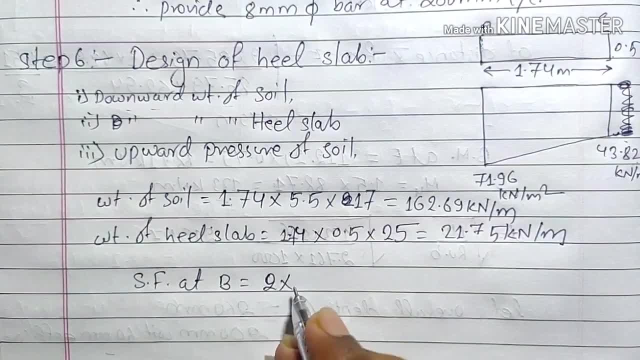 equals to this: multiply the outer- outer. equals to this: multiply the outer- outer. pressure intensity by 2, so it will be 2. pressure intensity by 2, so it will be 2. pressure intensity by 2, so it will be 2 times. sorry, we need to find the shear. 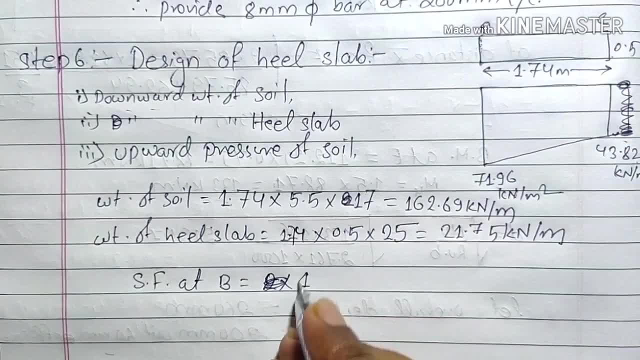 times. sorry, we need to find the shear times. sorry, we need to find the shear force. so again, we need to find the area of force. so again, we need to find the area of force. so again, we need to find the area of this diagram which will be given as: 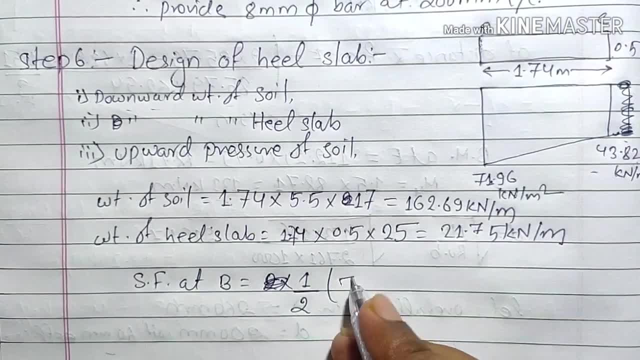 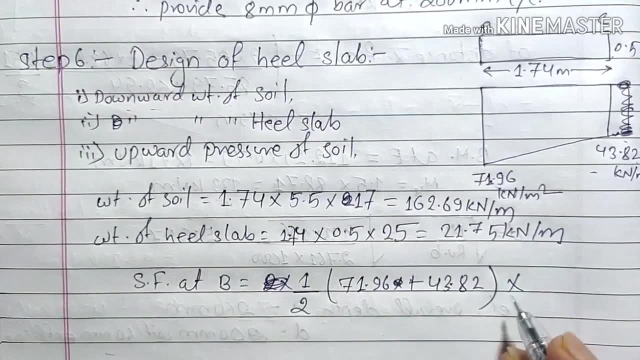 this diagram, which will be given as. this diagram, which will be given as half into sum of parallel sides means half into sum of parallel sides, means half into sum of parallel sides means seventy one point nine six plus forty. seventy one point nine six plus forty seventy one point nine. six plus forty three point eight. two into span means one. 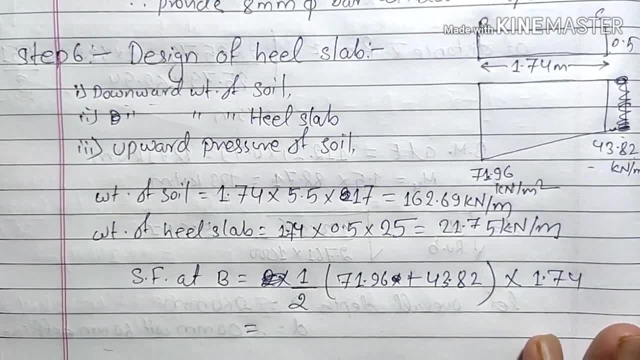 three point eight. two into span means one. three point eight. two into span means one point seven, four meter. so we will get point seven, four meter. so we will get point seven, four meter. so we will get the shear force of B as one hundred point. the shear force of B as one hundred point. 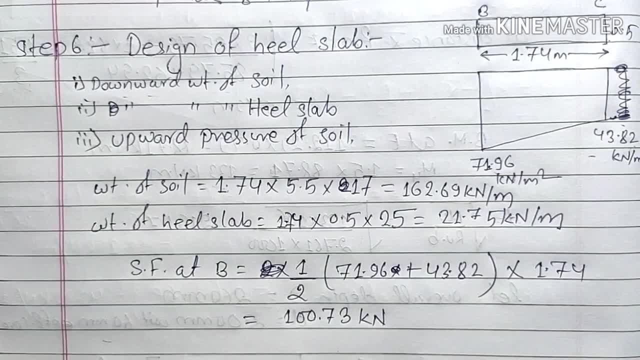 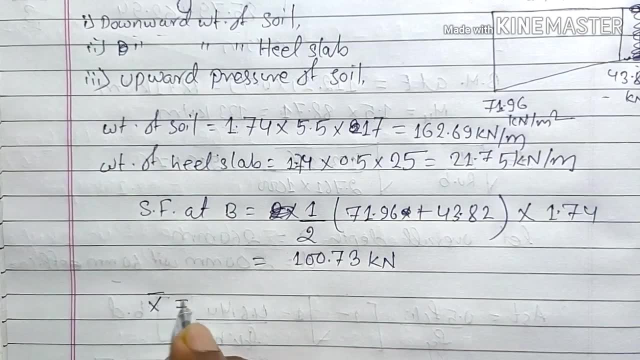 the shear force of B as one hundred point seven, three kilo Newton now this year. seven, three kilo Newton now this year. seven, three kilo Newton now this year. force will be acting at distance: X bar force will be acting at distance, X bar. force will be acting at distance, X bar, which will be given as X bar equals to. 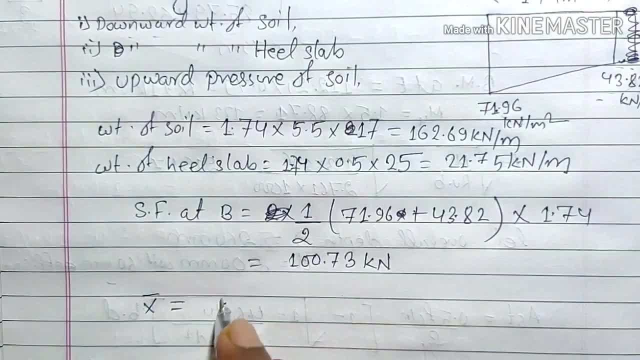 which will be given as X bar equals to, which will be given as X bar equals to: multiply this outer moment by two times. multiply this outer moment by two times. multiply this outer moment by two times, so two times forty three point eight two. so two times forty three point eight two. 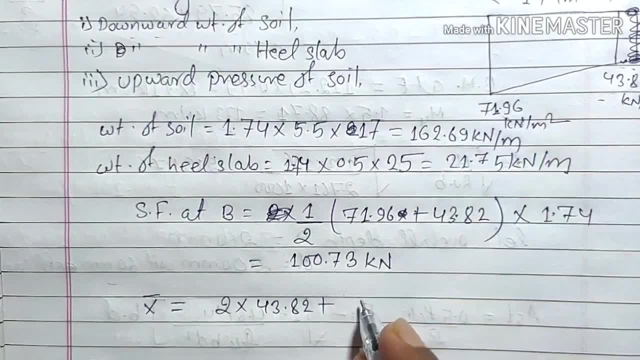 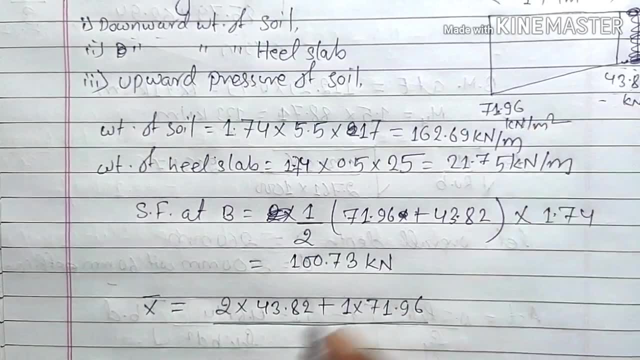 so two times forty three point eight, two plus multiply this inner moment by one. plus multiply this inner moment by one plus multiply this inner moment by one, one time seventy. one point nine, six by one time seventy. one point nine, six by one time seventy one point nine, six by some of the pressure intensities: seventy. 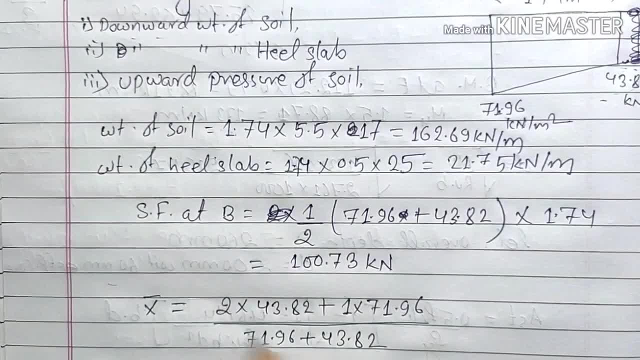 some of the pressure intensities seventy. some of the pressure intensities seventy: one point nine six plus forty three, one point nine six plus forty three, one point nine six plus forty three. point eight: two into span means one point. point eight: two into span means one point. 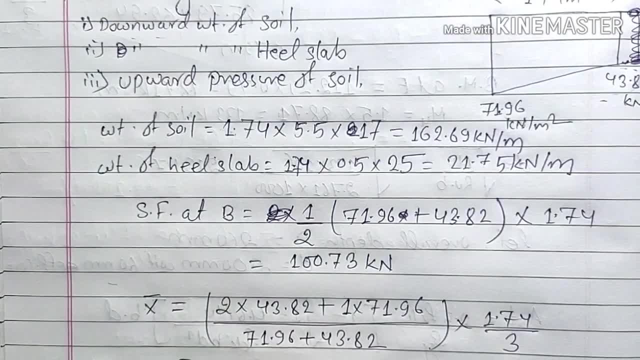 point eight, two into span, means one point seven four divided by three, and we seven four divided by three, and we seven four divided by three, and we would get the value of X bar, which will be. would get the value of X bar which will be: would get the value of X bar, which will be equals to zero point seven nine meter. 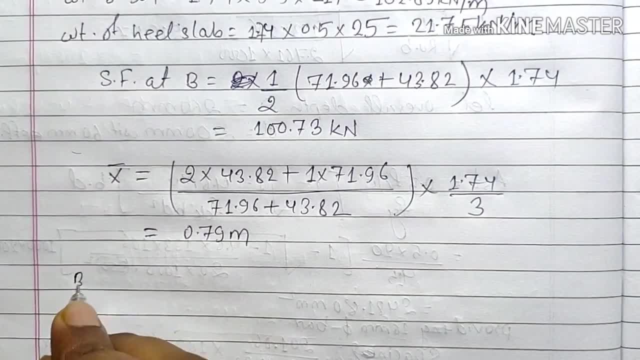 equals to zero point seven nine meter equals to zero point seven nine meter. now, let's find out the bending moment. now, let's find out the bending moment. now. let's find out the bending moment at B and for bending more bending moment at B and for bending more bending moment. 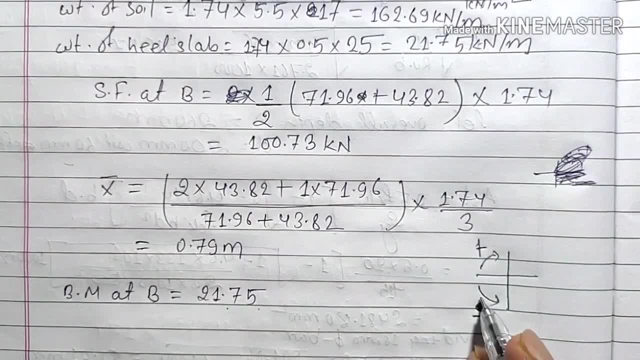 at B and for bending, more bending moment at B. we will take clockwise direction, as at B, we will take clockwise direction as at B. we will take clockwise direction as positive and anti-clockwise direction as positive and anti-clockwise direction as positive and anti-clockwise direction as negative. and here the soil is exerting. 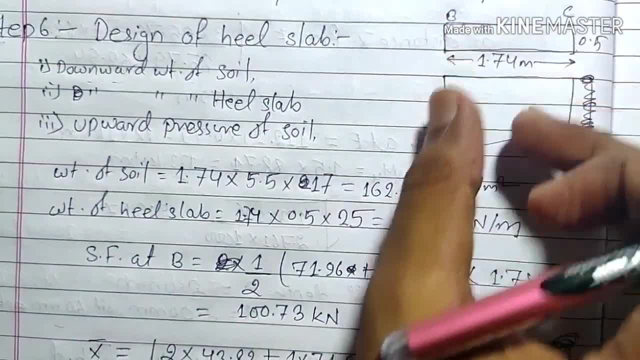 negative. and here the soil is exerting negative. and here the soil is exerting pressure. here the soil is acting up pressure. here the soil is acting up pressure. here the soil is acting up, exerting pressure in upward direction, exerting pressure in upward direction, exerting pressure in upward direction, which will turn the wheels he'll slab in. 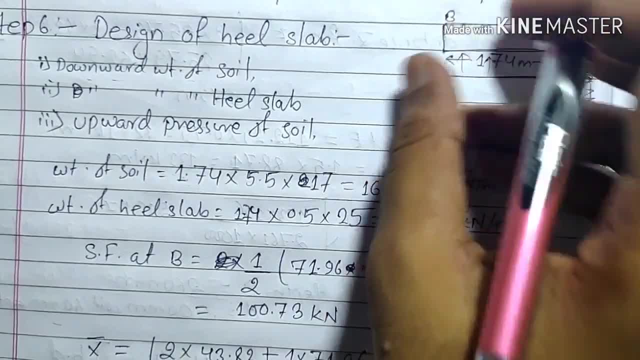 which will turn the wheels. he'll slab in. which will turn the wheels. he'll slab in claw. anti-clockwise direction here like claw. anti-clockwise direction here like claw. anti-clockwise direction here like this. see here it will be rotate in this. see here it will be rotate in. 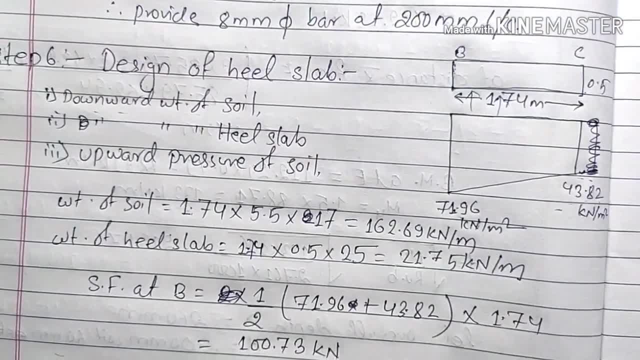 this. see here it will be rotate in: rotated in anti-clockwise direction, so rotated in anti-clockwise direction, so rotated in anti-clockwise direction. so here our anti-clockwise direction will be here our anti-clockwise direction will be here. our anti-clockwise direction will be taken as negative. so write it down here. 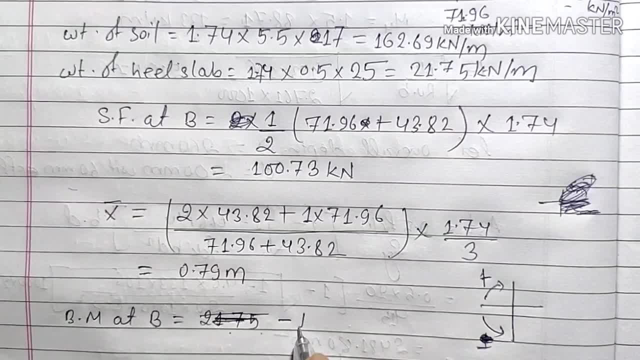 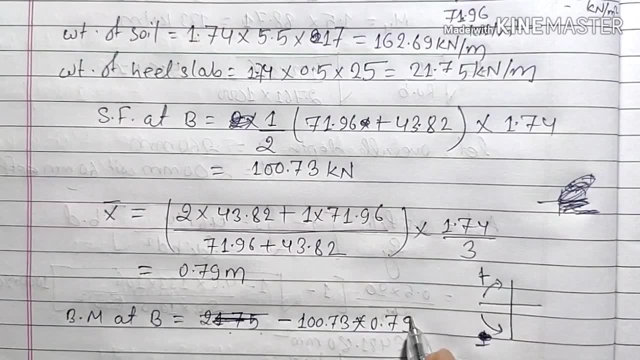 taken as negative, so write it down here. taken as negative, so write it down here: minus one hundred point seven three. into minus one hundred point seven, three. into minus one hundred point seven, three. into zero point seven nine. this is this. zero point seven nine, this is this. 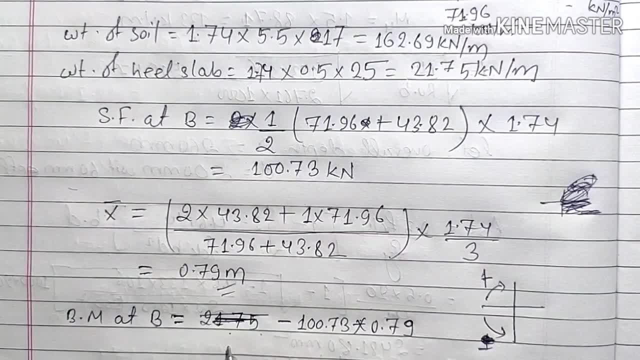 zero point seven, nine. this is this distance of X bar and plus. because the distance of X bar and plus, because the distance of X bar and plus, because the weight of soil is acting in down weight. weight of soil is acting in down weight. weight of soil is acting in down. weight of hill slab is acting in downward. 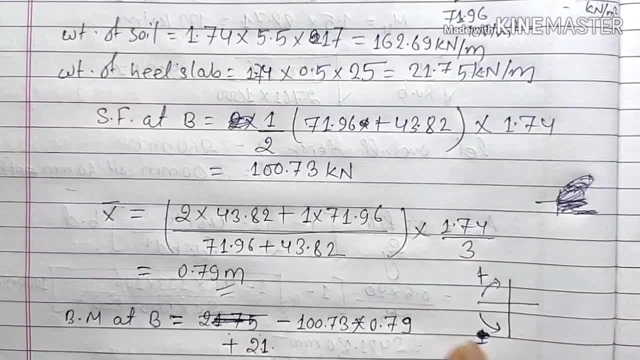 of hill slab is acting in downward, of hill slab is acting in downward direction. downward direction is taking direction. downward direction is taking direction. downward direction is taking clockwise direction. so it will be taken clockwise direction. so it will be taken clockwise direction. so it will be taken as positive. twenty one point seven five. 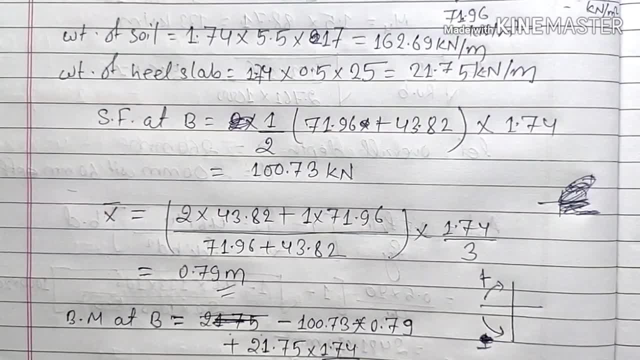 as positive. twenty one point seven, five as positive. twenty one point seven. five into one point, into one point seven, into one point seven, five into one point seven, four divided by two, up to the CG. seven, four divided by two up to the CG. seven, four divided by two up to the CG, and plus one hundred sixty two point. 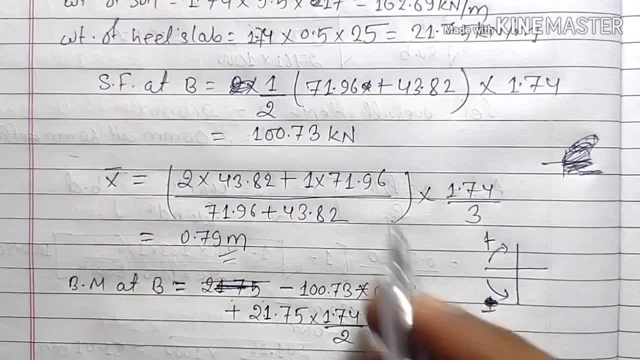 and plus one hundred sixty two point and plus one hundred sixty two point, six nine into which is the weight of soil. six nine into which is the weight of soil. six nine into which is the weight of soil. one hundred sixty two point six nine is one hundred sixty two point six nine is. 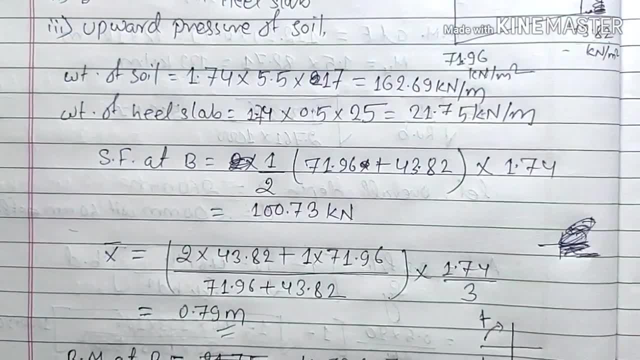 one hundred sixty two point six nine is the weight of soil which is also acting, the weight of soil which is also acting, the weight of soil which is also acting in downward direction. so it will also in downward direction, so it will also in downward direction, so it will also create the clockwise moment, so it will. 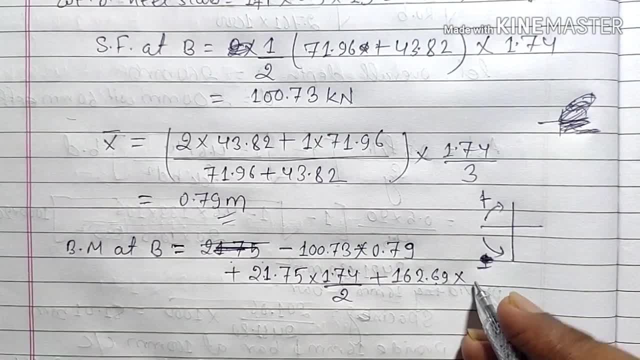 create the clockwise moment. so it will create the clockwise moment, so it will also be again. it will be positive into also be again. it will be positive into also be again. it will be positive into one point seven, four, because the soil. one point seven, four, because the soil. 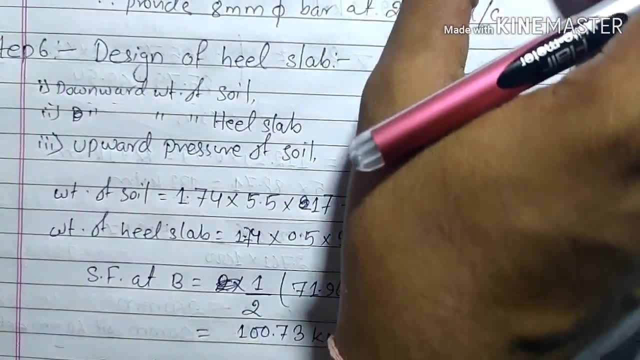 one point seven four, because the soil above the hill slab was taking above the hill slab was taking above the hill slab, was taking rectangular portion and the base was one rectangular portion and the base was one rectangular portion and the base was one point seven four meters, so half of the 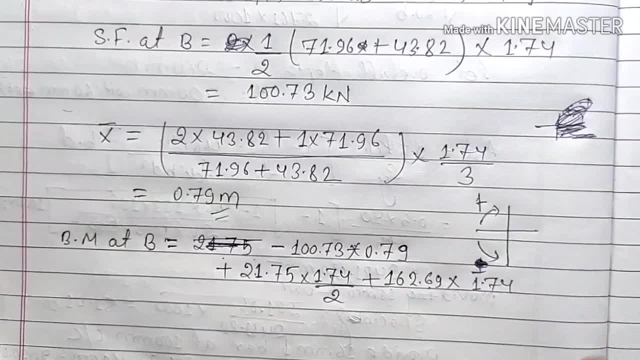 point seven, four meters, so half of the point seven, four meters, so half of the one point seven, four meter. so it will be one point seven, four meter. so it will be one point seven, four meter. so it will be one point seven, four divided meter divided. one point seven, four divided meter divided. 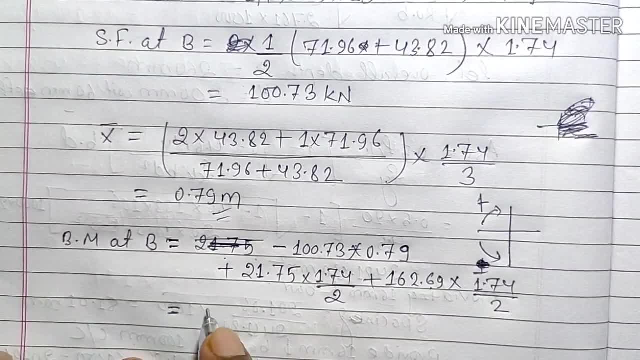 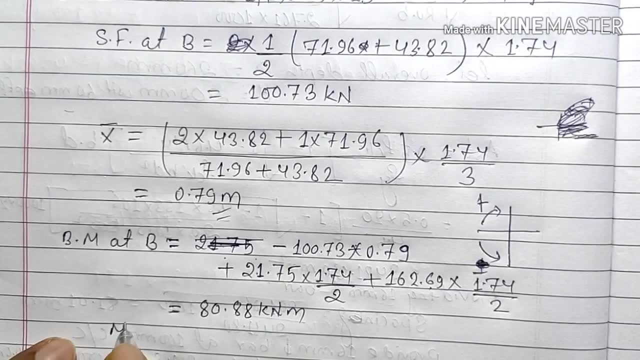 one point seven four meter divided by two, and we will have the bending moment at by two, and we will have the bending moment at by two and we will have the bending moment at B equals to eighty point eight, eight. B equals to eighty point eight, eight. B equals to eighty point eight, eight kilo Newton meter, and we will have MU. 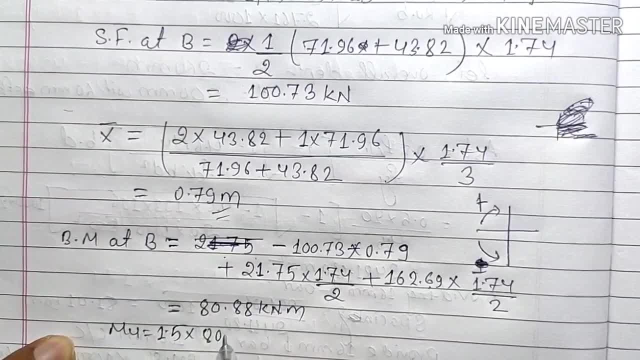 kilo Newton meter and we will have MU kilo Newton meter and we will have MU equals to one point five into eighty. equals to one point five into eighty. equals to one point five into eighty. point eight eight, which will be equals point eight eight, which will be equals. 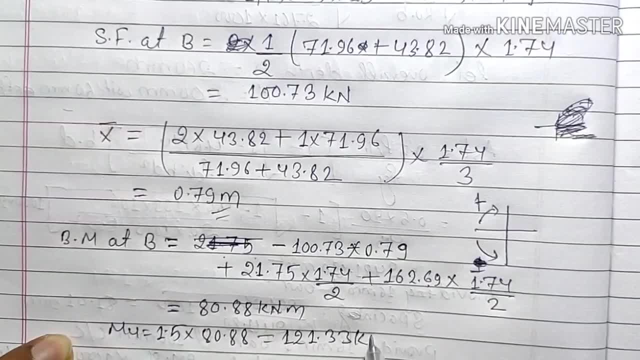 point eight, eight, which will be equals to one hundred twenty one point three to one hundred twenty one point three to one hundred twenty one point three. three kilo Newton meter. now, let's find three kilo Newton meter. now, let's find three kilo Newton meter. now, let's find out the effective depth, effective depth. 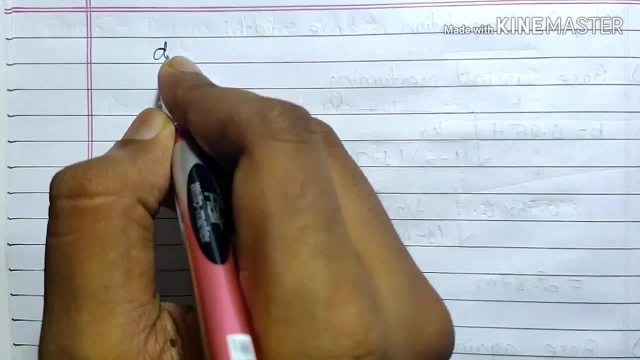 out the effective depth, effective depth, out the effective depth. effective depth of the hill slab, so effective depth of of the hill slab, so effective depth of of the hill slab, so effective. depth of hill slab D will be equals to root under. hill slab D will be equals to root under. 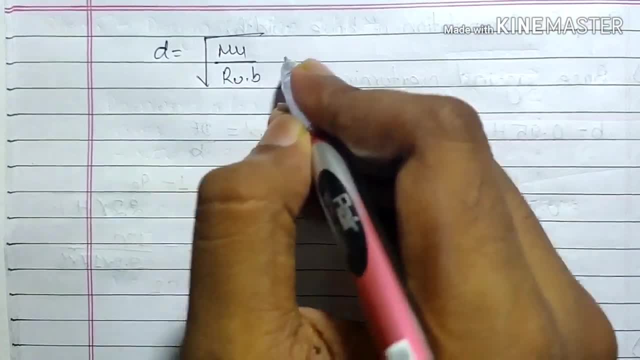 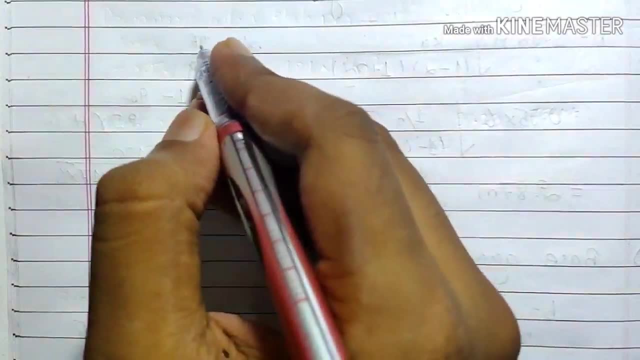 hill, slab D, will be equals to root under MU by R? U times B, which will be equals MU by R? U times B, which will be equals MU by R? U times B, which will be equals to 80 point eight eight, now let's find, to 80 point eight eight, now let's find. 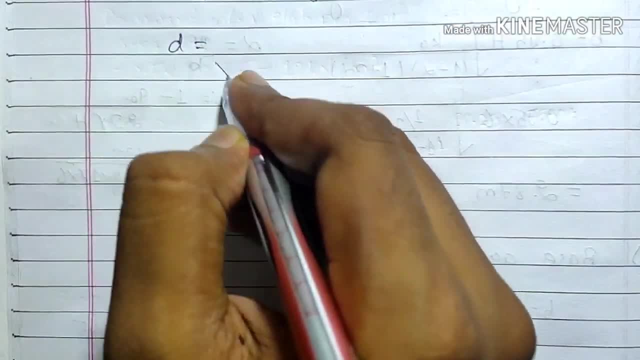 to 80, point eight eight. now let's find out the effective depth of the hill out the effective depth of the hill out, the effective depth of the hill slab. for that we will have a formula D slab. for that we will have a formula D slab. for that we will have a formula D equals to MU by R? U times B, and it will. 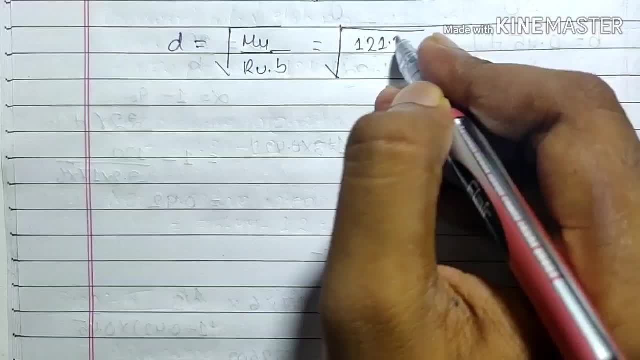 equals to MU by R? U times B, and it will equals to MU by R? U times B, and it will be written as: MU equals to one hundred. be written as MU equals to one hundred. be written as MU equals to one hundred. twenty one point three, three into ten to. 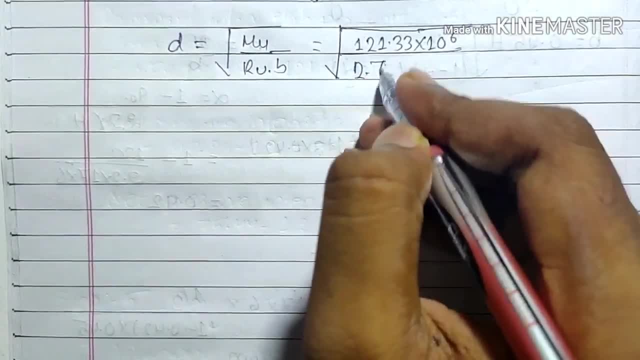 twenty one point three, three into ten to twenty one. point three, three into ten to. the power six: divide by R U means two. the power six, divide by R? U means two. the power six, divide by R? U means two. point seven six, one into thousand and point seven six, one into thousand, and. 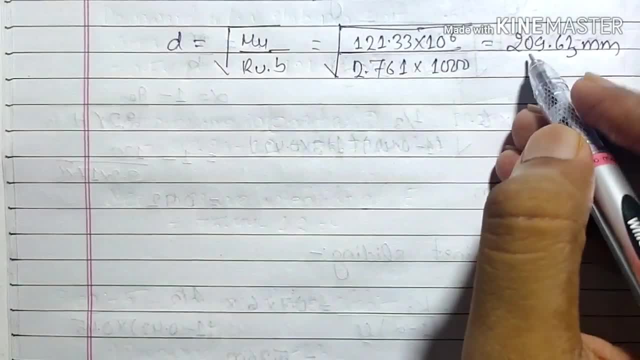 point seven, six, one into thousand, and let's find out the value of D we will. let's find out the value of D we will. let's find out the value of D we will get. is my overall depth equals to two? get? is my overall depth equals to two? 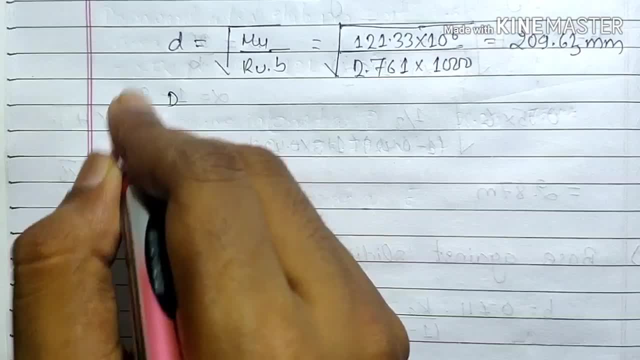 get is my overall depth equals to two hundred nine point six, three kilometer, hundred nine point six, three kilometer, hundred nine point six, three kilometer. so let's take, adopt overall depth equals. so let's take adopt overall depth equals. so let's take adopt overall depth equals to 260 millimeter so that our effective 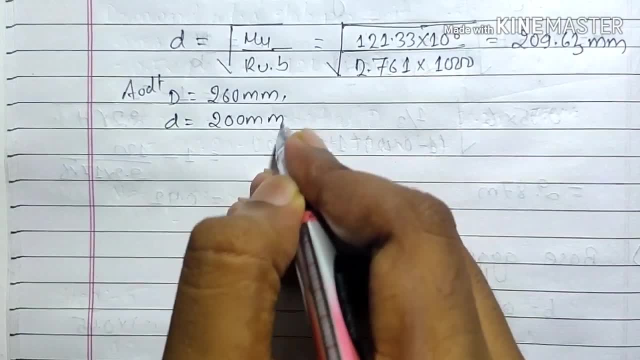 to 260 millimeter, so that our effective to 260 millimeter, so that our effective depth will be equals to 200 millimeter. depth will be equals to 200 millimeter. depth will be equals to 200 millimeter, with no effective cover of 60 millimeter. 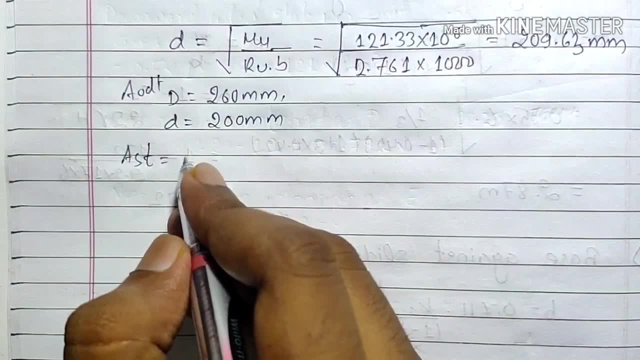 with no effective cover of 60 millimeter. with no effective cover of 60 millimeter. now let's find AST and use the formula. now let's find AST and use the formula. now let's find AST and use the formula for finding AST: 0.5 F, C, K by F Y times 1. 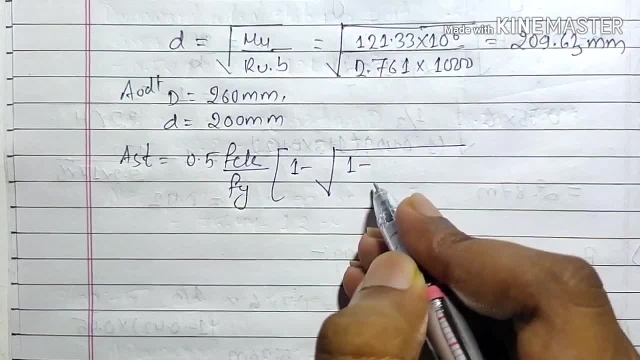 for finding AST 0.5 F C K by F Y times 1. for finding AST 0.5 F C K by F Y times 1 minus root under 1 minus 4.6 mu by F C. minus root under 1 minus 4.6 mu by F C. 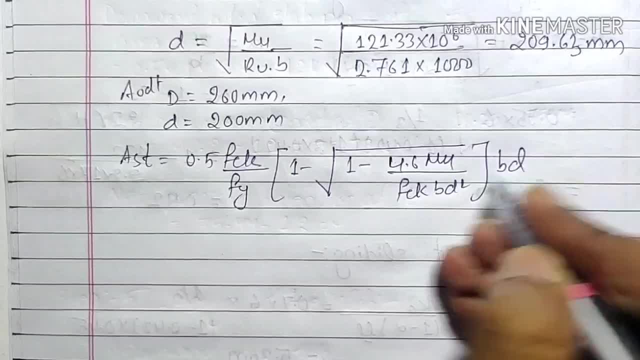 minus root, under 1 minus 4.6 mu by F C, K B D square times B D, put the value and K B D square times B- D. put the value and K B D square times B D, put the value and find AST. so we have got the value of. find AST. so we have got the value of find AST. so we have got the value of AST as: 2, 1, 6, 9 point 3, 2 millimeter. AST as 2, 1, 6, 9 point 3, 2 millimeter. 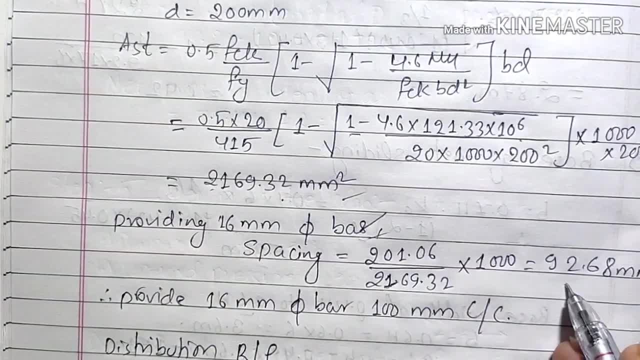 AST as: 2, 1, 6, 9, point 3: 2 millimeter square. we have provided 16 millimeter square. we have provided 16 millimeter square. we have provided 16 millimeter dia bar and calculated the spacing and I dia bar and calculated the spacing and I. 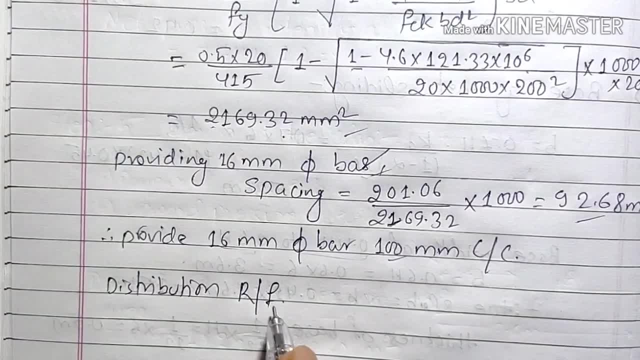 dia bar and calculated the spacing and I have provided 16 millimeter dia bar at. have provided 16 millimeter dia bar at. have provided 16 millimeter dia bar at 100 millimeter Center to Center now. 100 millimeter Center to Center now. 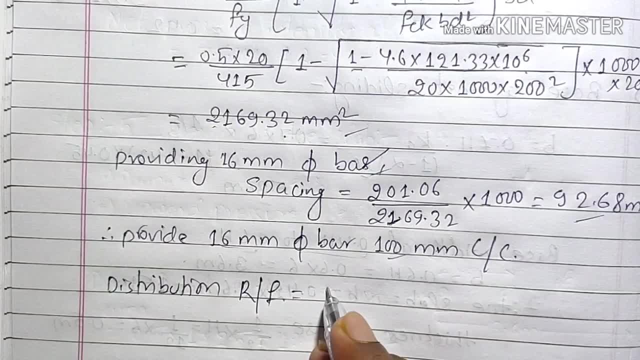 100 millimeter Center to Center. now let's find out distribution reinforcement. let's find out distribution reinforcement. let's find out distribution reinforcement taking 12% of the overall diameter. so taking 12% of the overall diameter. so taking 12% of the overall diameter, so overall area, gross area, which is actually 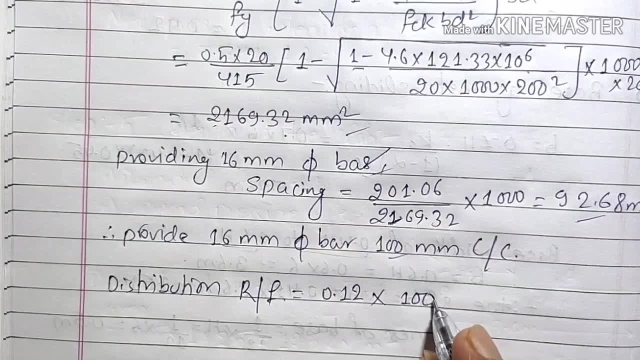 overall area, gross area, which is actually overall area, gross area, which is actually gross area. so it will be equals to 1000 gross area. so it will be equals to 1000 gross area. so it will be equals to 1000 into 200 divided by 100, and we will get 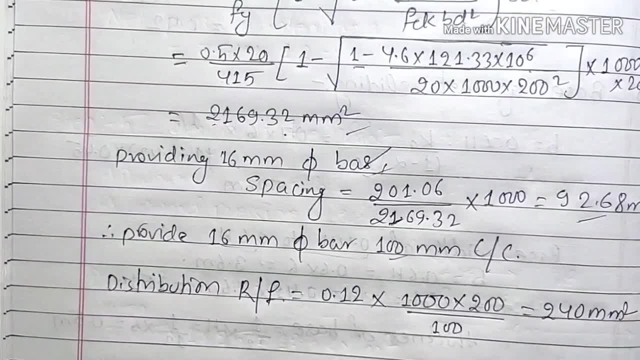 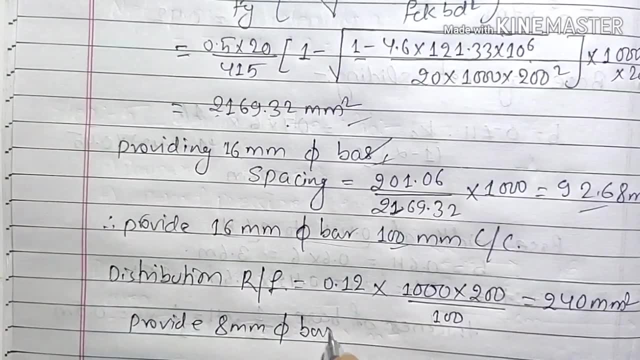 into 200 divided by 100, and we will get into 200 divided by 100 and we will get it as 240 millimeter square and provide it as 240 millimeter square and provide it as 240 millimeter square and provide 8 millimeter, 8 millimeter dia bar and we 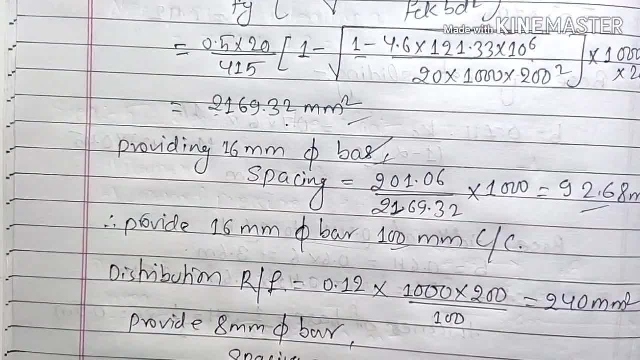 8 millimeter, 8 millimeter dia bar and we 8 millimeter, 8 millimeter dia bar and we will get spacing equals to area of 1, will get spacing equals to area of 1, will get spacing equals to area of 1 bar divided by AST into thousand. 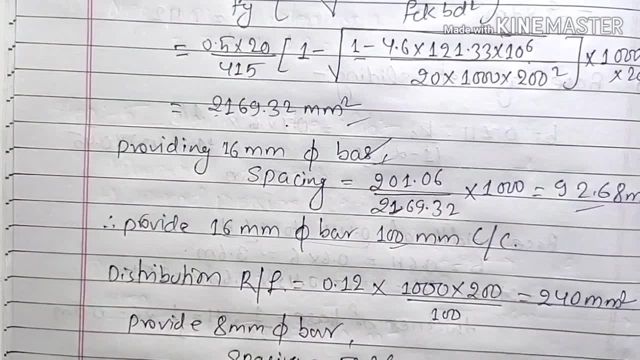 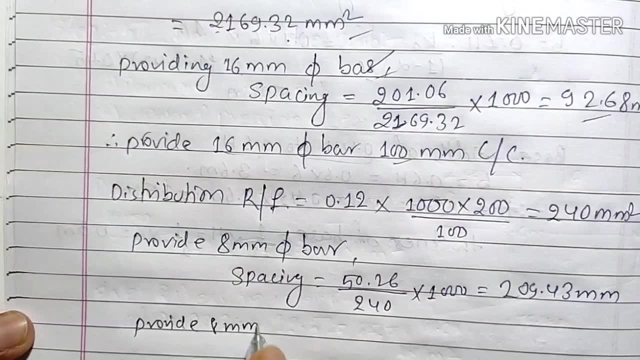 bar divided by AST into thousand. bar divided by AST into thousand, and it will be equals to 209 point for, and it will be equals to 209 point for, and it will be equals to 209 point for 3 millimeter. so provide 8 millimeter dia. 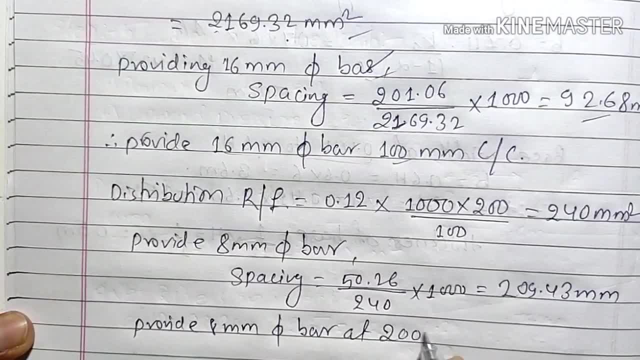 3 millimeter, so provide 8 millimeter dia. 3 millimeter, so provide 8 millimeter dia. bar at 200 millimeter Center to Center. bar at 200 millimeter Center to Center. bar at 200 millimeter Center to Center. now it's time for the design of. 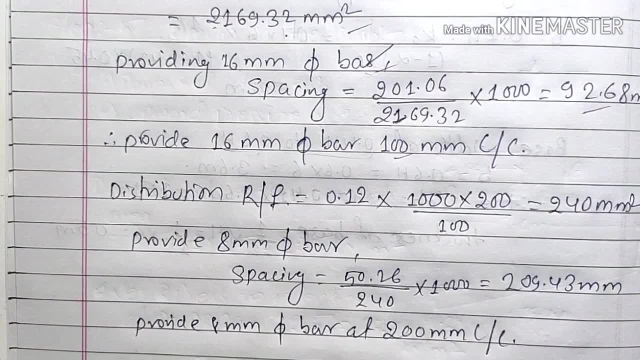 now it's time for the design of. now it's time for the design of reinforcement of the steam slab. let's, reinforcement of the steam slab, let's reinforcement of the steam slab, let's, now, let's go for it. so, here in step 7, we now, let's go for it. so here in step 7, we. 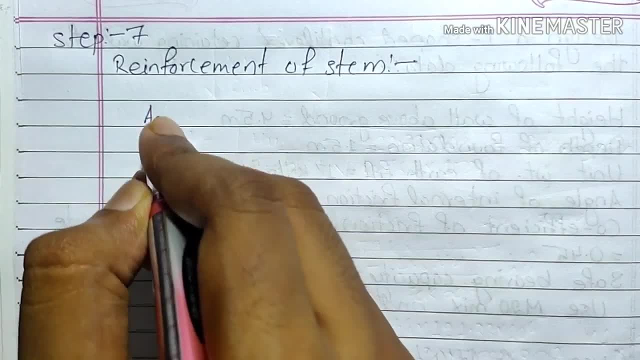 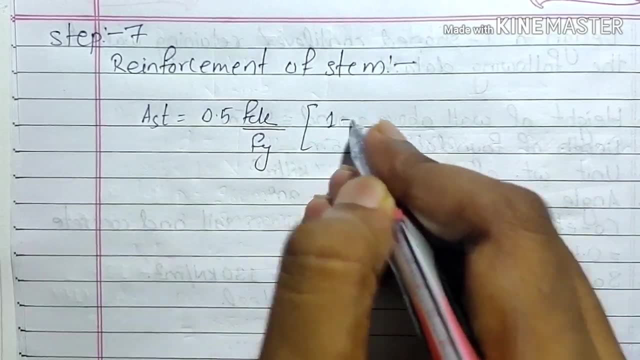 now, let's go for it. so here, in step 7, we will design the reinforcement of his will, design the reinforcement of his will, design the reinforcement of his team, and we have AST equals to zero team, and we have AST equals to zero team, and we have AST equals to zero. point 5, fck by FY times 1 minus root. 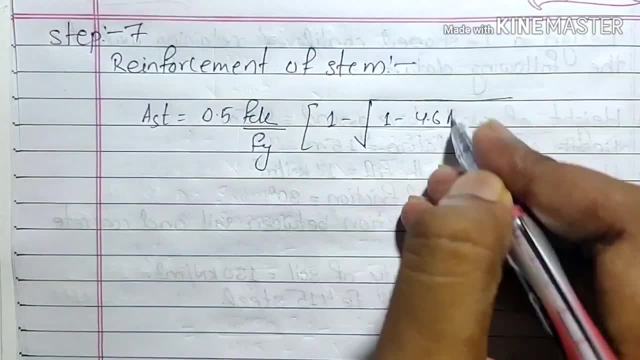 point 5: fck by FY times 1 minus root. point 5: fck by FY times 1 minus root. under 1 minus 4.6 mu by fck BD square. under 1 minus 4.6 mu by fck BD square. 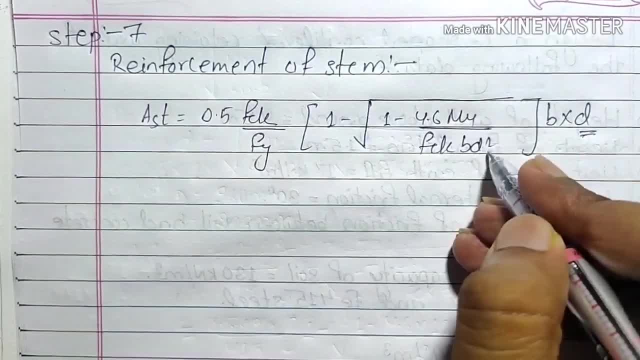 under 1 minus 4.6 mu by fck BD square times B into D, and we have already times B into D, and we have already times B into D and we have already calculated the value of a small D, so put. calculated the value of a small D, so put. 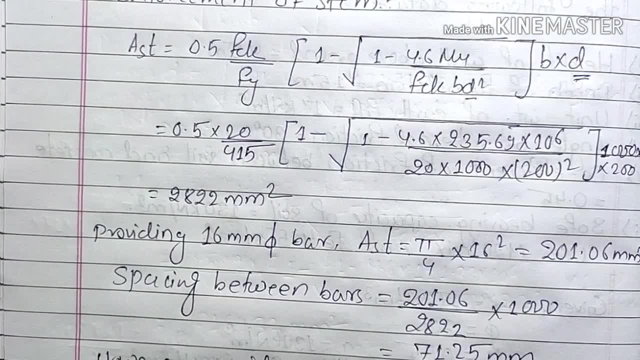 calculated the value of a small D. so put the value and find out the AST. so the the value and find out the AST. so the the value and find out the AST. so the step is similar for the reinforcement of step is similar for the reinforcement of step is similar for the reinforcement of esteem, which is we have calculated AST. 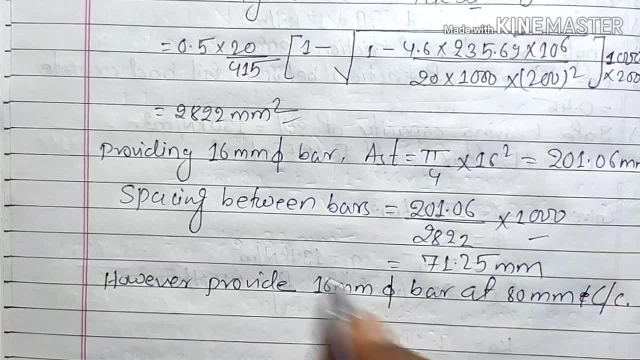 esteem, which is we have calculated AST esteem, which is, we have calculated AST, and then we have calculated the spacing, and then we have calculated the spacing, and then we have calculated the spacing between the bar by providing 16 minute between the bar, by providing 16 minute. 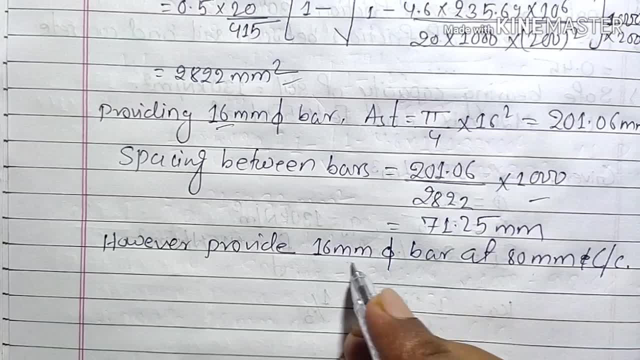 between the bar by providing 16 minute a dia bar, and hence we have provided 16 a dia bar, and hence we have provided 16 a dia bar, and hence we have provided 16 meter dia bar at 80 centimeter center to meter dia bar at 80 centimeter center to. 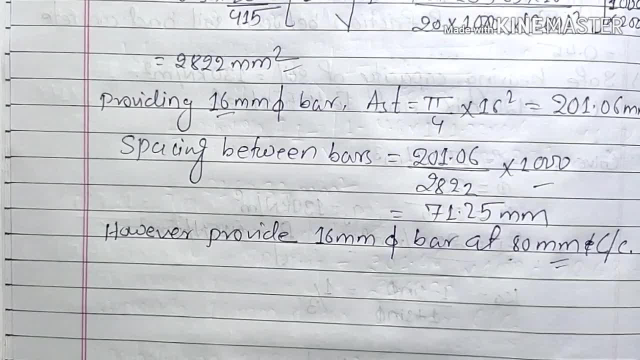 meter dia bar at 80 centimeter center to center. now let's move to our the final center. now let's move to our the final center. now let's move to our the final step, which is the design of CR key step, which is the design of CR key. 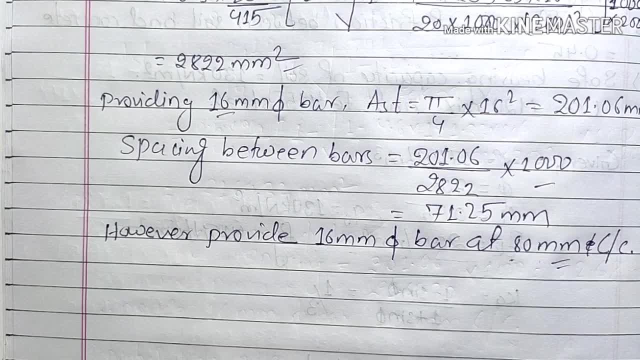 step, which is the design of CR key. because we are providing the CR key, because we are providing the CR key because after, because our retaining wall, because after, because our retaining wall, because after, because our retaining wall was fading in sliding, if it were, if our was fading in sliding, if it were, if our 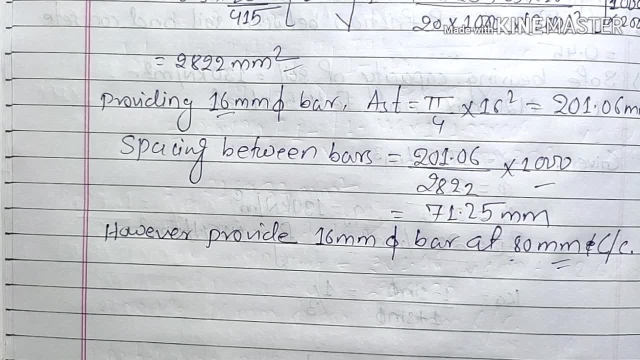 was fading in, sliding, if it were, if our value- a factor of safety- would have come, value, a factor of safety would have come value, a factor of safety would have come greater than 1.5, then there you would. greater than 1.5, then there you would. 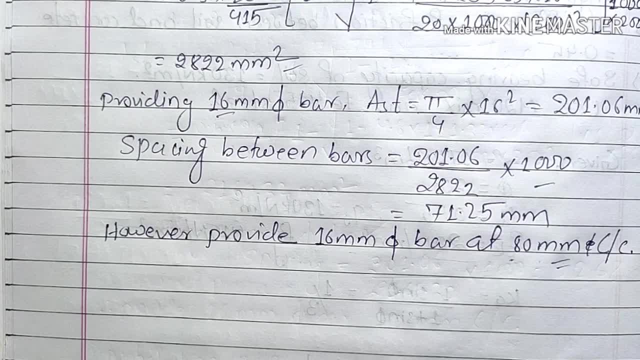 greater than 1.5, then there you would have no need to do the design of CR key, have no need to do the design of CR key, have no need to do the design of CR key as our value was less than 1.5. so we 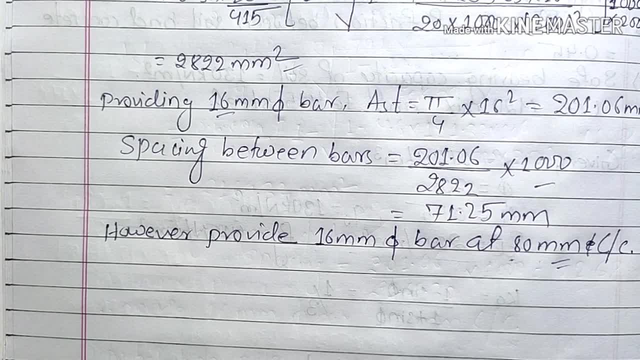 as our value was less than 1.5. so we, as our value was less than 1.5, so we need to design the CR key. let's go for need to design the CR key. let's go for need to design the CR key. let's go for it now and for the design of CR key. it. 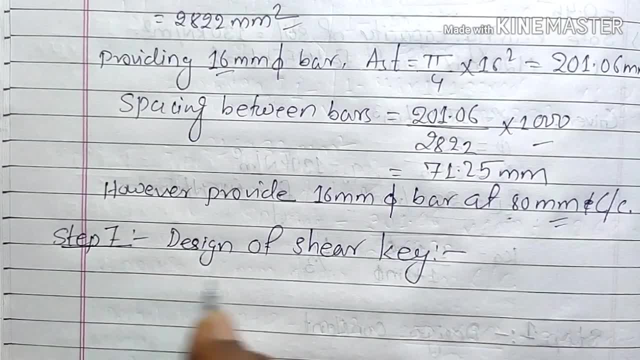 it now and for the design of CR key. it it now and for the design of CR key. it is up to us how much dimension we were. we is up to us how much dimension we were. we is up to us how much dimension we were we want to take. so let's take size of CR. 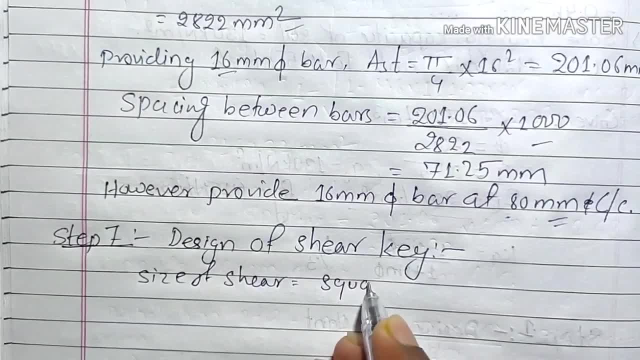 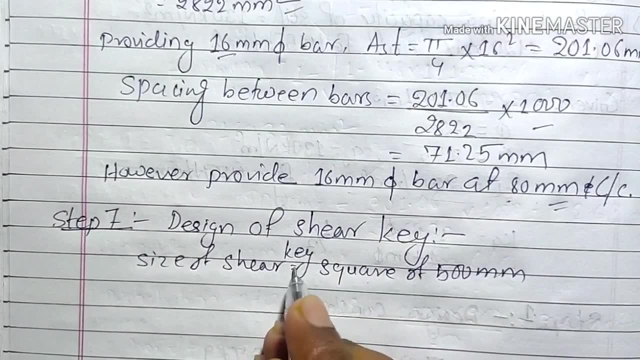 want to take, so let's take size of CR. want to take, so let's take size of CR. key equals to square of 500 millimeter. key equals to square of 500 millimeter. key equals to square of 500 millimeter. it's the CR. key. should be slightly more.